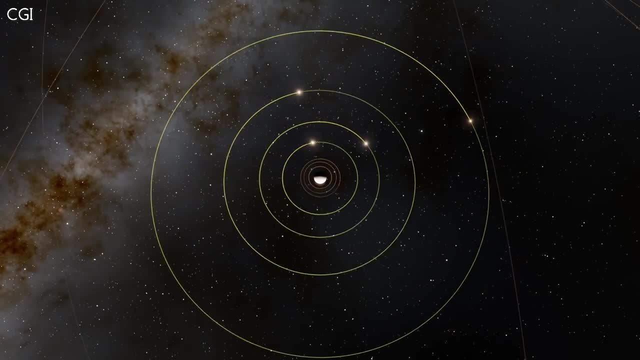 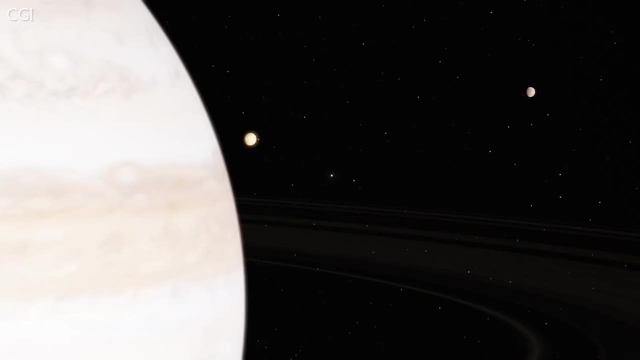 Ganymede and Callisto. Beyond them are the irregular moons of Jupiter, all of which are much further out than the previous moons. Io orbits very close to Jupiter, only 350,000 kilometres above Jupiter's cloud tops. This means from Io's surface, Jupiter would appear thirty-nine times bigger. 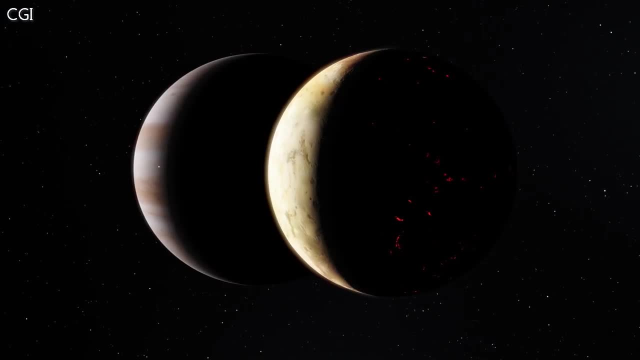 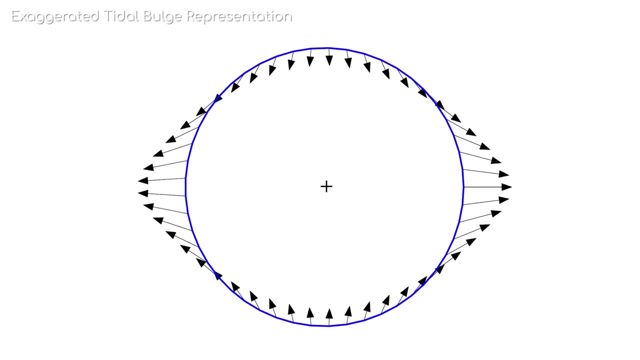 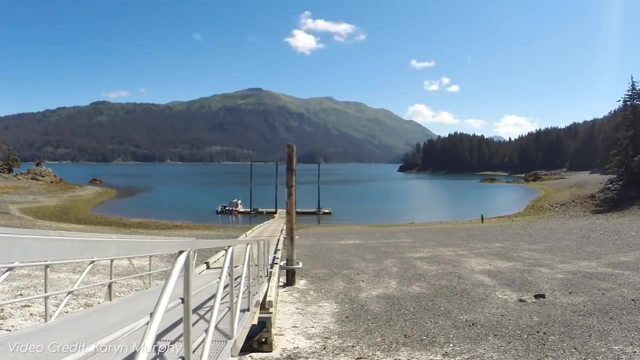 in the sky than our moon. Io orbits Jupiter in only 42.5 hours, compared to our moon's monthly orbit. At some points in its orbit, the tidal bulge on Io is thought to be up to 100 metres. This effect is similar to what we see on Earth, with the ocean's tides being 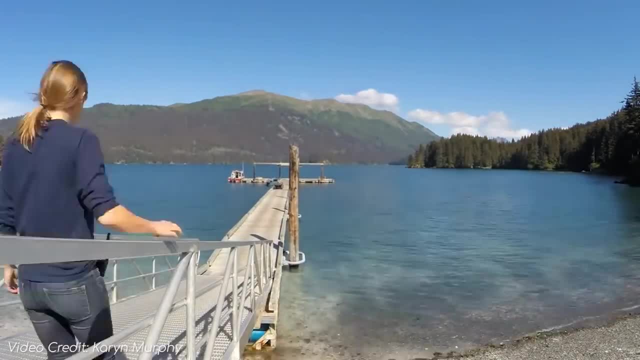 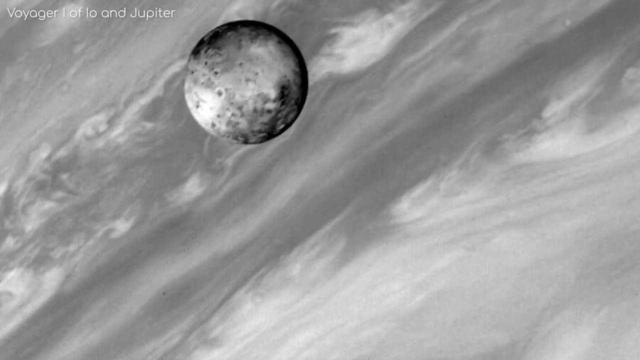 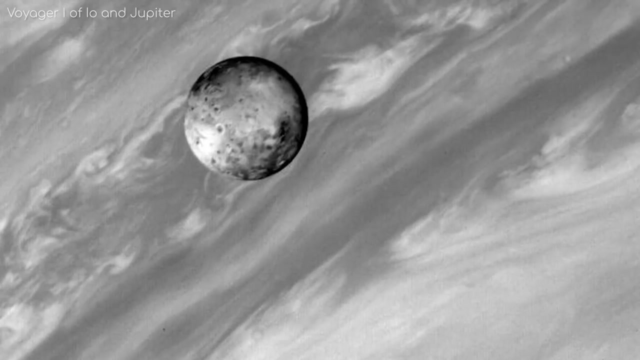 caused by the moon, although on Earth the effect is much more minimal, the tides only usually shifting about 2 metres from high to low. Io is getting 300% more tidal force exerted on it in comparison to our moon on us because of its close proximity to the biggest. 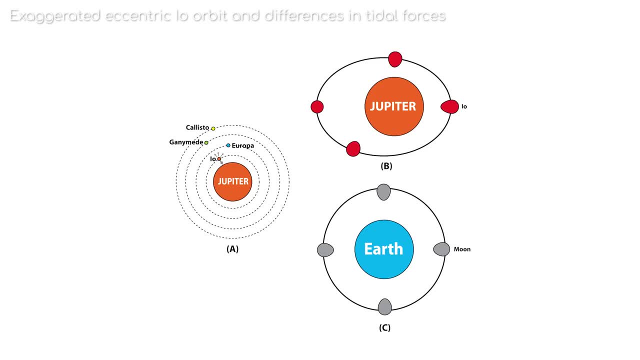 planet in the solar system, Jupiter and the other big moons in the system don't allow the moon's orbit to be any less eccentric, meaning Io isn't going to be getting any respite any time soon. A day on Io is the same as its orbital rotation, which means 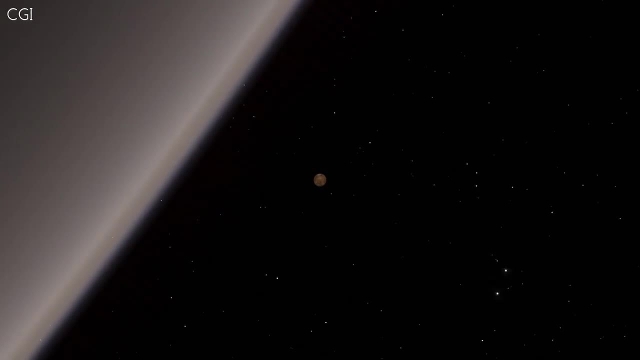 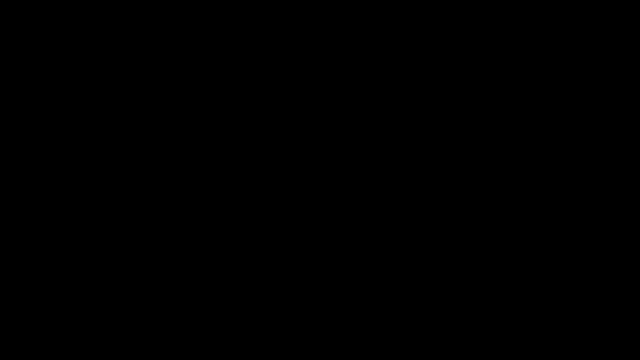 that Io is not going to be getting any respite any time soon. Io is tidally locked to Jupiter. just like we can only see one face of our moon from Earth, only one face of Io can ever be seen from Jupiter. Io is a pretty big moon, although. 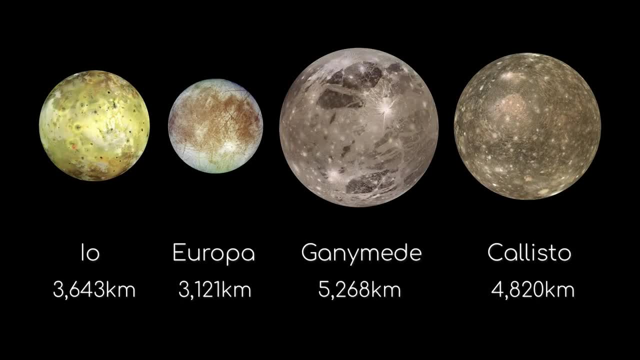 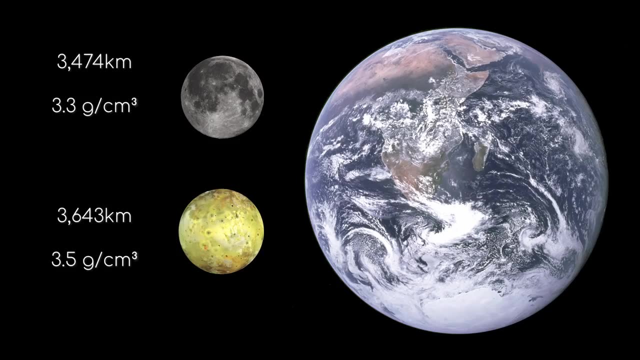 it is the second smallest out of the Galilean moons. It is comparable in size to Earth's moon and shares a similar density, meaning it has a similar amount of gravity, but interestingly it does have the highest density of any other moon in the solar system. 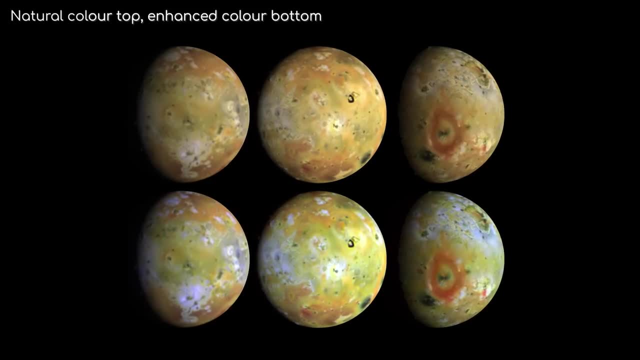 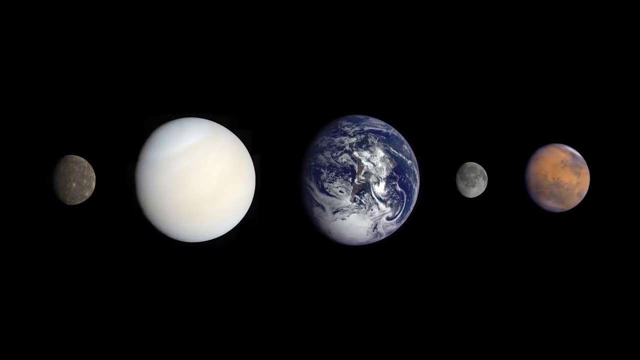 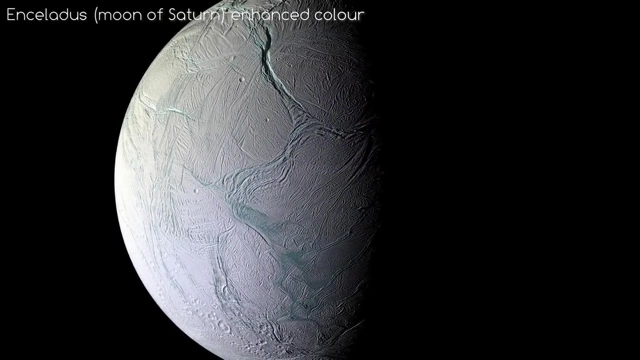 teaspoon. Io is a little over 2.7 famoso. It bears almost 7 million tons of uranium per trillion inspiration, on the top of which are around 2 million stars. The ordinary light� cites a very average solar constellation that is probably about 3 times as large in the solar system as the. 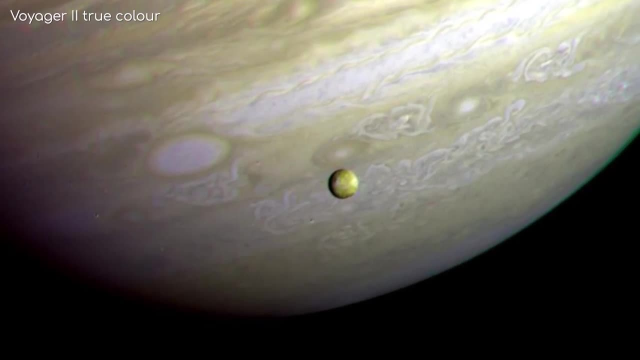 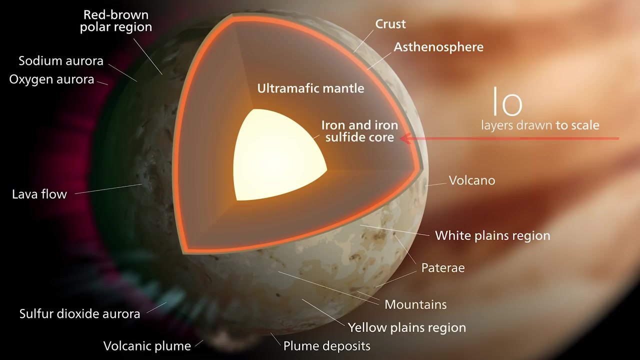 one in Io, in Pluto. It is quite unique, given how few such celestial beings having ever ever been found in the solar system: tom tom, eggplant or silicate-rich mantle and crust. The core is not thought to be convecting, though, as no. 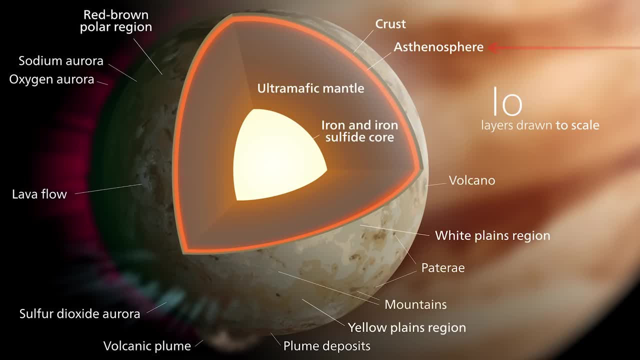 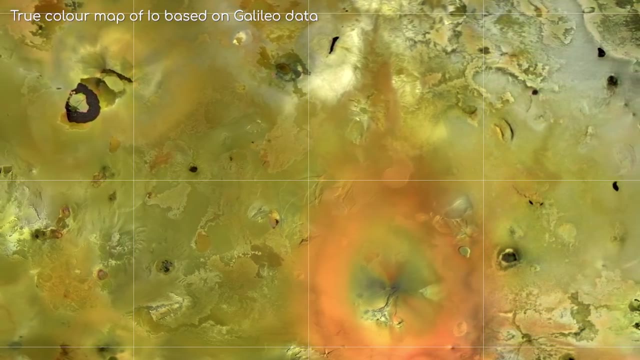 magnetosphere has been detected around the moon. The mantle is thought to be liquid near the crust and is at least 50km thick. This is where all the volcanism originates, Which brings us to perhaps the most interesting part about Io: the hundreds of huge volcanoes. 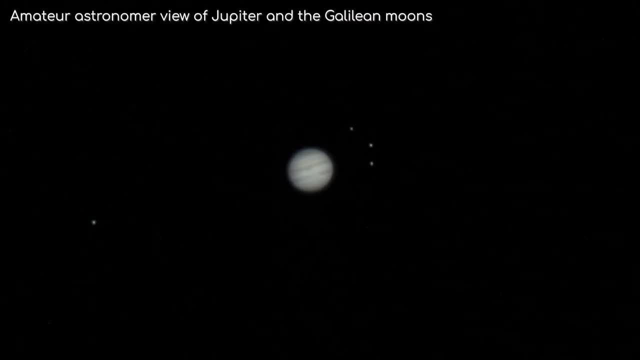 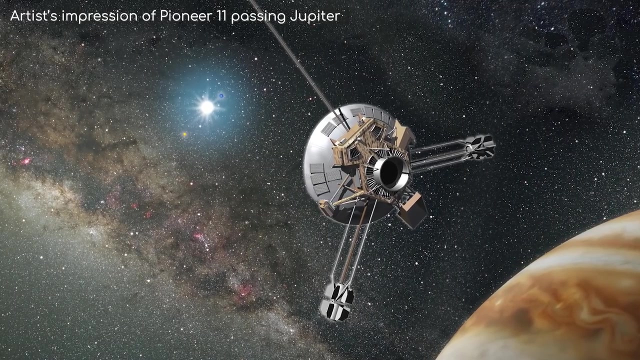 all over its surface. Before the 1970s, we didn't know much about Io at all, although telescopes were starting to pick up hints that the moon was devoid of water and that it may have a surface of sulphur. The first mission to see Io in any kind of detail was 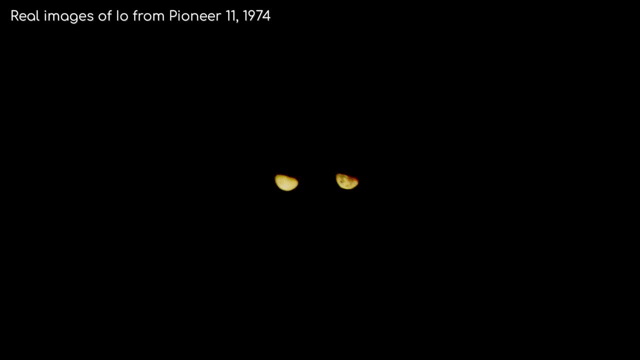 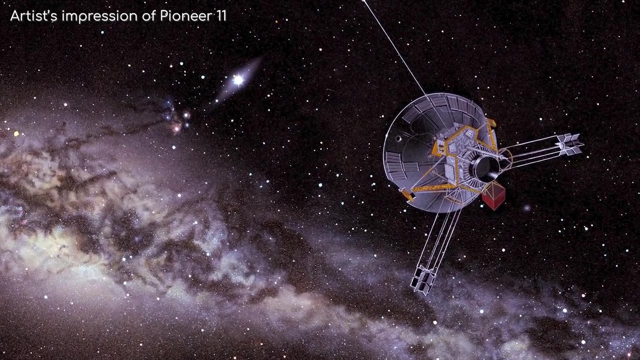 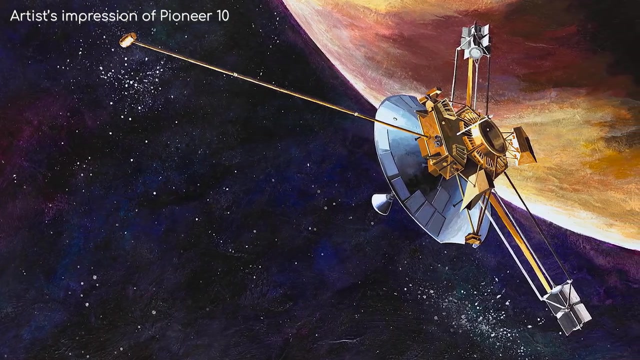 Pioneer 11,, although the quality was still not great. What it did detect, however, is that Io was made of silicate rock and not water ice, and that it has a thin atmosphere. Pioneer 10 was also meant to take some closeup. 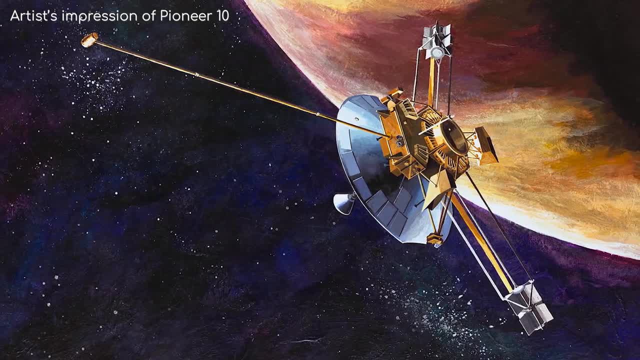 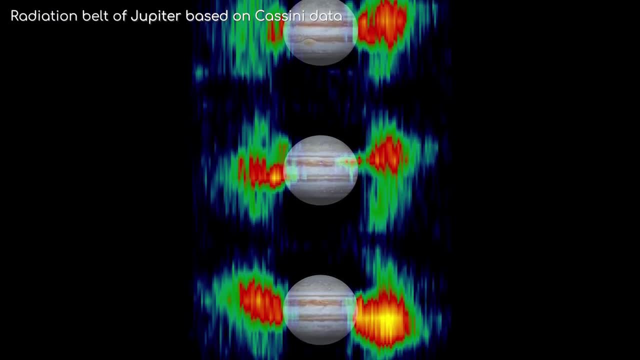 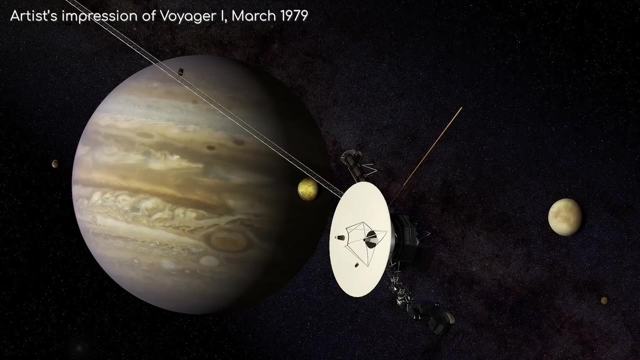 shots of Io, but this was lost due to Jupiter's radiation interfering with the on-board command system. The radiation Pioneer 10 went through was 10,000 times stronger than the maximum radiation around the Earth. The next missions to Jupiter were the Voyager. 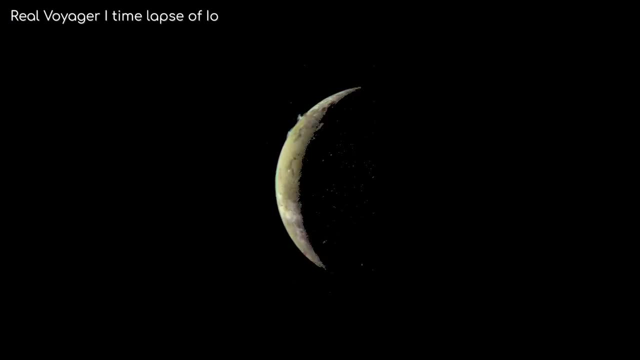 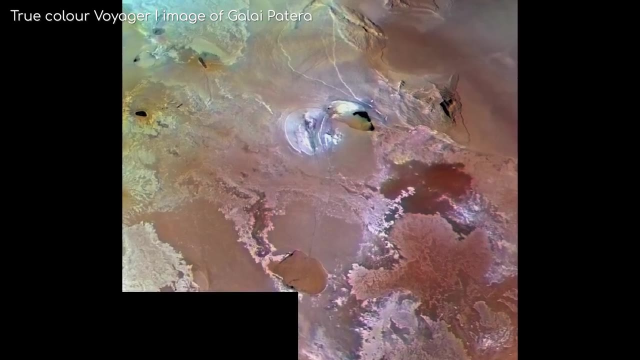 1 and 2 missions in 1979.. Voyager 1 flew by at a distance of only 20,000 kilometres and was able to take some impressive close-ups of Io's surface. What it saw was a remarkable landscape full of vibrant colours and a total absence of 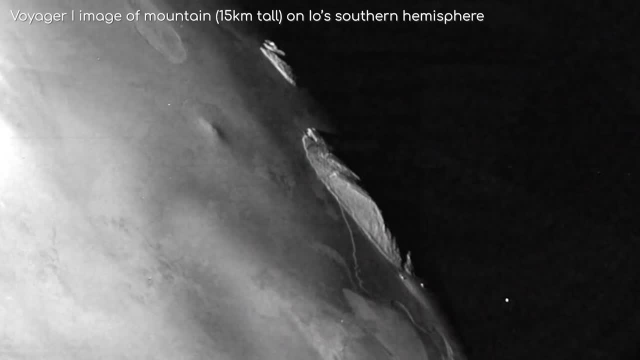 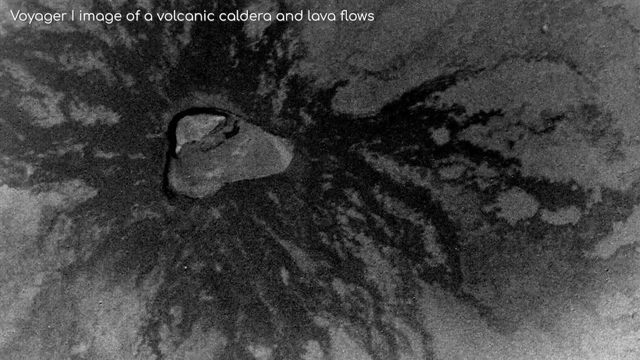 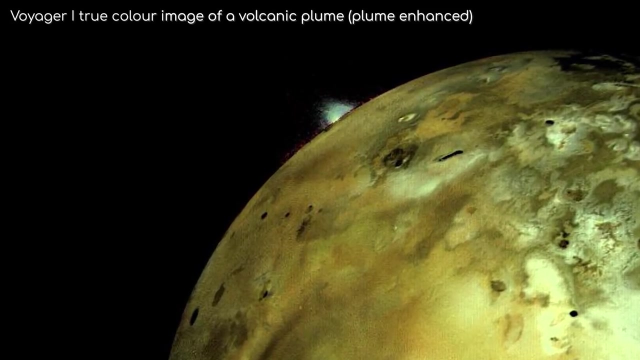 impact craters. It found mountains taller than Everest, as well as volcanic pits hundreds of kilometres wide and what looked to be lava flows. Most notably, however, was the presence of plumes coming from the surface. This proved that Io is volcanically active. 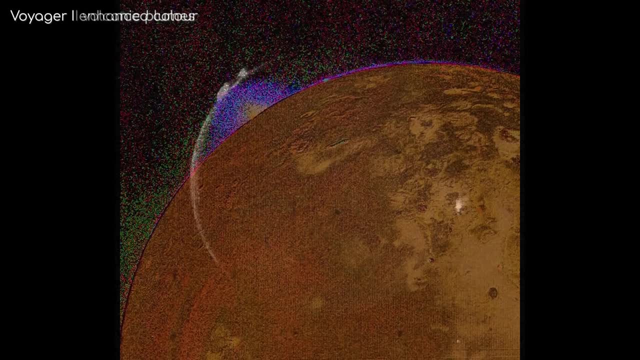 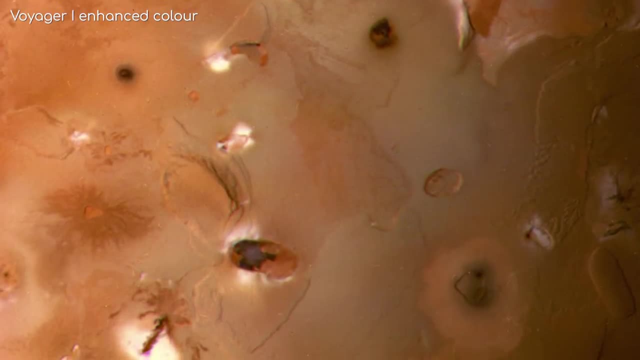 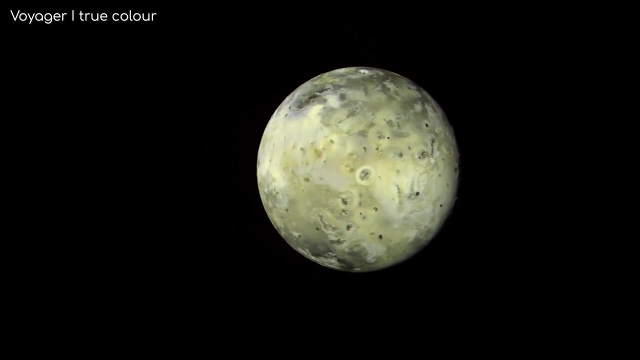 and it is still the first and only place this has been visibly seen beyond Earth, not including cryovolcanoes. Voyager 1 also confirmed that the surface of Io is covered in different sulphur frosts. This is what gives Io its many spectacular colours. It found that it 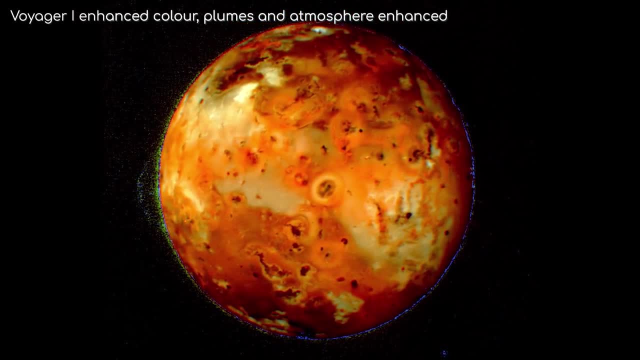 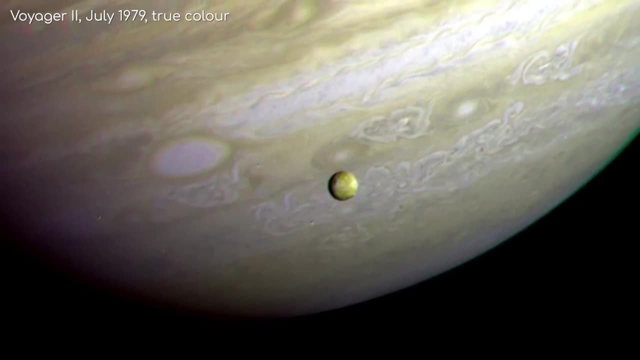 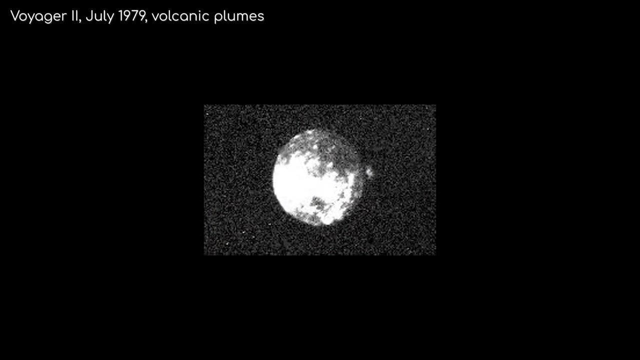 is these sulphur compounds that dominate the atmosphere. 3.. Voyager 2 also saw Io in July of 1979, but was much further away, at 1 million kilometres, although it still saw seven of the nine plumes Voyager 1 saw in March, which meant those: 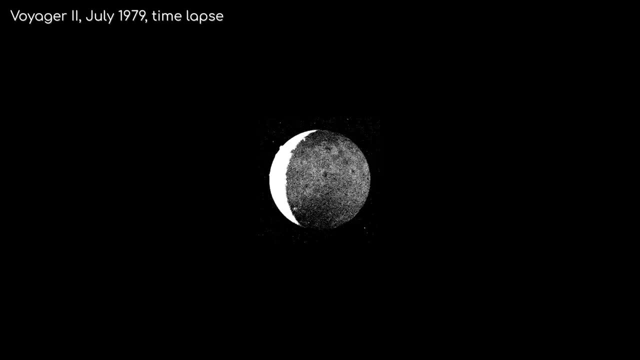 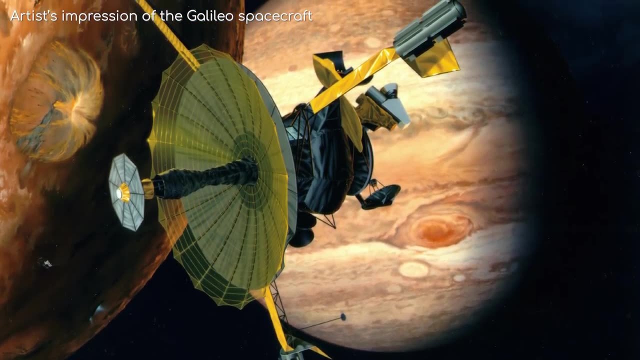 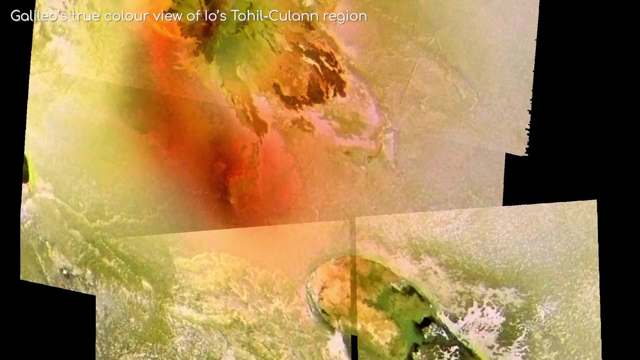 volcanoes had likely remained active throughout those four months. The really interesting images came about with the Galileo spacecraft that arrived at Jupiter in 1995.. The spacecraft wasn't especially designed to study Io, but it was able to acquire some of the highest 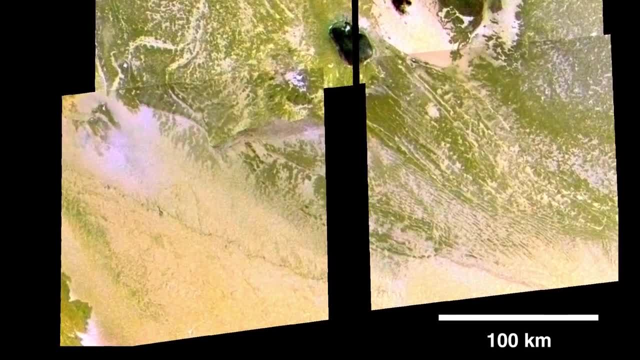 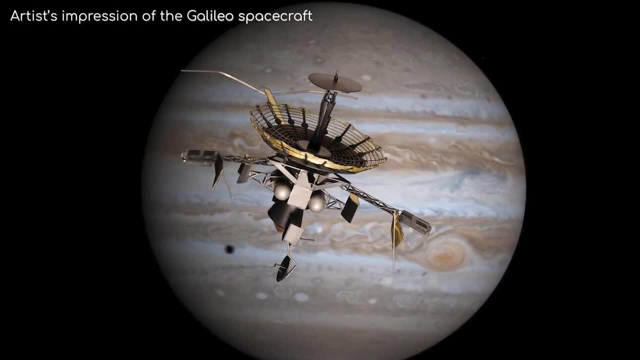 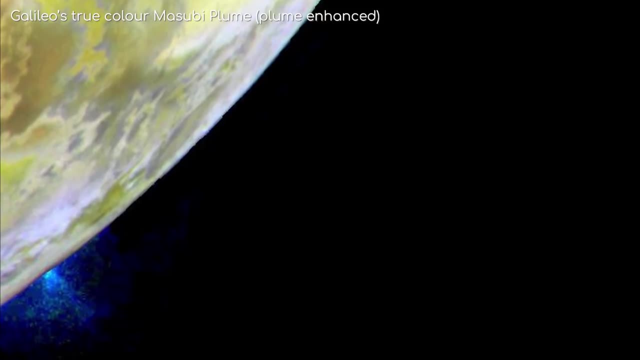 resolution images we now have of its surface. Sadly, though, Galileo never worked at full capacity, as it had quite a few mechanical malfunctions, which means we could have had even better images had it been fully operational. What it was able to see, though, were plumes. 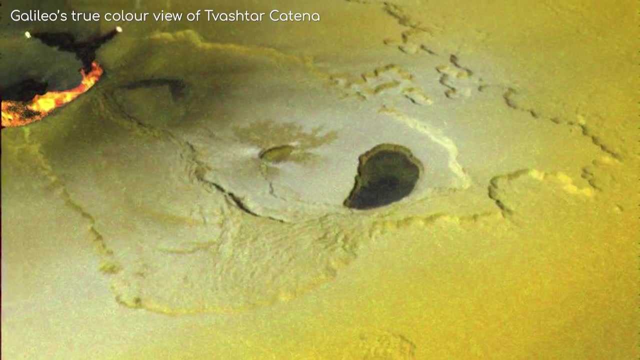 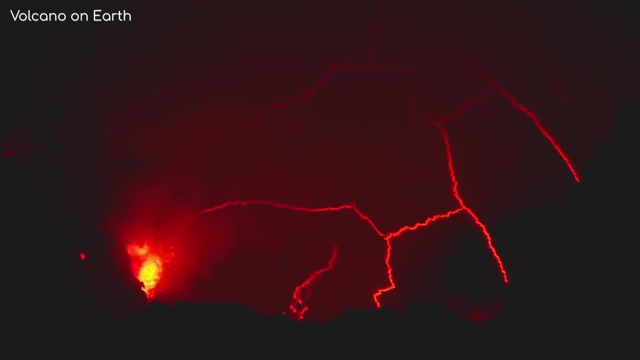 from many volcanoes. 4. Volcanoes in Io. In the early 20th century, the Volcanoes of Io were known to have erupted in sulphur and silicate magmas similar to what we have on Earth. except the magma on Io is also rich. 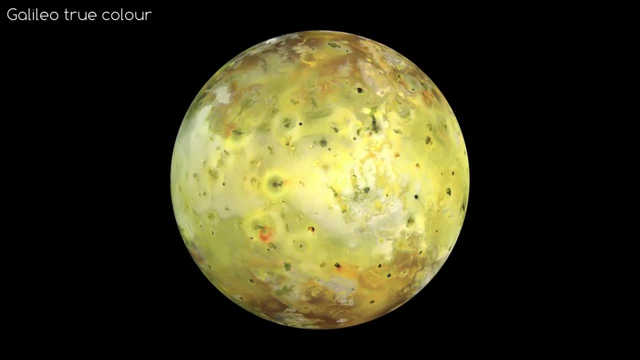 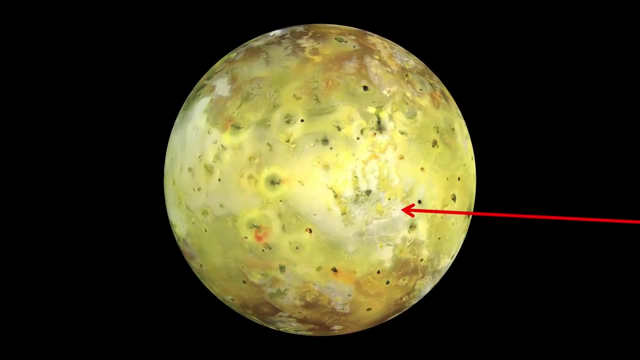 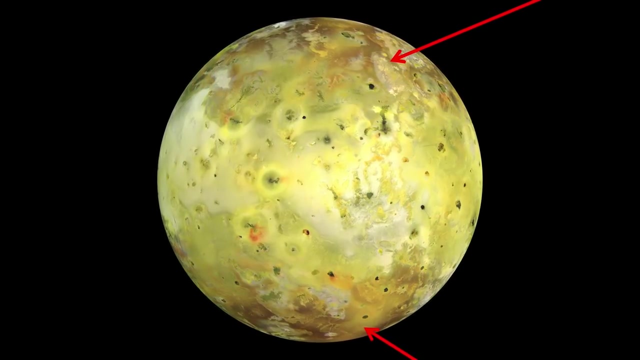 in magnesium. The surface of Io is spectacularly colourful. The yellow plains are composed of mainly sulphur. the white areas are mainly fresh sulphur dioxide frosts Towards the poles. the sulphur is damaged by radiation, which can be seen as the poles appear to be. 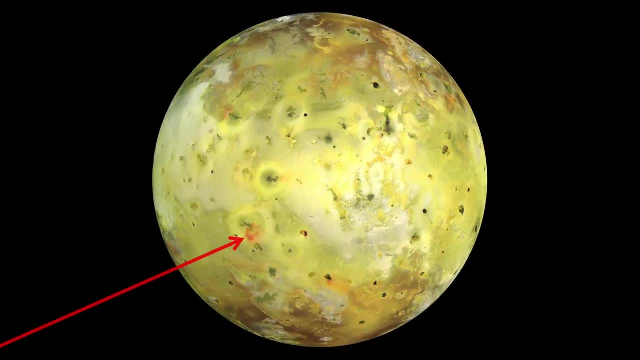 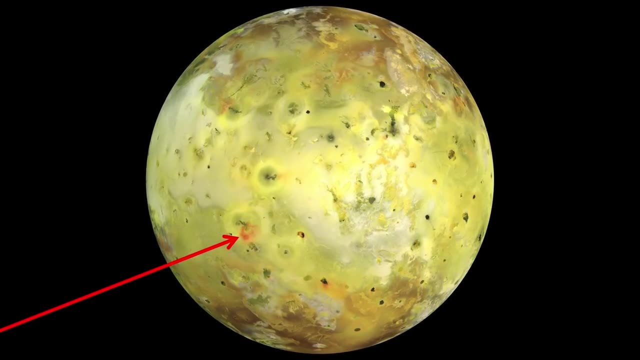 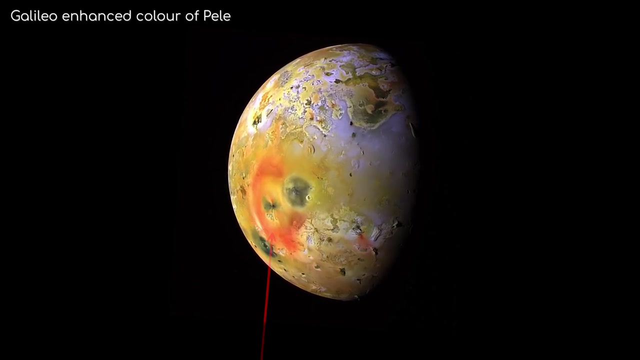 redder than the rest of the planet. In other places, the colours of red are the deposits left by volcanic plumes that reached hundreds of kilometres above Io. The most obvious deposit is from the volcano Pele, Sadly an inactive volcano when Galileo was around, but Voyager. 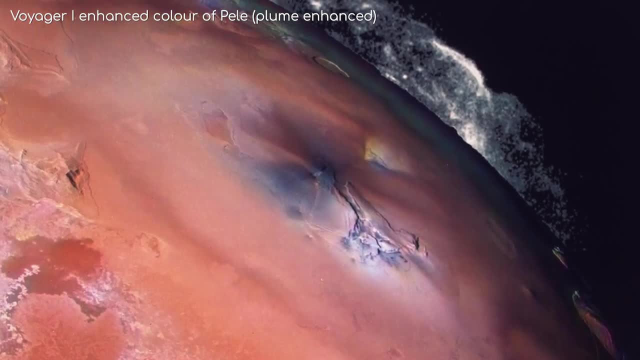 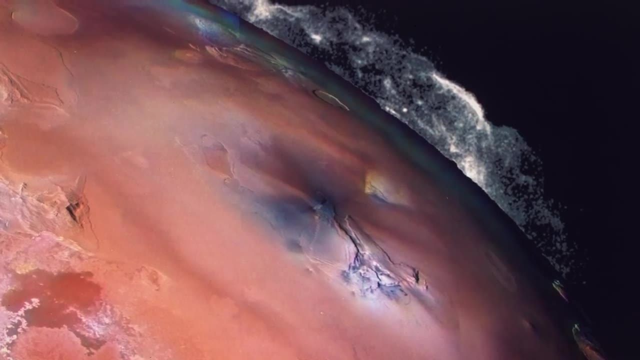 1 was able to see a massive plume when it passed by. In this image, this plume is 300km tall and 1200km wide. 5. Volcanoes in Io, The volcano Pele is 300km wide, in other words, roughly the size of Alaska. Interestingly, 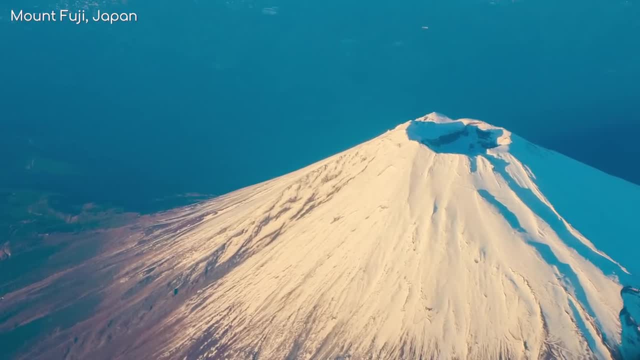 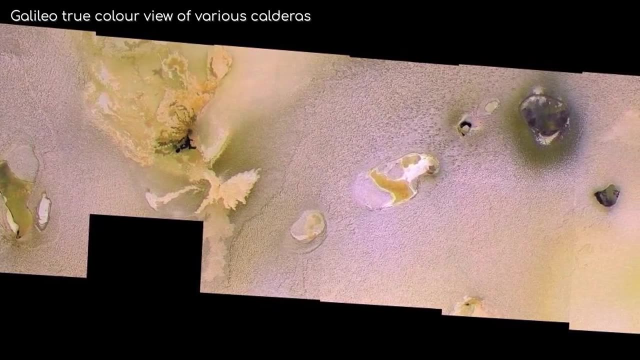 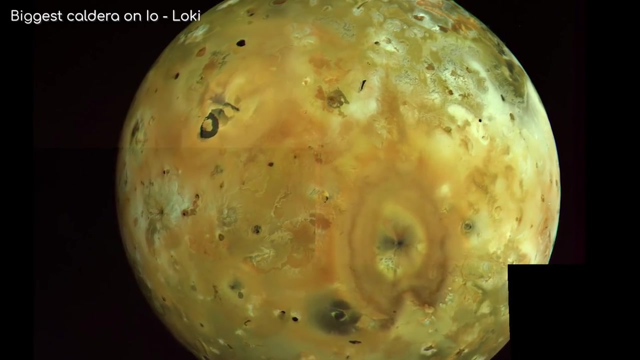 though. the source of lava flows on Earth are typically the depression you would normally see at the top of volcanoes, but these depressions are not found on high peaks on Io. Instead, you have these lava lakes with high walls along the outside. Here is Loki the largest. 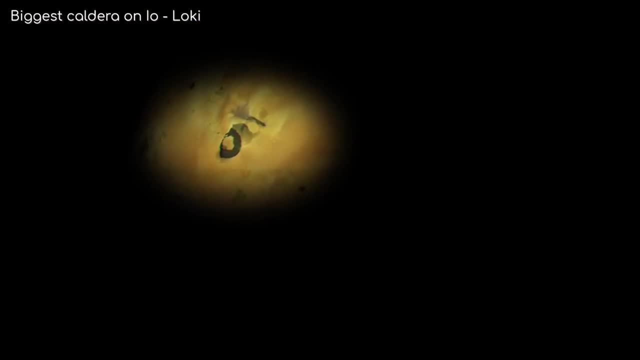 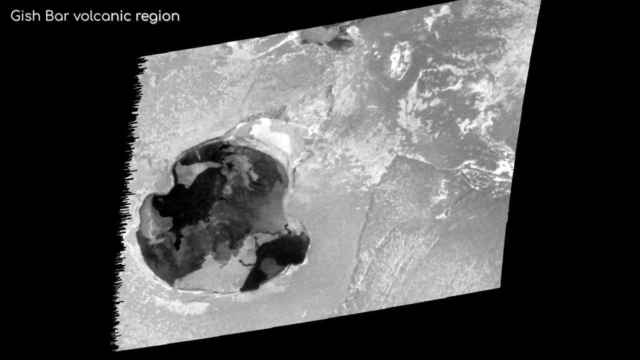 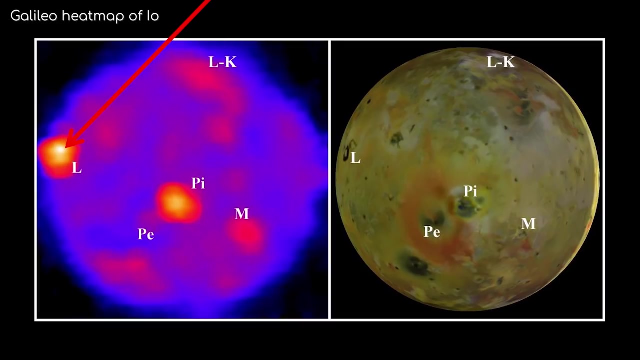 volcano depression on Io, 200km in diameter. 6. Volcanoes in Io. These lakes are directly connected to the lava reservoir below, but usually have a thin layer of solidified crust on top. On average, Loki produces 25% of the average heat output. 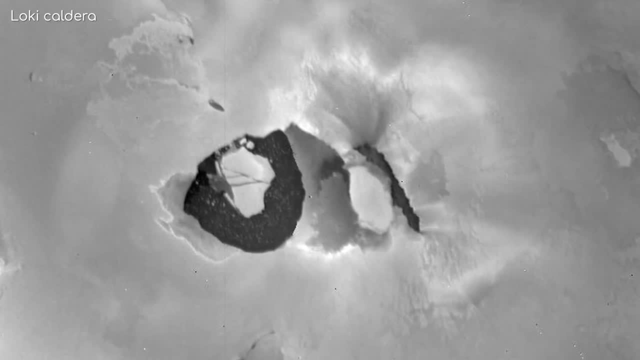 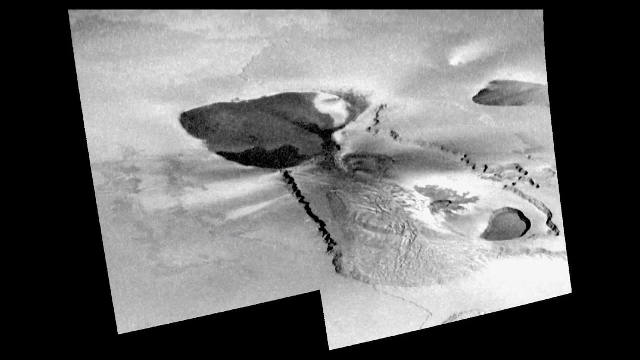 of Io, but sometimes the crust on the lava lake sinks back into the lake, causing Loki to produce 10 times more heat than normal. This can especially be seen in one of Io's other big volcanoes, Tvashtar. Normally this area looks like a volcano, but it's not. 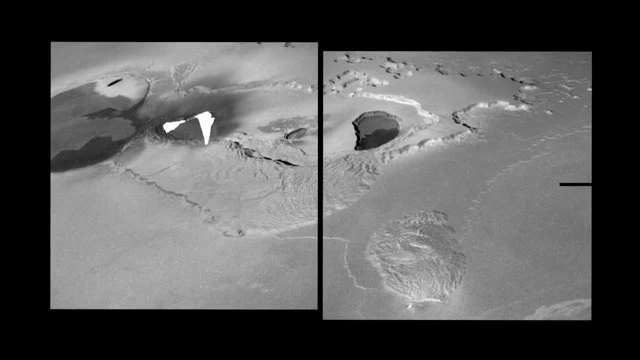 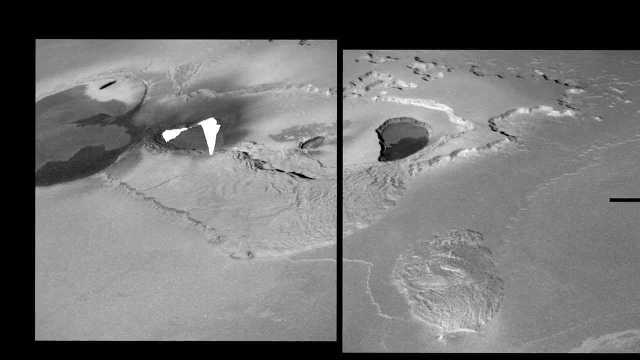 7. Volcanoes in Io. In Io, the lava layer looks like this, But here the crust is seen falling into the lava lake In this image, where there is just white. the radiant energy from the lava curtain was so intense that the camera only registered white. 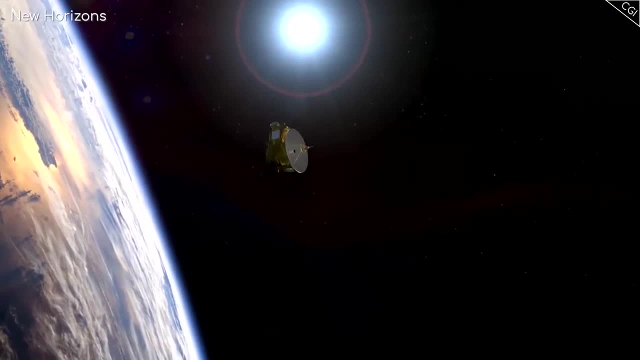 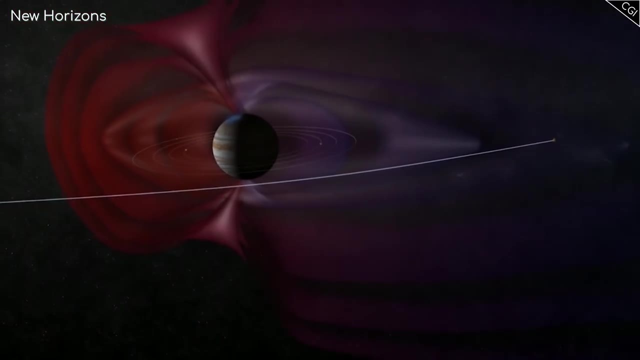 8. Volcanoes in Io. In 2007,, New Horizons used Jupiter as a gravity assist on its way to Pluto. It also used the opportunity to test its equipment. It focused its lens on Io during its flyby. and what? 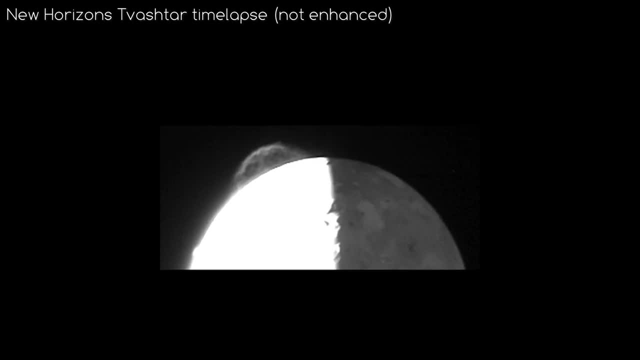 it saw was amazing. It took a picture of Jupiter's surface surface and it was able to see Jupiter's amazing Tvashtar. the volcano I just mentioned was in full eruption and the plume could be seen hundreds of kilometres above Io's surface. You can also see smaller eruptions. 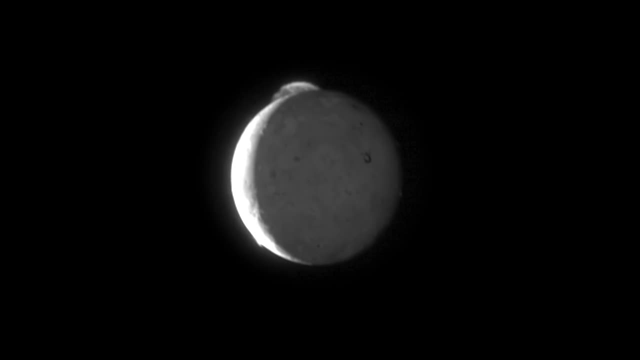 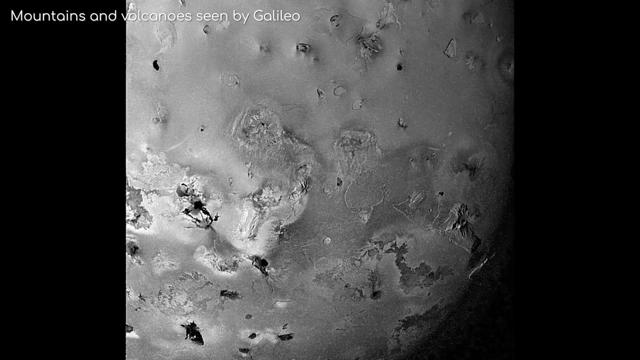 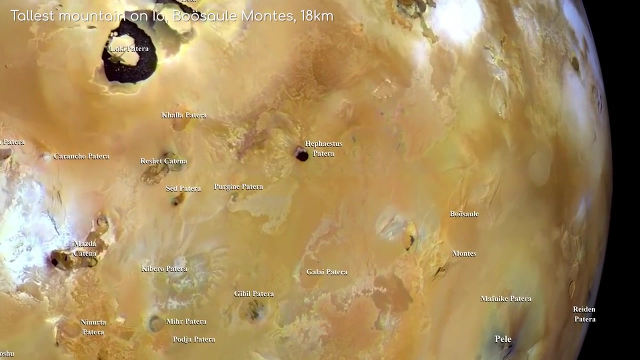 around the moon. I must admit, this is one of the most impressive things I've ever seen of space. Even though the volcanoes tend to be flat, it also has some extremely tall mountains, the highest one reaching 18 kilometres tall. These mountains tend to be completely by themselves. 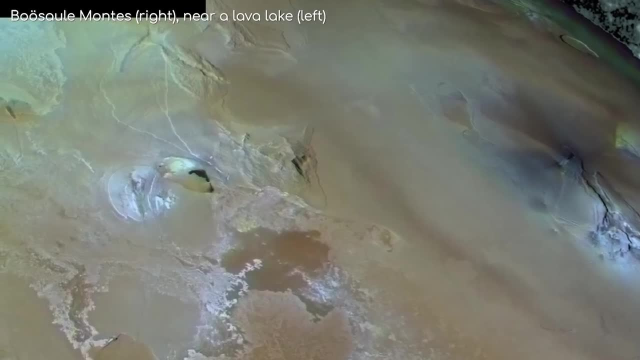 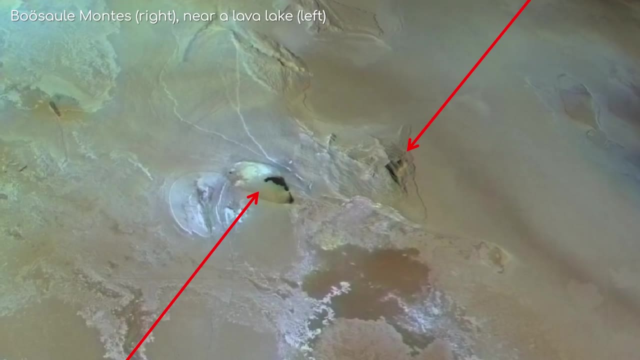 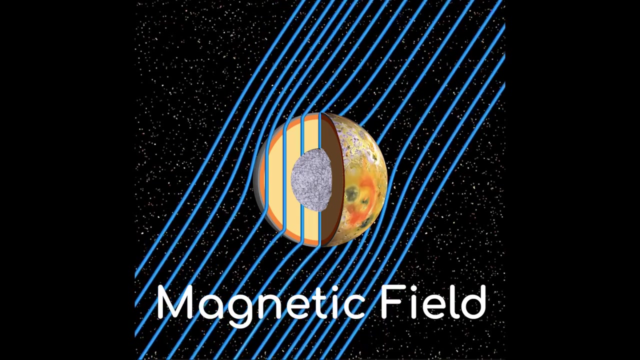 not as part of a ridge or a range. Although most are not volcanoes, lava lakes are found near them, indicating there are faults in the crust near these mountains. Another of the unique aspects of Io is its interaction with the magnetic field of Jupiter. 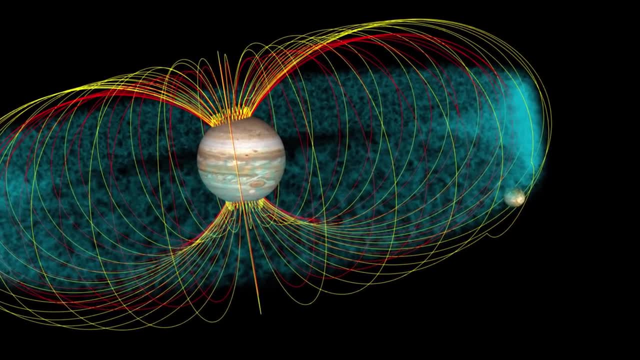 Jupiter has an extremely large and strong magnetic field and it is known for its magnetic field. Jupiter has an extremely large and strong magnetic field and it is known for its magnetic field. Jupiter has an extremely large and strong magnetic field, and Io orbits. 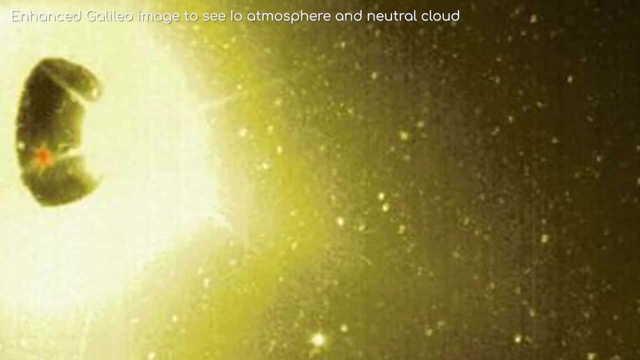 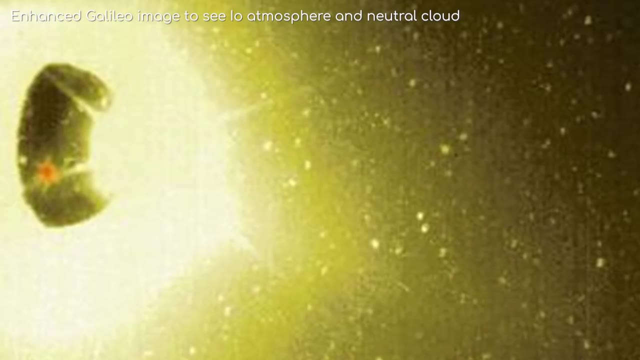 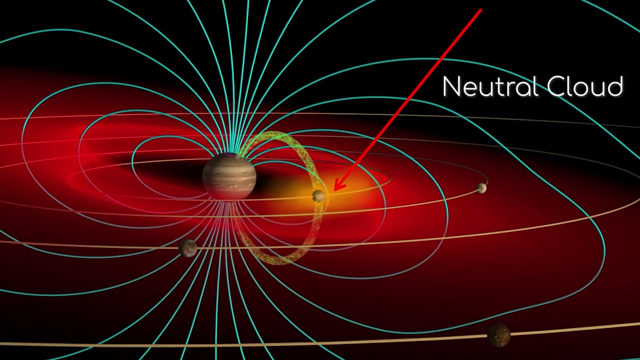 within some of the strongest sections. The unusual thing about this interaction is that when particles from some of Io's thin atmosphere and its eruptions are lost to space, these particles float in orbit around Jupiter in what is known as a neutral cloud. This cloud 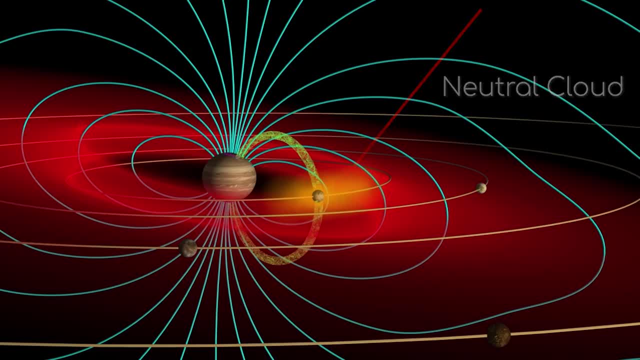 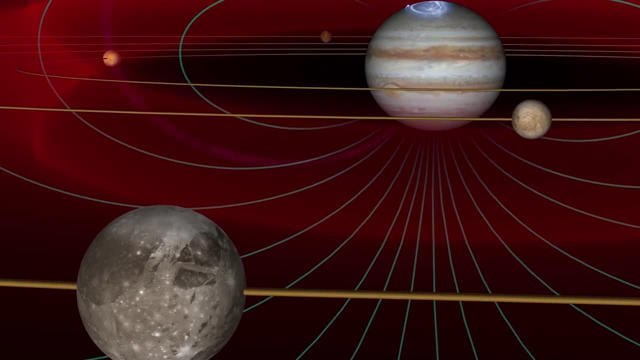 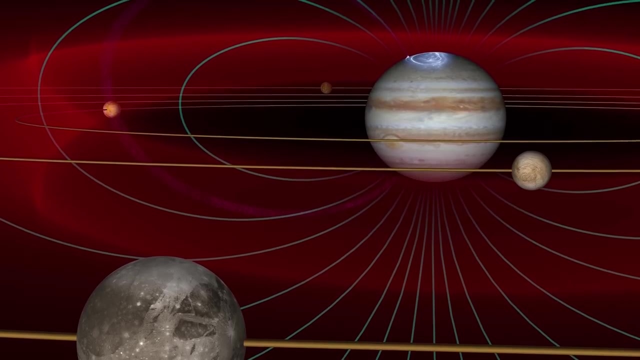 can extend far beyond and behind the orbit of Io, but also surrounding Jupiter is something known as a plasma torus. This is known as the plasma torus, a donut of ionised particles that follow the rotation of Jupiter's magnetic field. The plasma torus rotates a lot faster than Io's orbit, at 70. 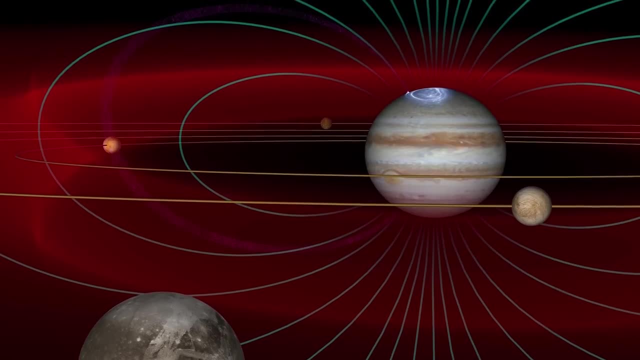 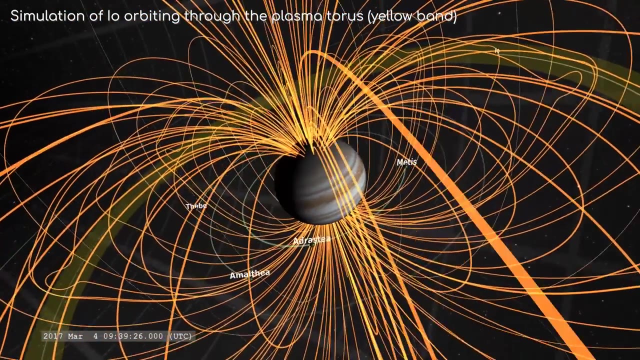 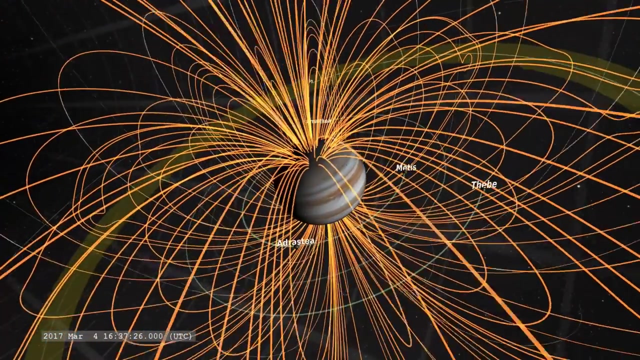 kilometres per second, compared to Io's 17 kilometres per second orbital velocity. Io orbits right through the middle of it, with the particles from the torus bombarding the particles in the neutral cloud, exciting them to higher energies. These newly ionised particles. 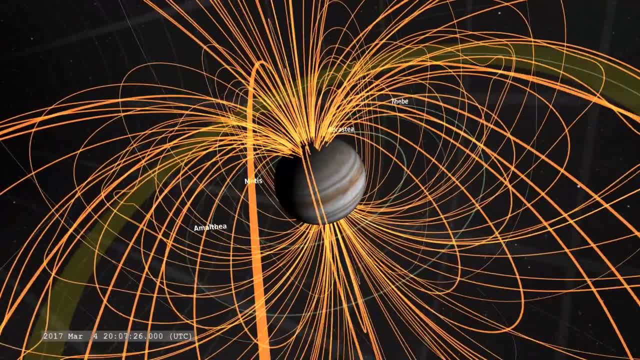 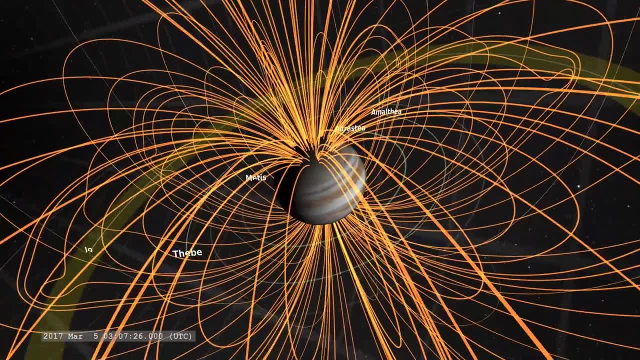 feed into the torus and produce an analytical energy called the ionization energy. This energy torus attracted by the magnetic field lines of the magnetosphere. These particles are lost from the neutral cloud into the plasma torus at a rate of about 1 tonne of matter. 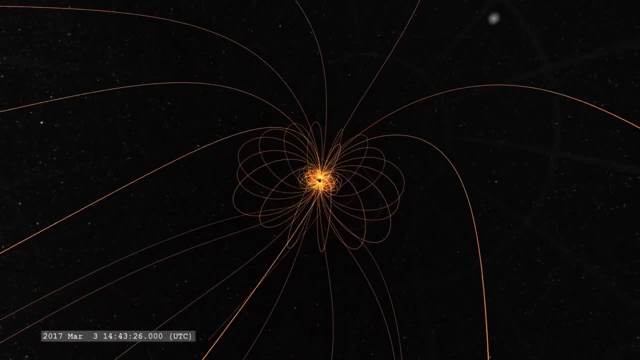 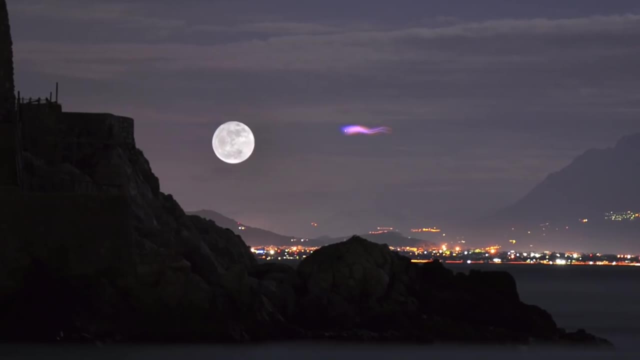 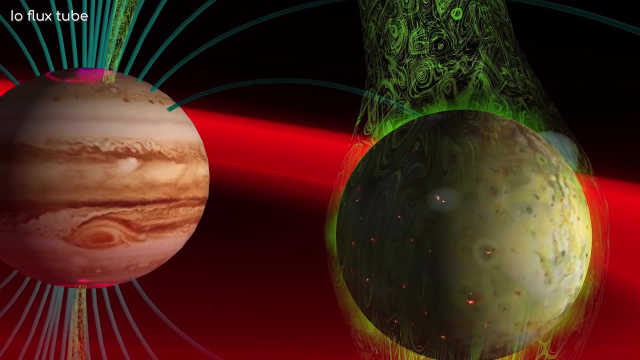 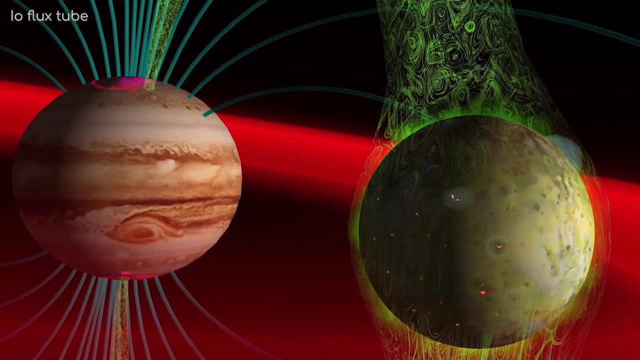 per second, which greatly increases the size of Jupiter's magnetic field. In fact, if it was visible, Jupiter's magnetosphere would be about the same size as the Moon in our sky. Io's interaction with Jupiter doesn't end there. Jupiter's magnetic field lines, which Io crosses, couple Io's atmosphere and 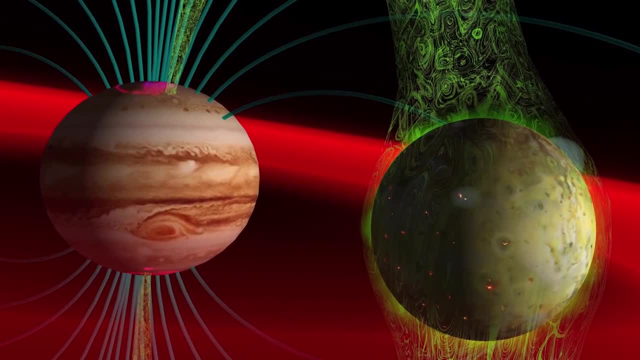 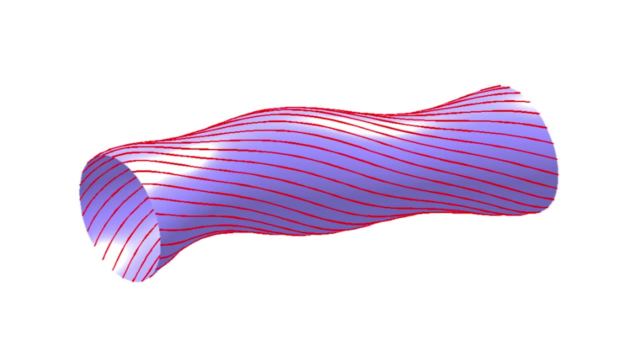 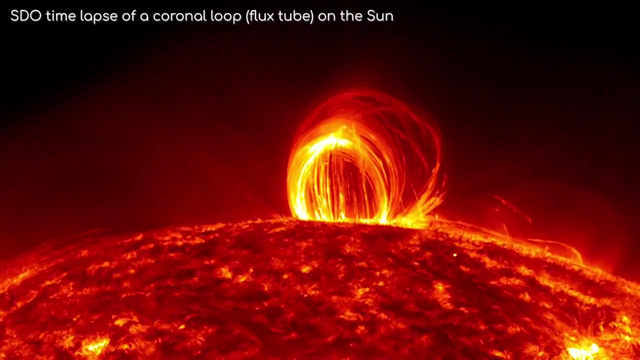 neutral cloud to Jupiter's polar upper atmosphere by generating an electric current known as the Io flux tube. A flux tube is basically a concentration of magnetic field lines. The Sun has these between sunspots and the ion is very visible on the Sun because of the charged plasma that flows between them. 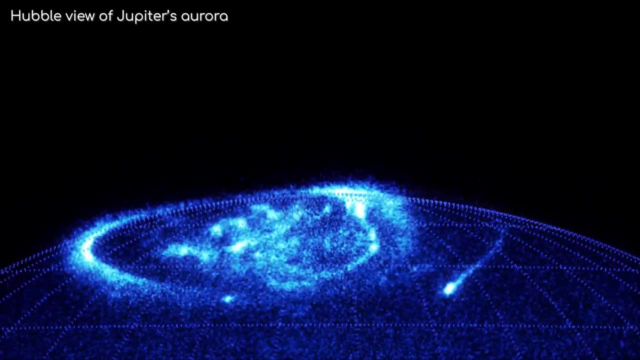 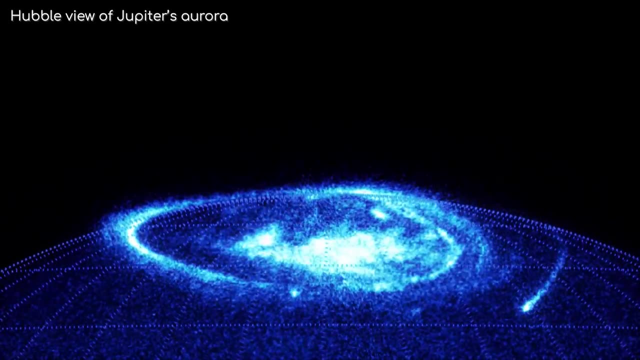 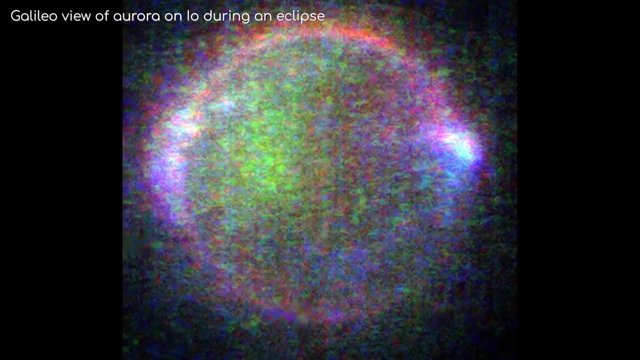 Io's flux tube causes an aurora trail around Jupiter's poles. This point here is the flux tube from Io striking the upper atmosphere of Jupiter. Aurorae are also visible on Io, although they are not just limited to the poles. The different 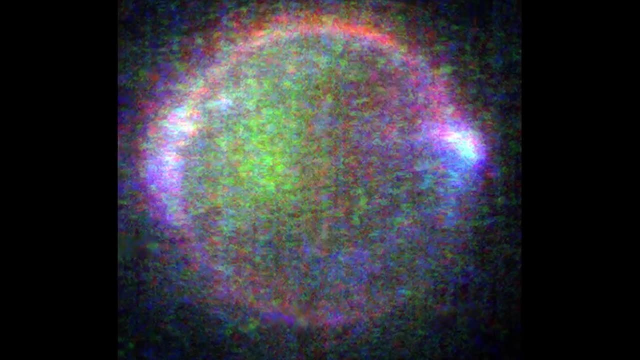 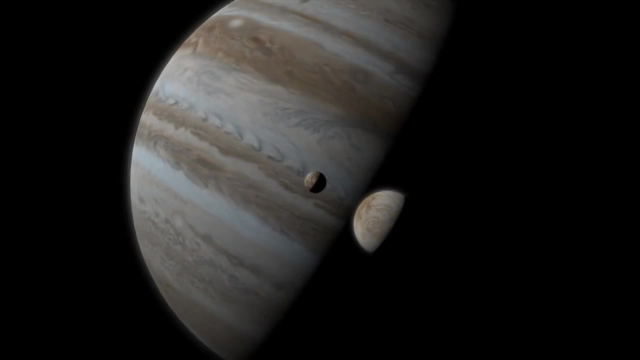 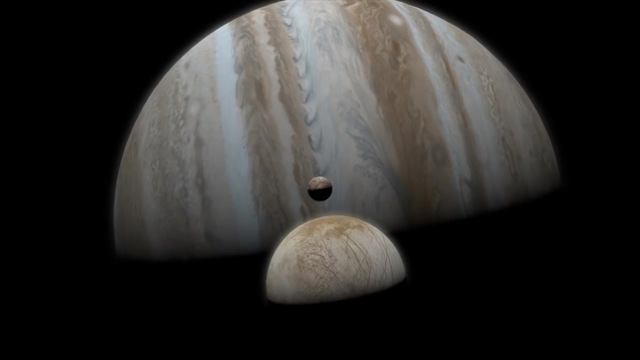 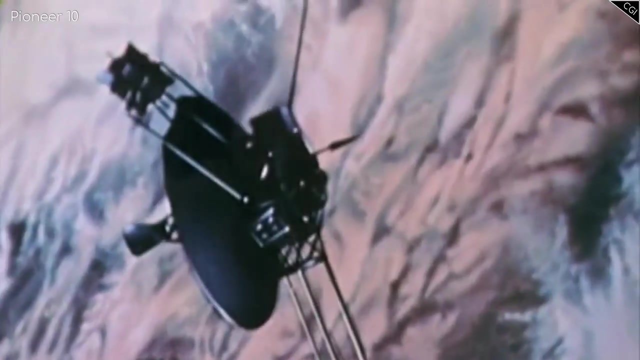 colours represent the different particles being ionised: green is sodium, red is oxygen, blue from sulphur. Europa, One of the most exciting moons in the entire solar system. It is a beautiful world filled with mysteries. This is the first ever close-up image of Europa taken by the Pioneer probe back in 1973.. Since then, we've had the Voyager and Galileo probes explore the moon and with each visit, Europa has never failed to surprise us. We are yet to solve a lot of Europa's puzzles, but there are many things that we are starting to piece together. 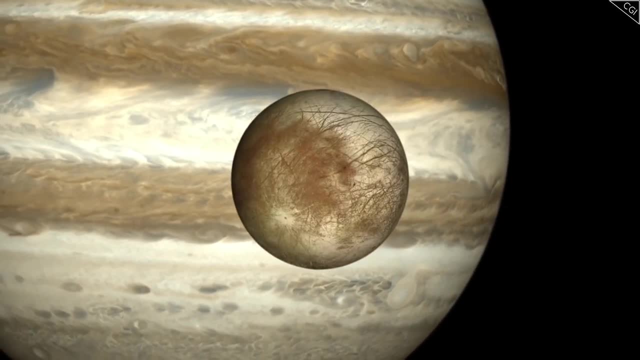 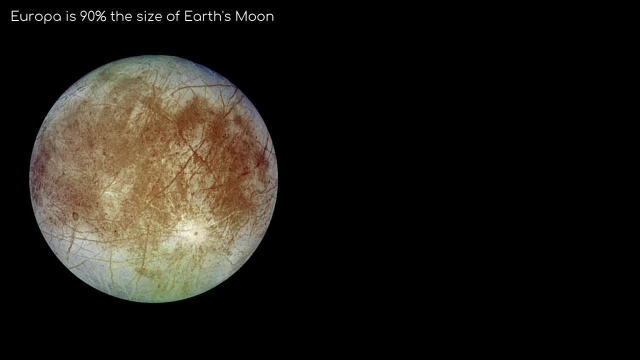 Let's first of all see where Europa fits into the Jovian system. Europa is the second and smallest of the four Galilean moons, although it's still the sixth biggest moon in the entire solar system, just behind Earth's moon with a diameter. 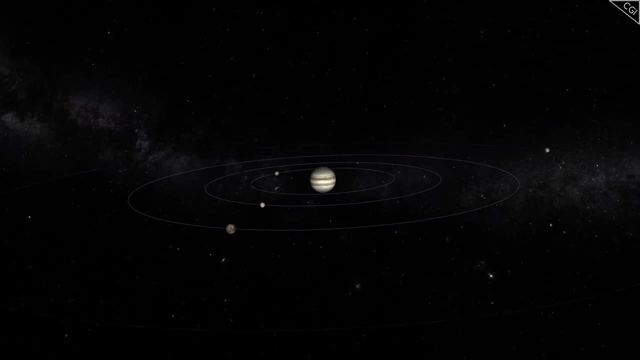 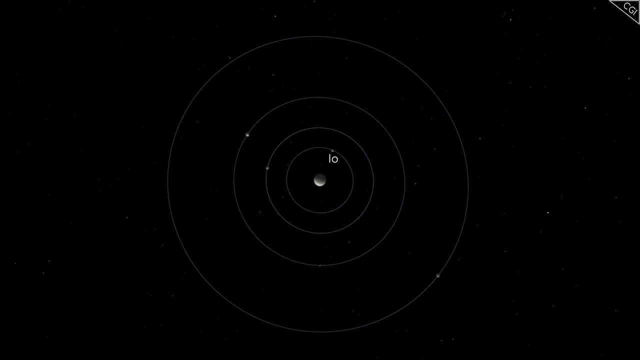 of about 3000km. It takes Europa 3.5 miles to reach Europa. However, Europa is only 3.5 days to orbit Jupiter once. Interestingly, the first three Galilean moons, Io, Europa and Ganymede, are locked in a 4-2-1. 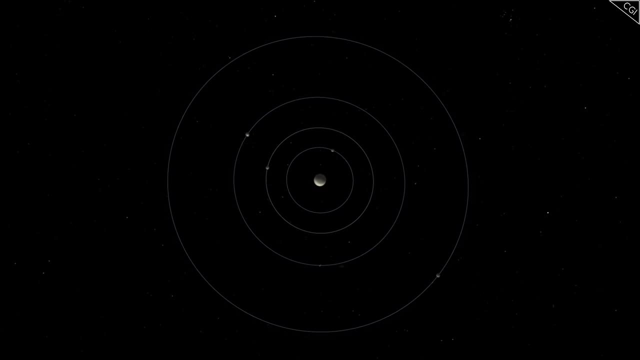 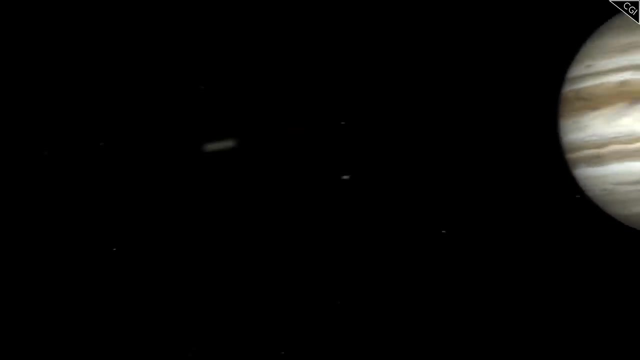 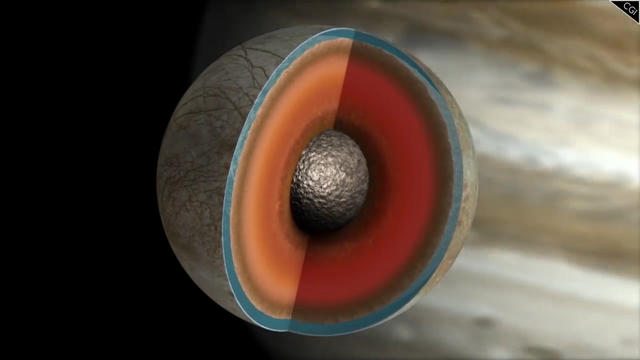 orbital resonance due to their gravitational influence with each other. This orbital resonance and the constant gravitational tugging from the other moons keeps the orbit of Europa from ever becoming completely circular. Due to Europa's slight ecliptical orbit, the magnitude of the gravitational force acting 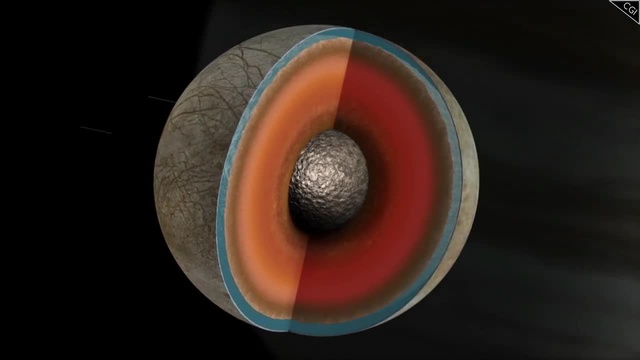 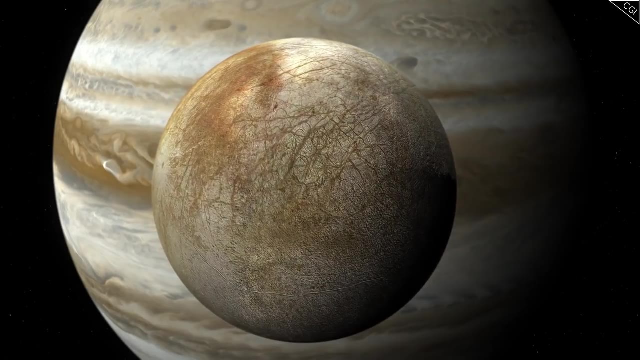 on it from Jupiter is very small. It increases and decreases as it orbits. This creates tides that stretch the moon's surface. These forces are significant as they have a big influence on the moon's appearance and what goes on under the surface. 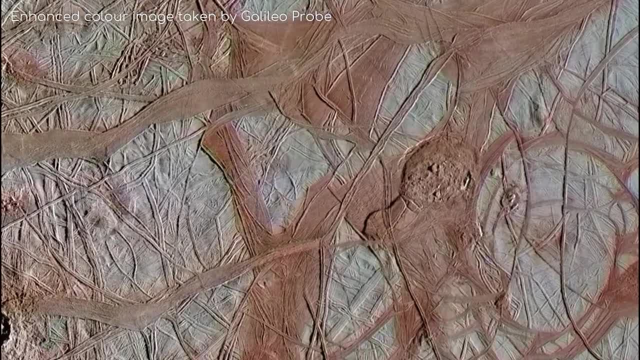 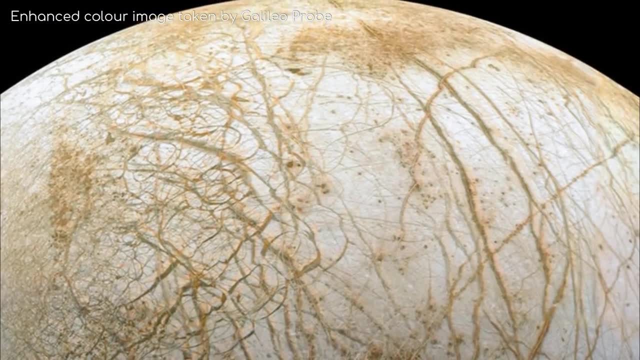 Europa's surface is made predominantly of water ice. As you can tell, it looks very remarkable and distinctive due to these long, continuous fractures and cracks. These are called lineae, which translates to lines in Latin. These are called lineae, which translates to lines in Latin. 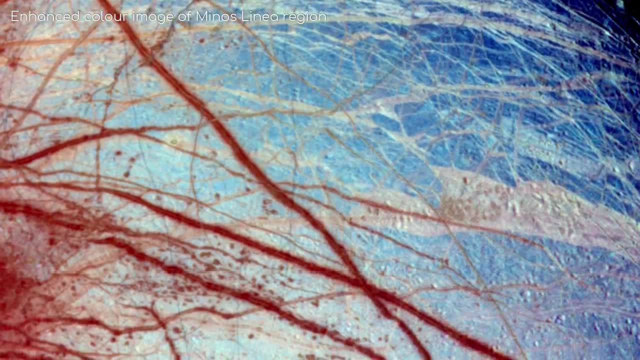 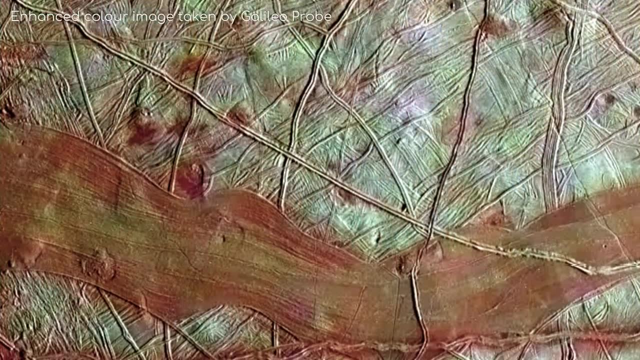 These are called lineae, which translates to lines in Latin. These are called lines in Latin. These lineae are often only about 1-2km wide, but can extend for thousands of kilometres across the moon's surface. We aren't sure how or why these lineae are formed at present, but the most likely theory 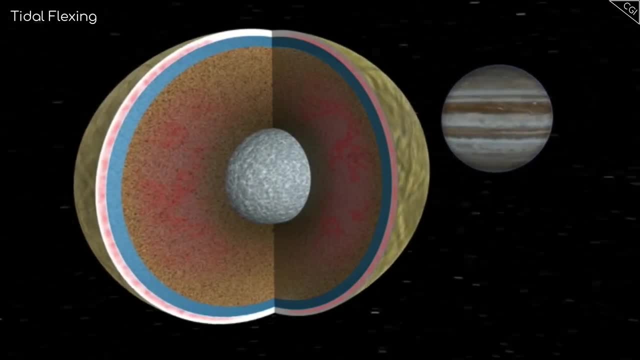 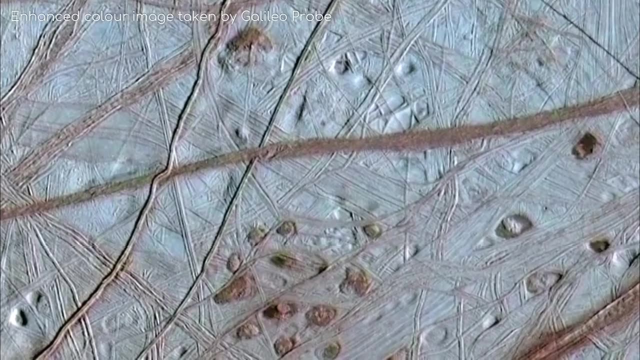 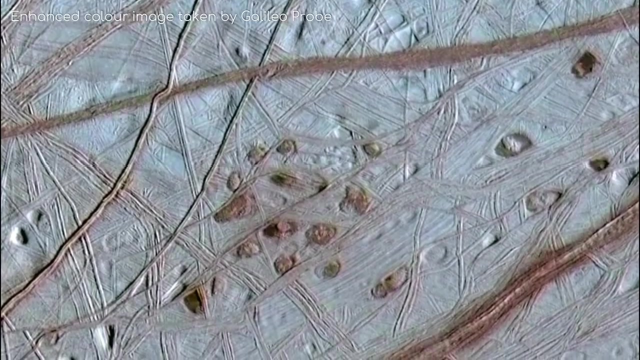 is that, as the crust pulls apart from tidal flexing, warmer material from beneath fills the gap in a similar fashion to the ocean ridges on Earth. In this image taken by the Galileo spacecraft, you will notice some dark brown spots. They are very small, only about 10km across, and they are known as lenticulae. 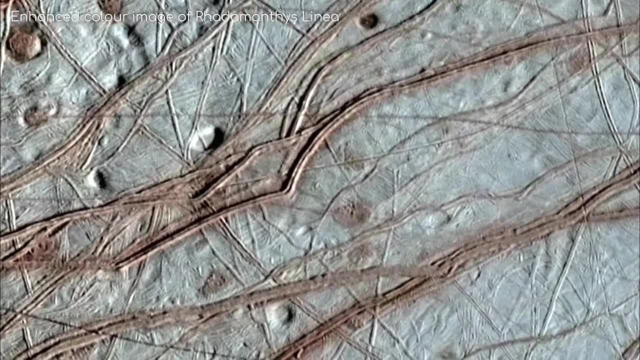 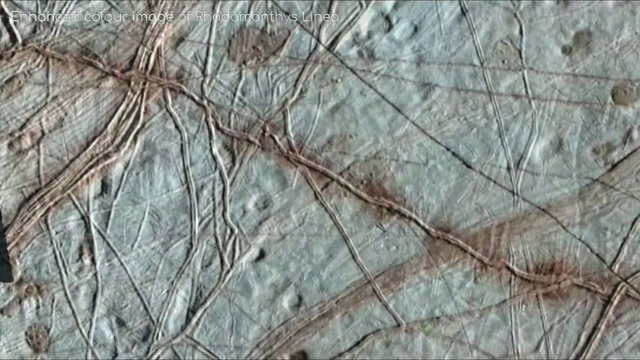 They are also believed to be formed by the upwelling of hot, less dense material to the surface, either by pushing the existing crust up or by breaking through altogether. Should the underground material have broken through, what we can then see are these strange? 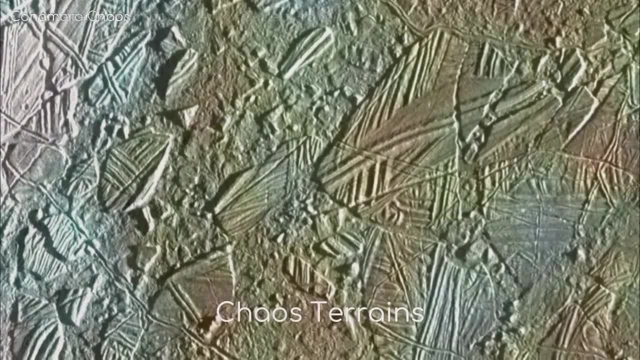 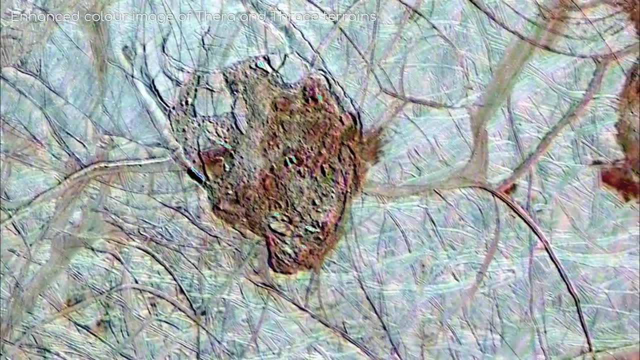 unusual terrains called chaos terrains. They are really rough patches surrounded by a rather smooth surface. They are also believed to be formed by the upwelling of hot, less dense material to the surface. These spots are expected to be soft and may contain significant information about. 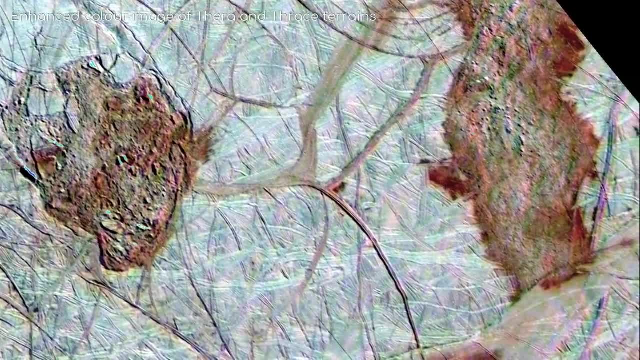 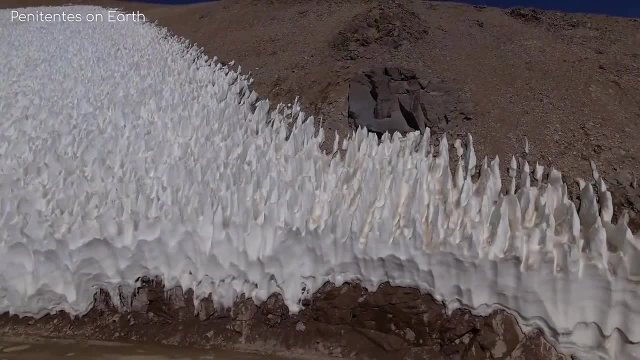 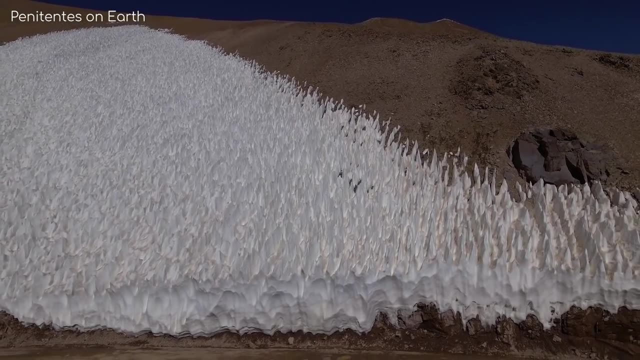 what's under Europa's surface, which we will get to later in the video. Data from Galileo also indicated that Europa's equator may be covered in icy spikes called penitentes. These vertical cracks may be up to 15m high and will have formed from direct overhead. 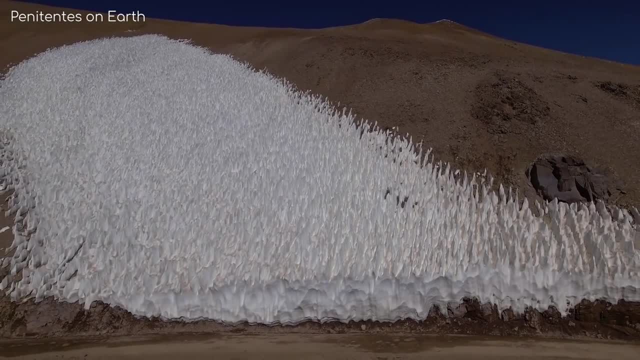 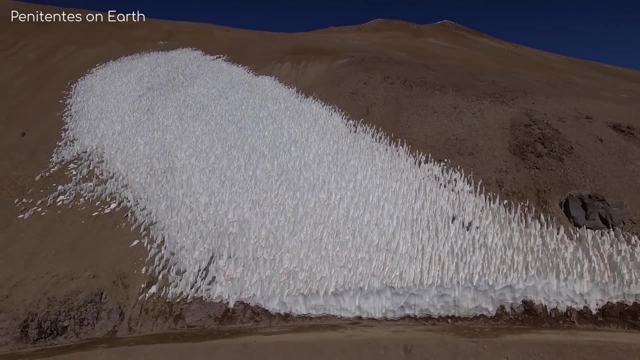 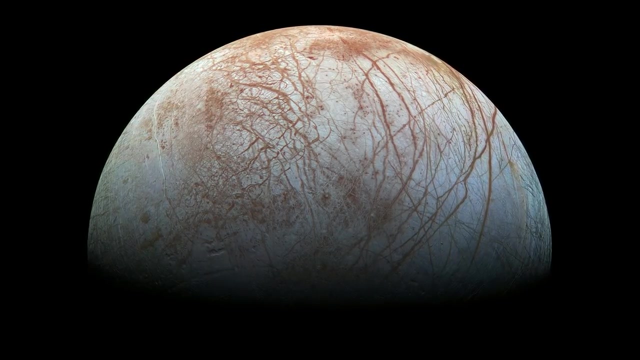 sunlight on the equator. Interestingly, penitentes are found on Earth too. They can be found at high altitudes, although nowhere near as large as on Europa. Despite being roughly the age of the solar system, Europa barely has any craters. 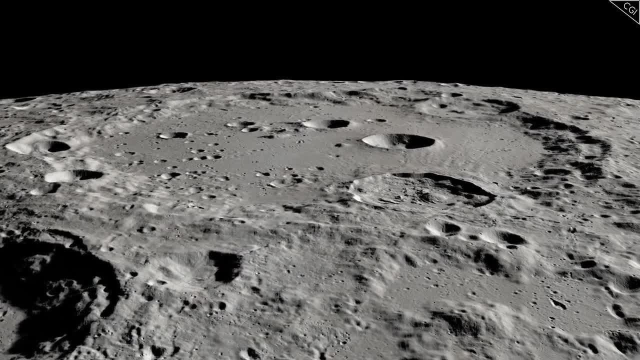 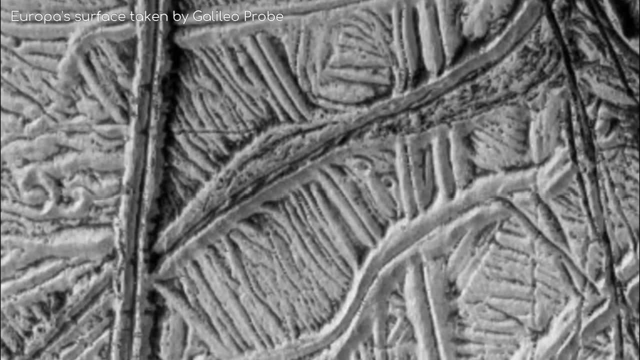 Europa has less than 50 major craters, whereas the Earth's moon has more than 5,000 craters with a diameter above 25km. This indicates that Europa's surface is constantly changing and reforming. Models suggest that Europa's surface is only about 30 to 180m high. 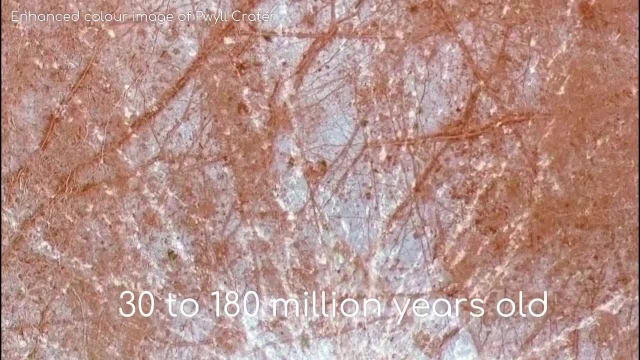 This means that Europa's surface is constantly changing and reforming. Models suggest that Europa's surface is only about 30 to 180m high. This means that Europa's surface is only about 30 to 180m high. Europa is about 4,000m long, which is very young in geological terms. 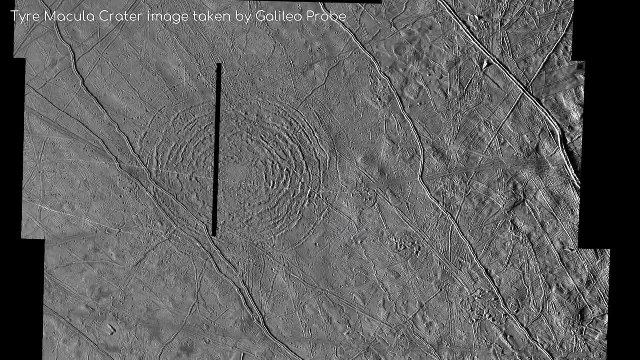 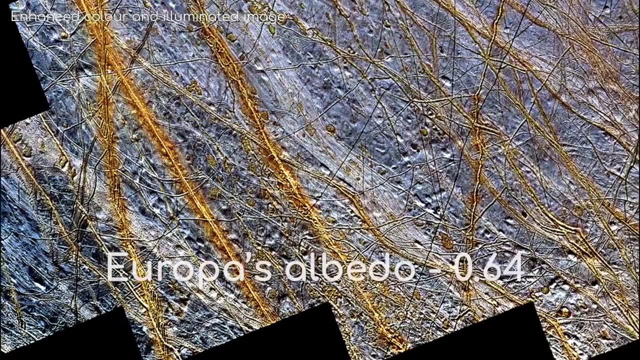 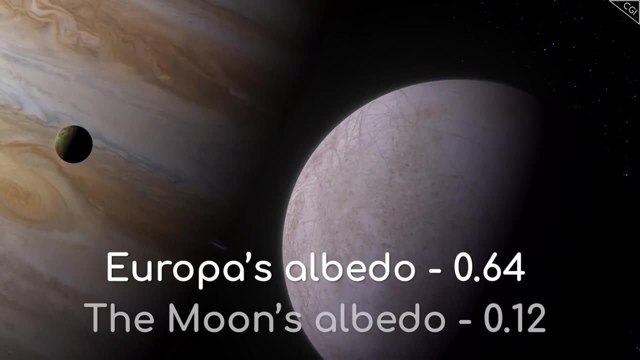 Additionally, Europa's icy surface is the smoothest surface of any known solid celestial object in the entire solar system. Europa's crust also has an albedo, or light reflectivity, of 0.64,, one of the highest of all moons. Europa's albedo makes Europa five times brighter than our Moon. 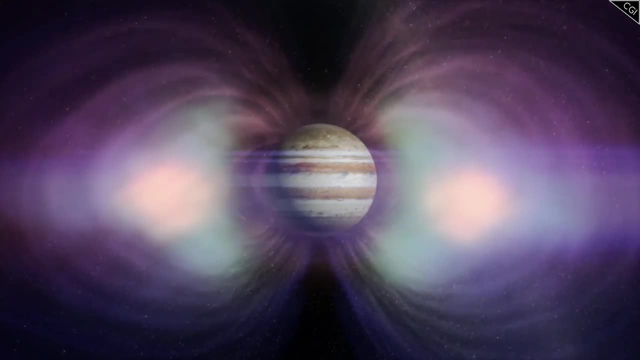 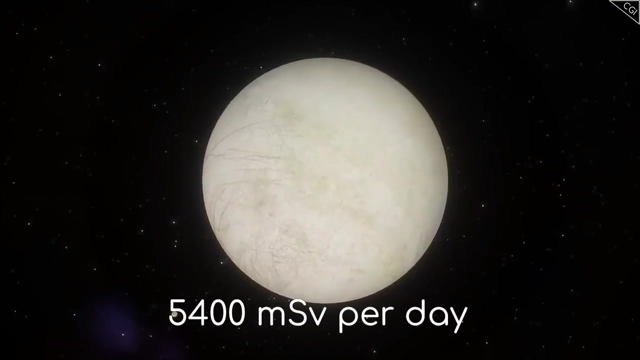 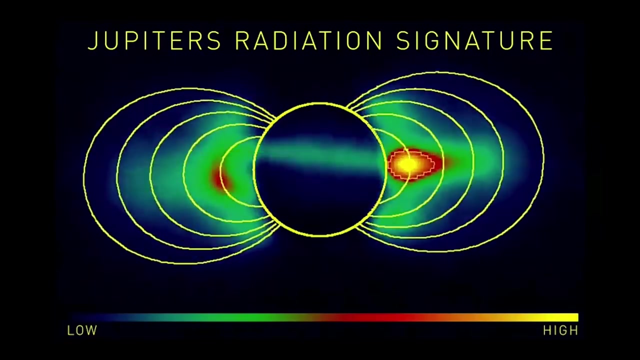 Europa's surface is being dominated by a constant and intense blast radiation from Jupiter. The radiation level at the surface of Europa is equivalent to a dose of about 5400 mSv per day. Exposure to radiation at that level would be enough to kill a human in a single day. The reddish-brown colour spread across the cracks and fractures. 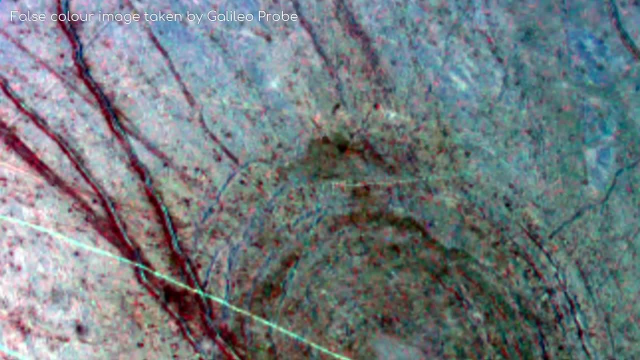 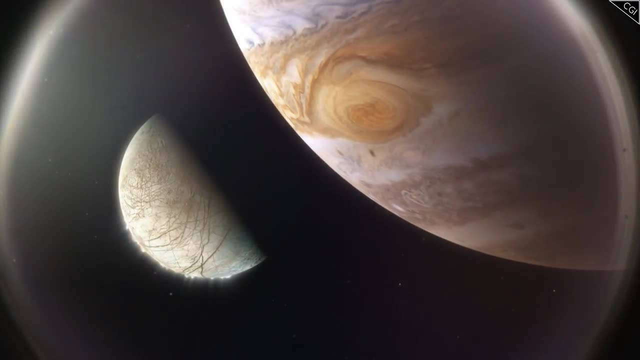 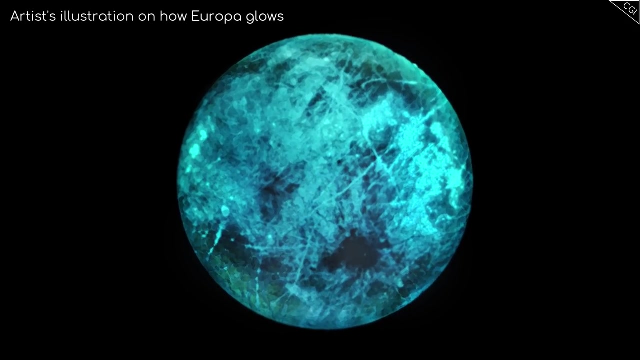 of the Moon is believed to be due to salt and sulphur compounds mixing with water ice and then modified by Jupiter's radiation. A recent study from JPL suggests that Europa might even glow in the dark. Energetic ions from the radiation penetrates the surface. 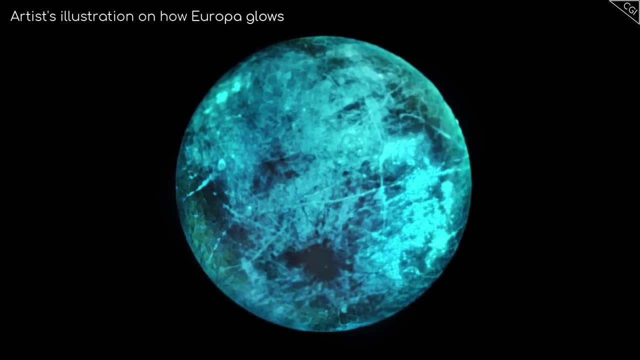 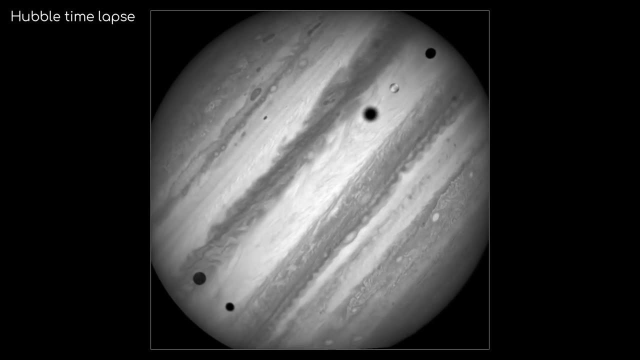 which would energise the molecules beneath, which would make them release energy as visible light. Unfortunately, we cannot see Europa's dark side from Earth, as we are between it and the Sun always, so we are going to have to wait for future missions to Europa before. 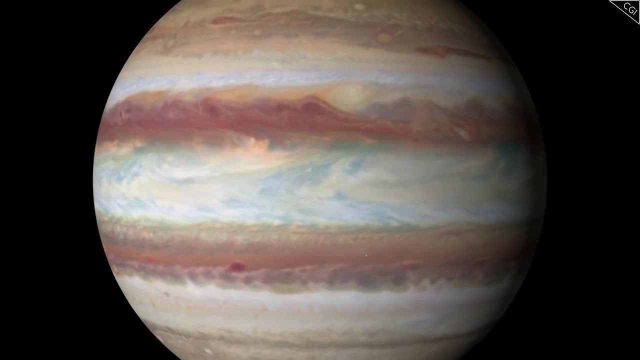 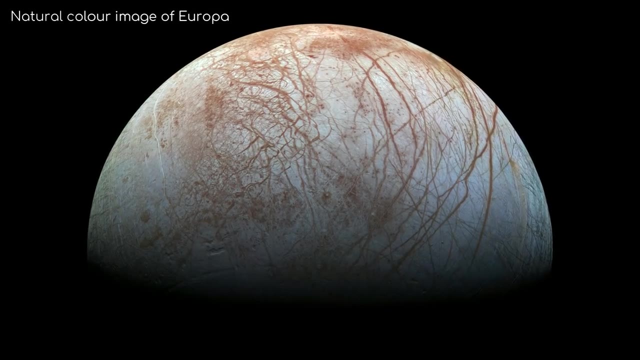 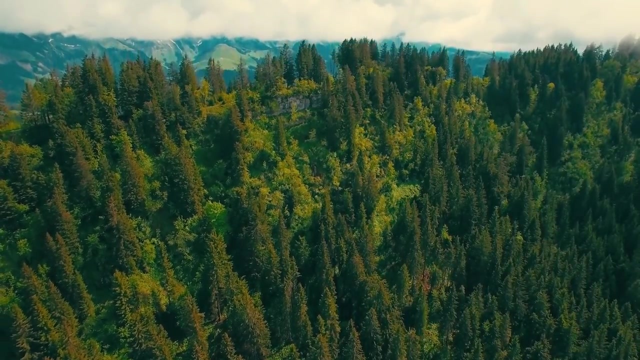 we know it, We can prove this- Radiation received from Jupiter plays a significant role in Europa's atmosphere as well. Europa has a very tenuous atmosphere composed primarily of oxygen. Unlike on Earth, the oxygen on Europa is formed by radiolysis, or in other words, the process of radiation bombarding. 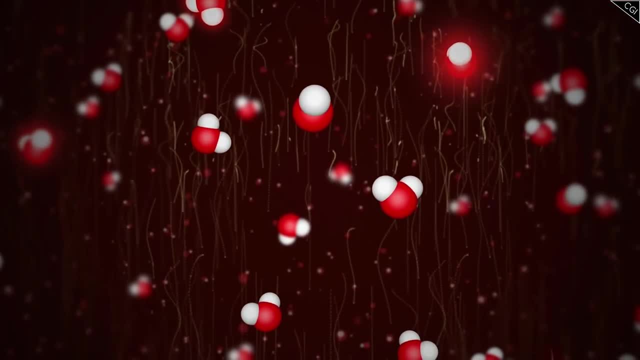 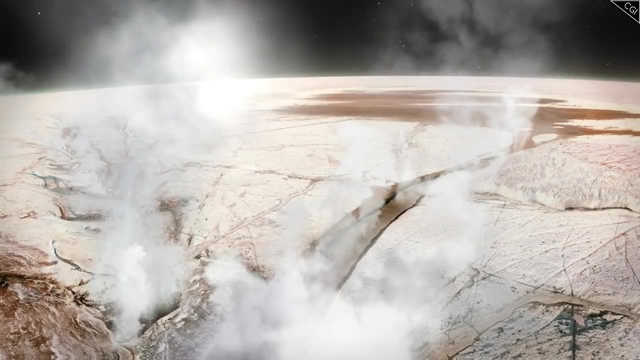 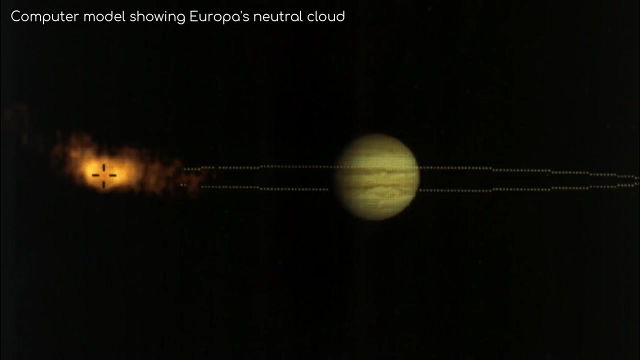 the water ice surface, separating the H2O into oxygen and hydrogen. Hydrogen escapes Europa's gravity altogether. Europa's gravity is so light. however, a lot of the heavier molecular oxygen remains – the hydrogen and oxygen that escape Europa's gravity form a dispersed neutral cloud, which 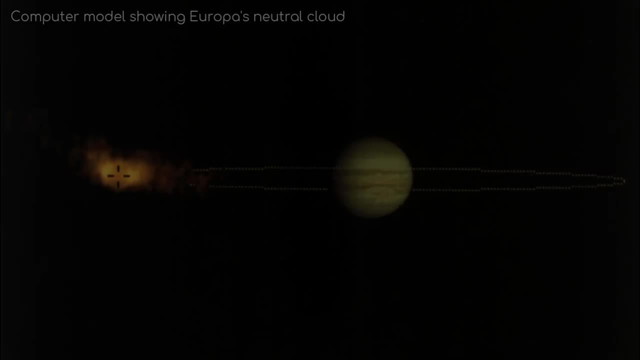 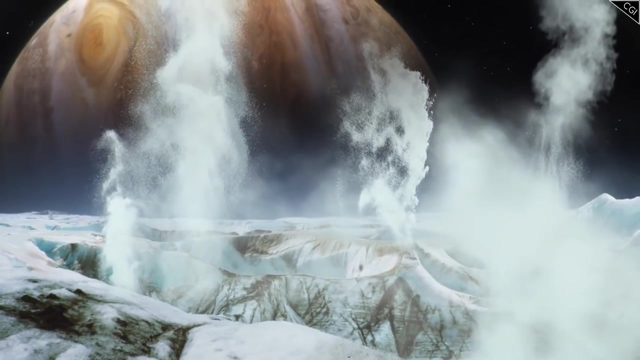 follows the orbit of Europa around Jupiter. In 2012,, the Hubble Space Telescope discovered plumes of water vapour erupting from Europa's South Pole. This image suggests that the water plumes rise up to 200 kilometres from its surface. 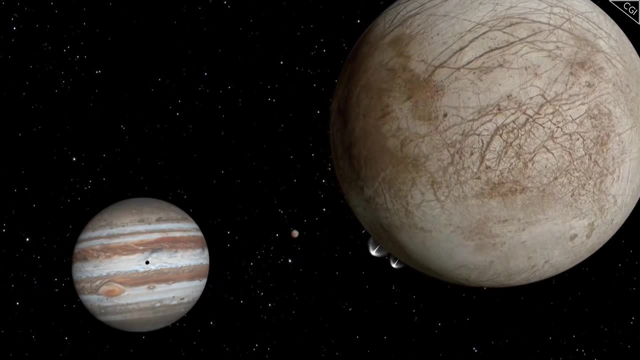 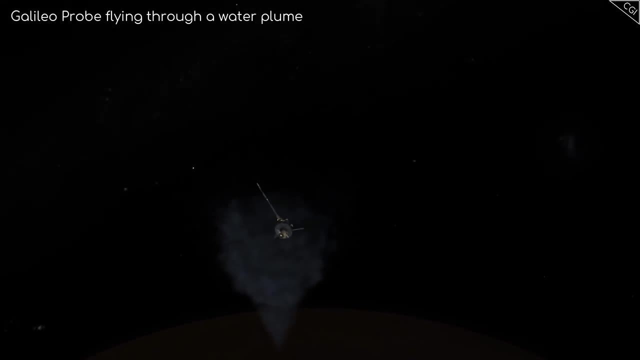 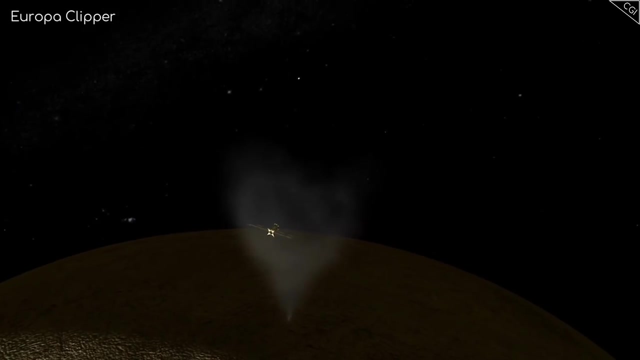 In 2018, astronomers found additional evidence of water plume activity on Europa when they looked back at the old Galileo data. with a new data analysis technique, A dedicated mission studying these plumes can also help us understand what's inside the Moon, without having to land on it, because what may lie underneath that solid ice surface? 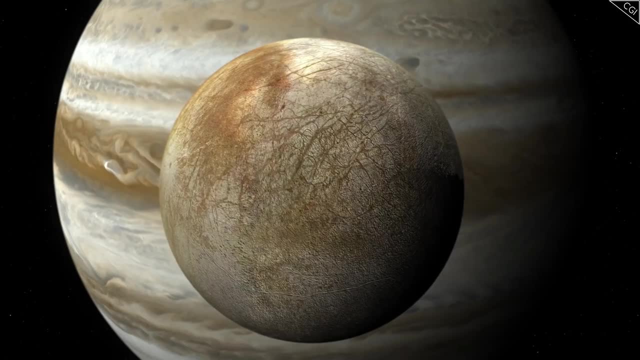 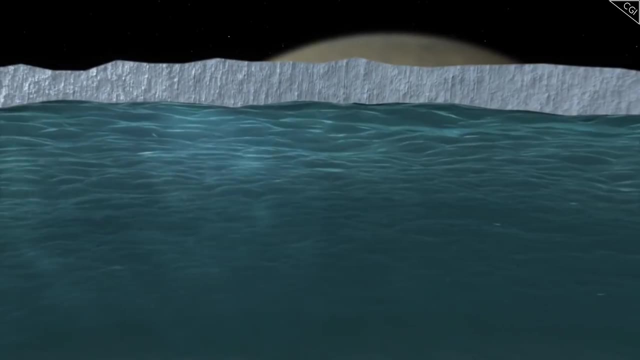 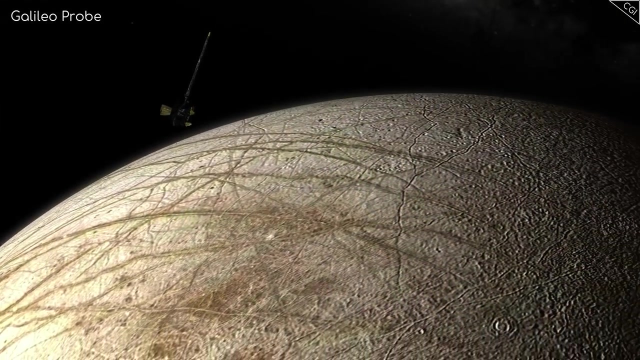 is perhaps the most fascinating thing about Europa. There is likely to be a global ocean between a rocky mantle and the water-ice crust. The first clue that this amazing ocean world was hidden under its surface was provided by the Voyager and Galileo probes in 1979 and the late 1990s respectively. 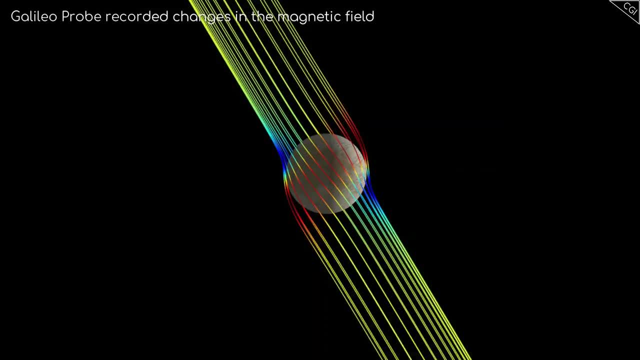 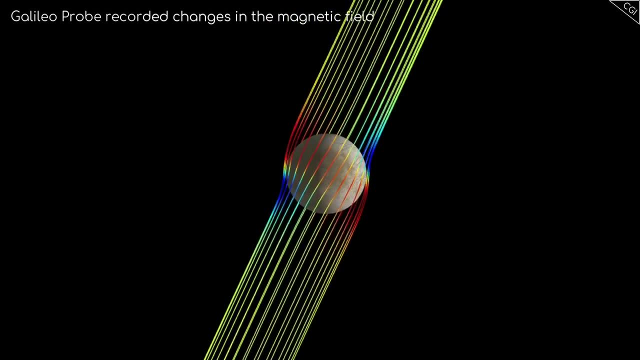 Between these missions, there was a drastic change in the magnetic field of the Moon, which is not possible unless there is some electrically conductive fluid beneath its surface. Europa's crust also indicates this. Europa indicates the presence of a liquid layer beneath it as it rotates with an angle. 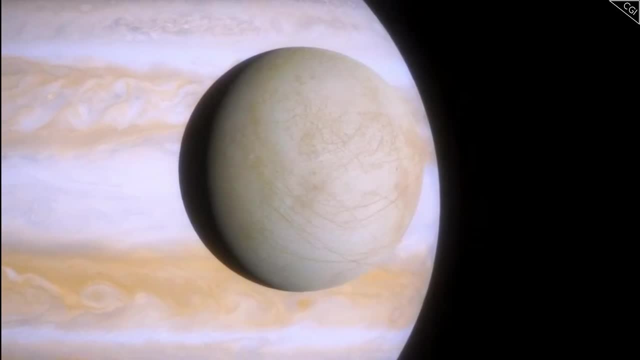 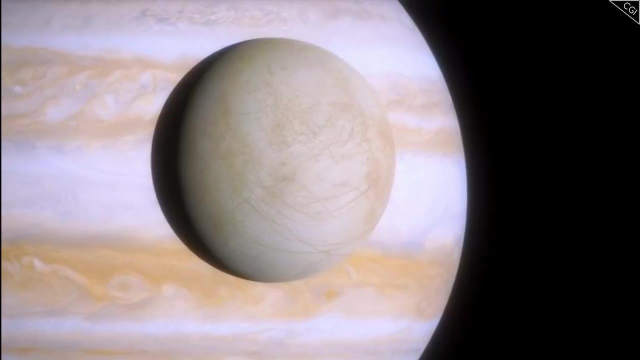 of 80 degrees, which is not possible if the crust and the rocky mantle were mechanically attached. Instead, it is likely that the icy crust floats on the ocean, and it is believed to make one full rotation around the Moon once every 12,000 years. 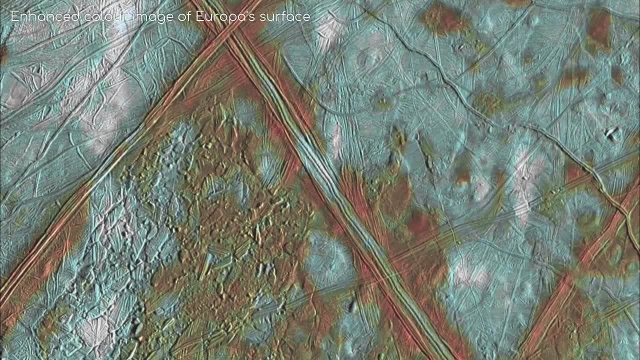 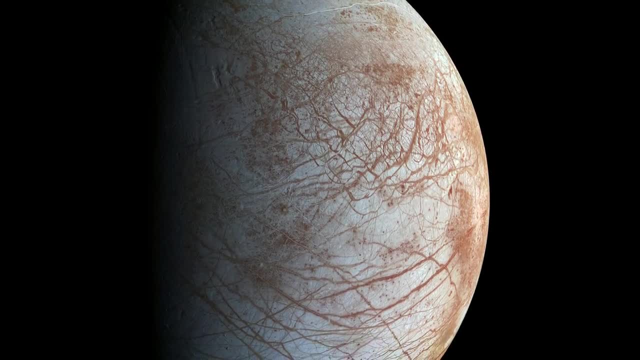 The fact that this ocean is not attached also explains the multitude of lineae on the surface. Tidal flexing should cause lineae to fall off. However, this is not the case. Europa is not the only place where lineae form at specific points on Europa- not all. 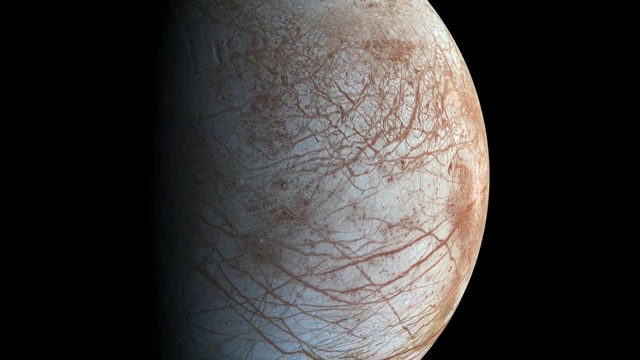 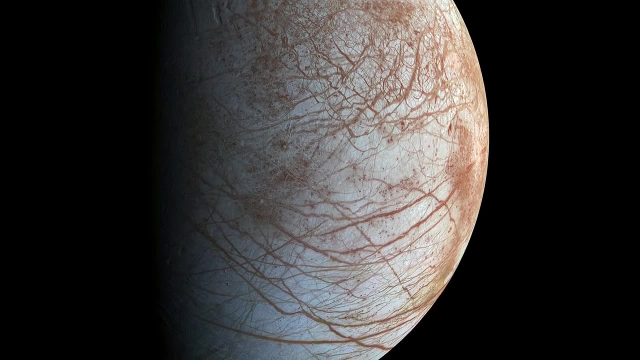 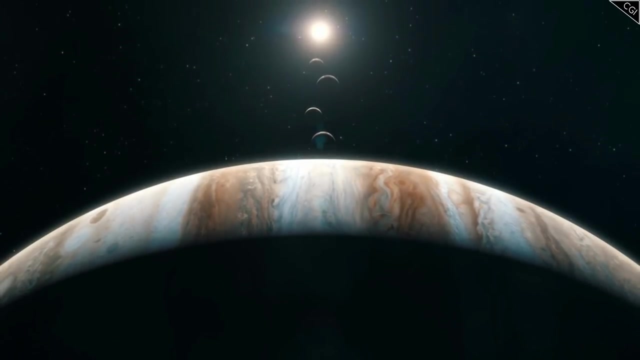 over, However, because the position of the crust changes over time and one spot never stays in the same place for long, hence why more and more lineae form. Europa is 780 million kilometres away from the Sun, which is five times further away. 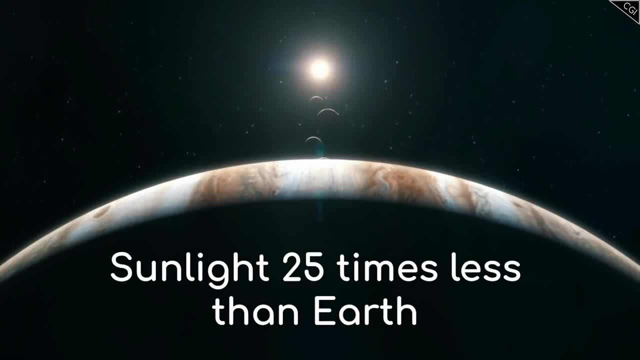 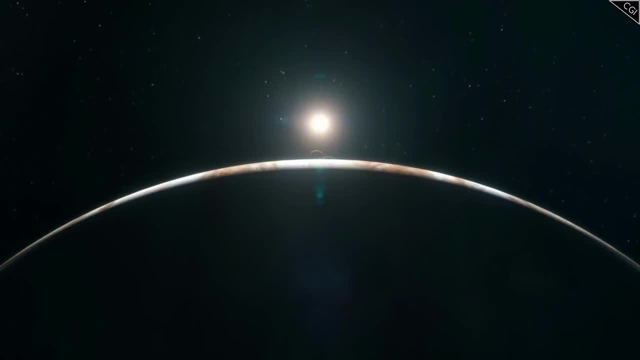 than the Earth. That makes the sunlight about 25 times fainter here. As such, Europa, or any other planet, is only 25 times fainter than the Earth That makes the Sun light about 25 times fainter. here, Europa, or any other moon in the Jovian system for that matter, barely receives any heat. 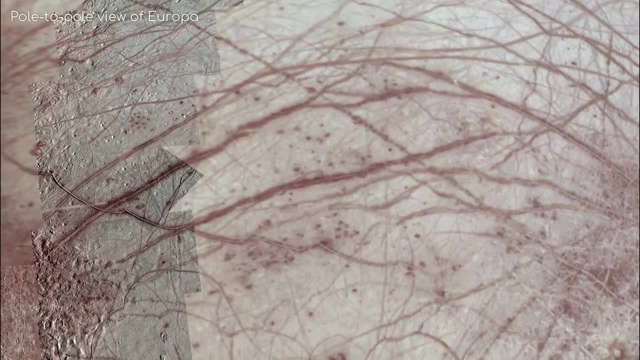 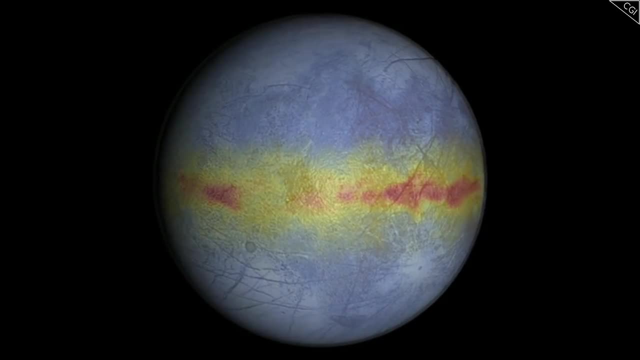 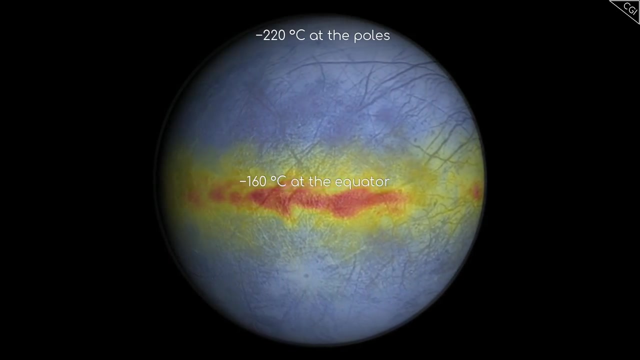 from the Sun, So, unsurprisingly, it's cold enough here that the surface is frozen. In fact, Europa's surface temperature averages about minus 160 degrees Celsius at the equator and minus 220 degrees Celsius at the poles, keeping Europa's icy crust as hard as granite. 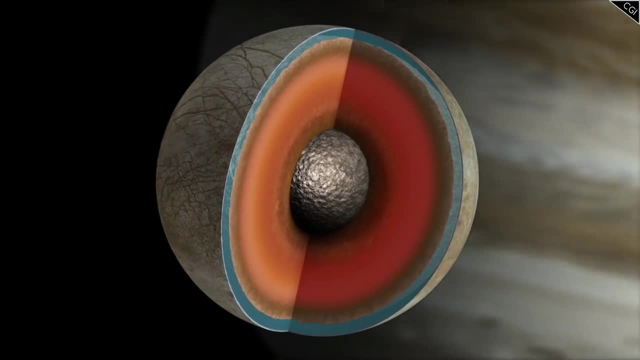 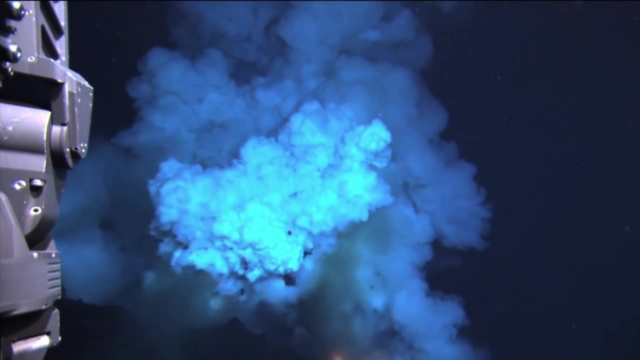 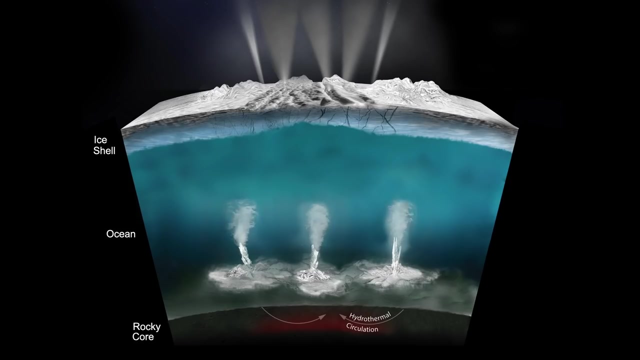 However, tidal pressures exerted on the Moon as it orbits Jupiter heats Europa's core, so geothermal activity from the core should keep the subsurface ocean in a liquid state. This ocean is believed to be under only 15 to 25 kilometres of solid frozen crust. 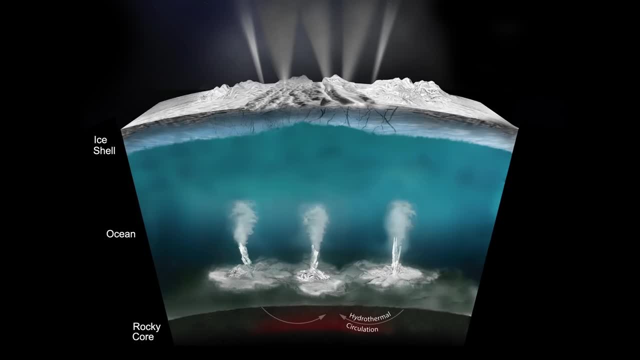 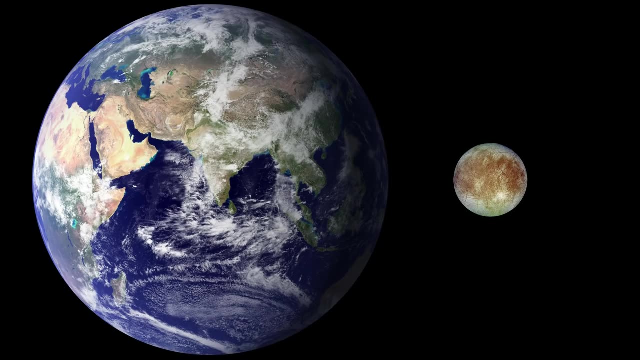 The ocean itself is probably about 60 to 150 kilometres deep. Interestingly, Europa is only one fourth the diameter of Earth, although it may contain twice as much water as all of Earth's oceans combined. What's most surprising is that Europa is only one fourth the diameter of Earth, although 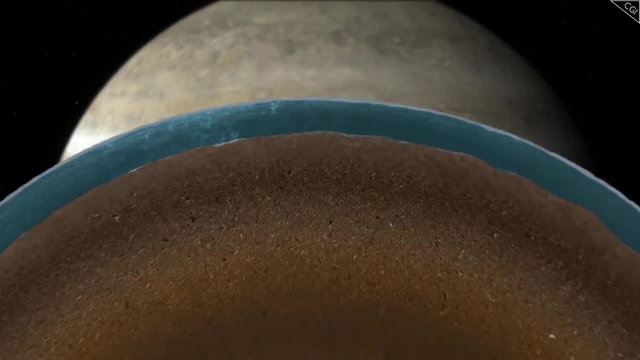 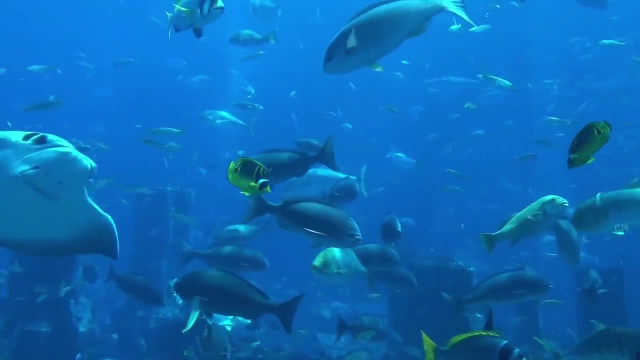 it may contain twice as much water as all of Earth's oceans combined. The most interesting about Europa's ocean is that scientists believe that it is in contact with Europa's silicate rocky mantle. This makes Europa's ocean a suitable environment for life as we know it to exist. 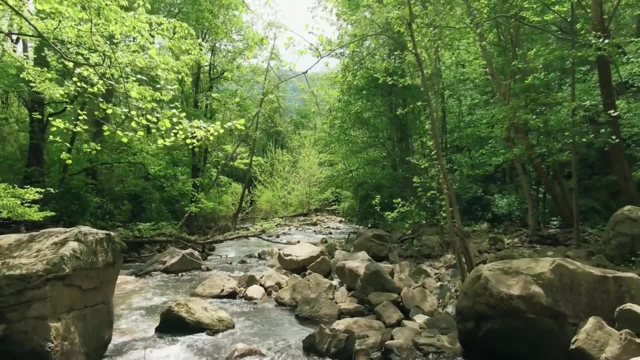 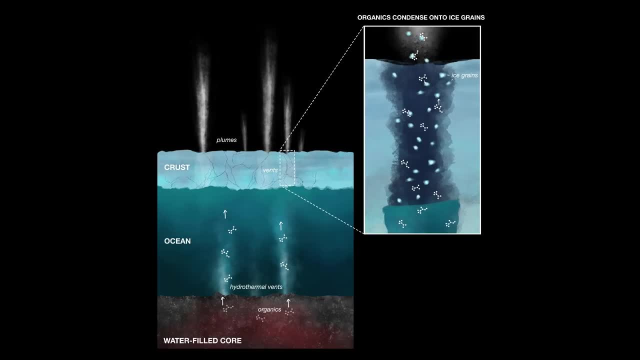 We believe that life requires water, minerals and energy to form, and Europa seems to have all these requirements. From the evidence we've seen so far, scientists are extremely confident that this ocean not only exists, but that chemical reactions can take place there. 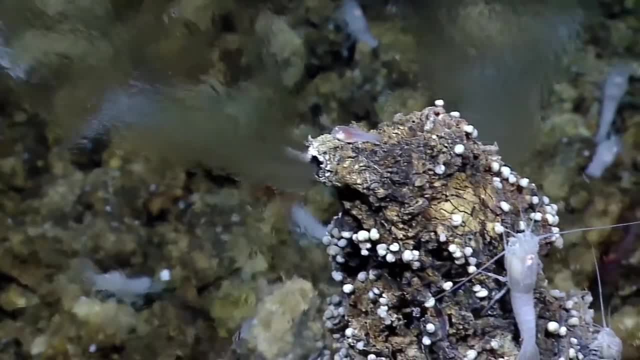 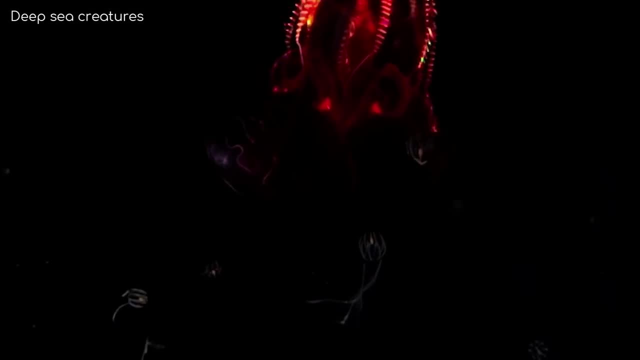 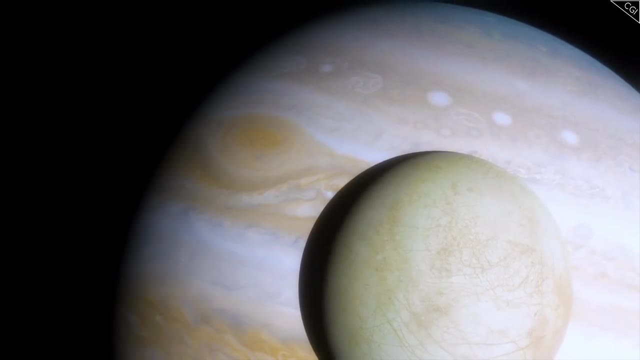 We also believe that there is enough tidal energy heating the core, that geothermal activity may exist on this ocean's floor. As we have seen on Earth, whole ecosystems can exist in such places, far from the sun's light. So for now, Europa is one of the most likely places we can find life outside of Earth. 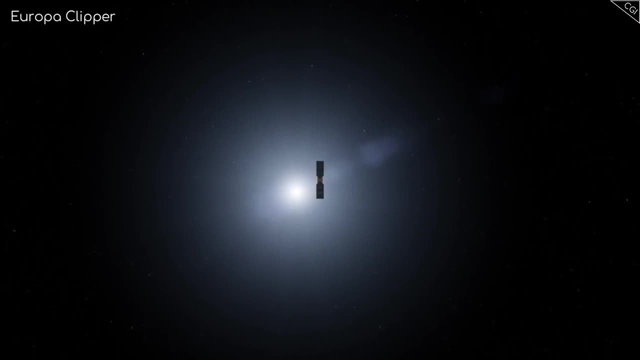 Now NASA's Europa Clipper spacecraft is scheduled to launch in 2022, and is likely to reach the Moon by the end of the decade. It is scheduled to perform more than 4,000 times its capacity. It is also likely to reach the Moon by the end of the decade. 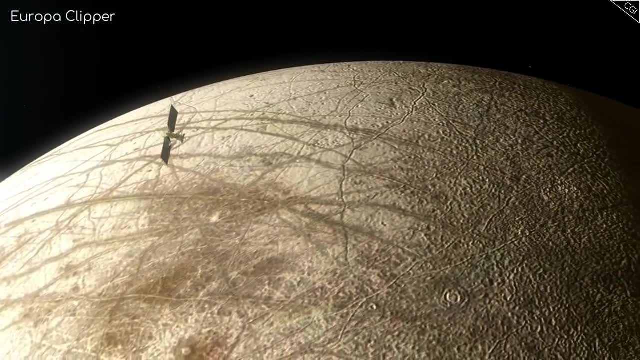 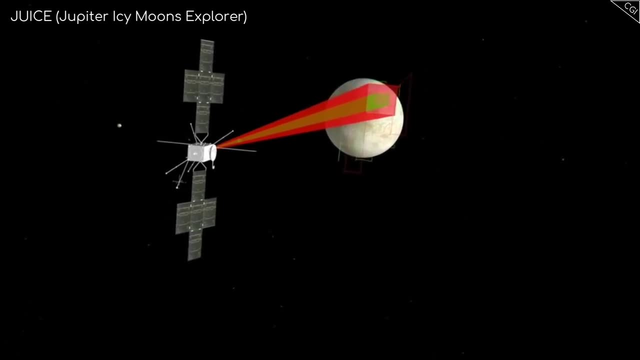 It is scheduled to perform more than 4,000 times its capacity. It is also likely to reach the Moon by the end of the decade. It is also likely to reach the Moon by the end of the decade. NASA will also be working on their own spacecraft called JUICE or Jupiter Icy Moons Explorer. 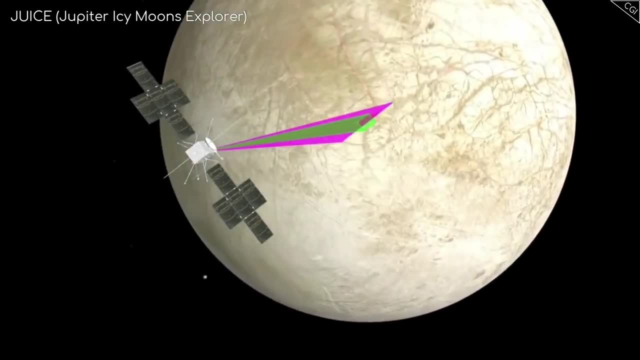 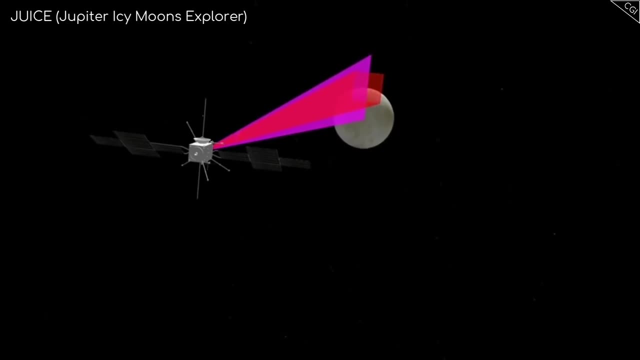 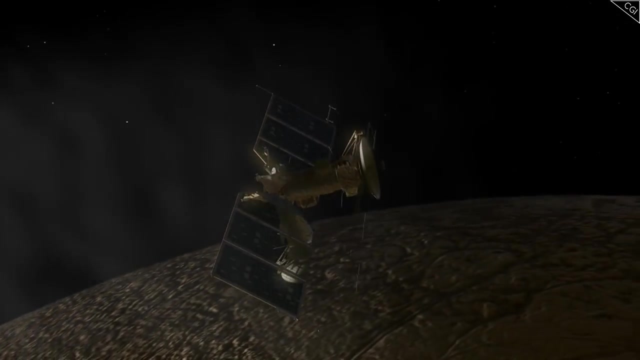 which will explore Jupiter and three of its largest moons: Ganymede, Callisto and Europa. JUICE is also scheduled to launch in 2022, and is also likely to reach the moon by the end of the decade. These probes are specifically designed to examine Europa's water plumes and atmosphere. 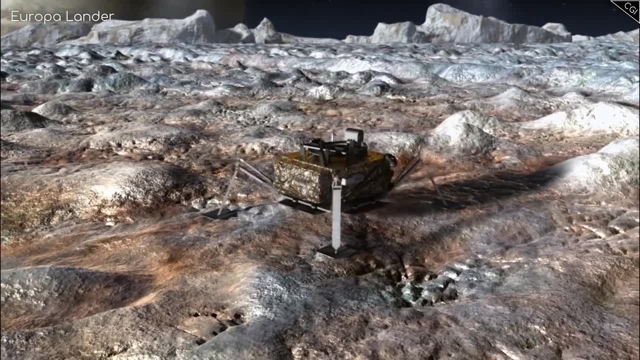 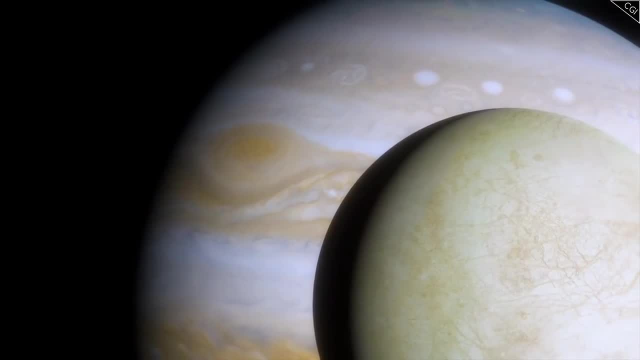 NASA is also planning a podemata probe, which is an image of the moon itself, a Europa lander mission, but this mission is going to launch well after the Europa Clipper mission. These missions will help us know more about Europa and hopefully confirm the answer. 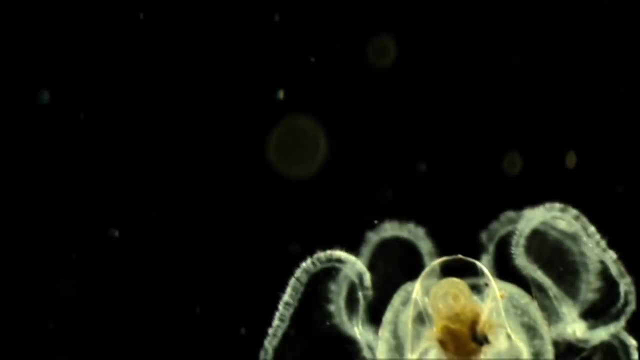 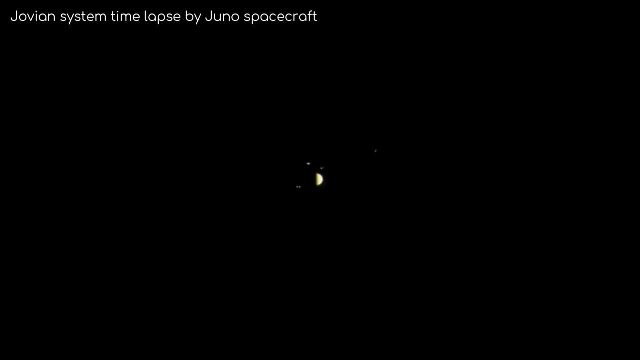 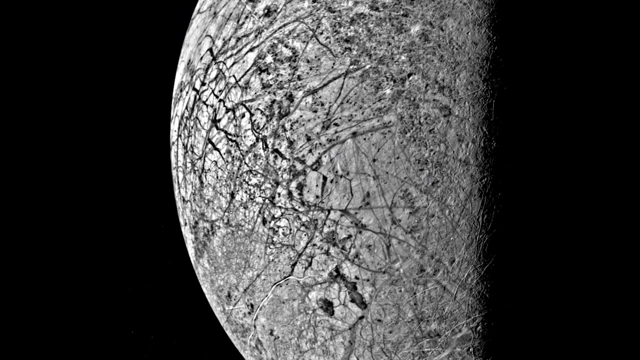 to the most tantalising question of all: does it and can it sustain life? At the very least, these missions will give us a new perspective of our solar system and help us understand how it works. So there we have it: almost everything you could want to know about the fascinating world of. 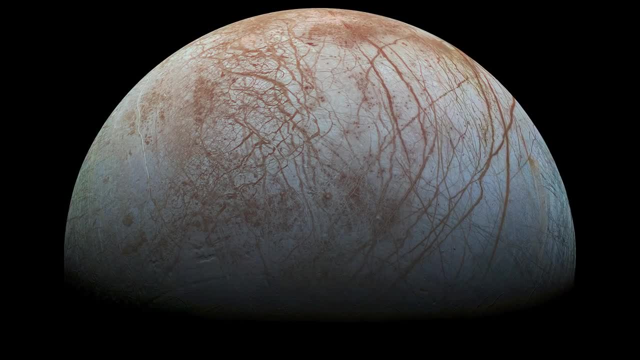 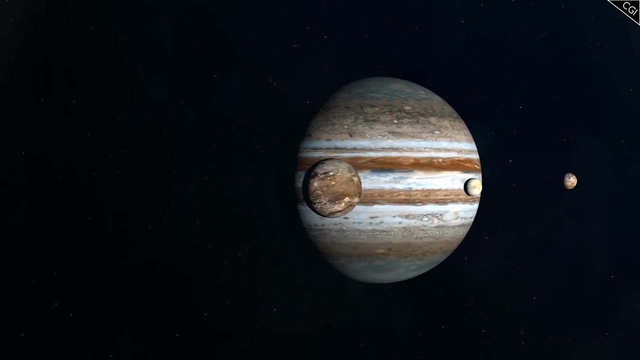 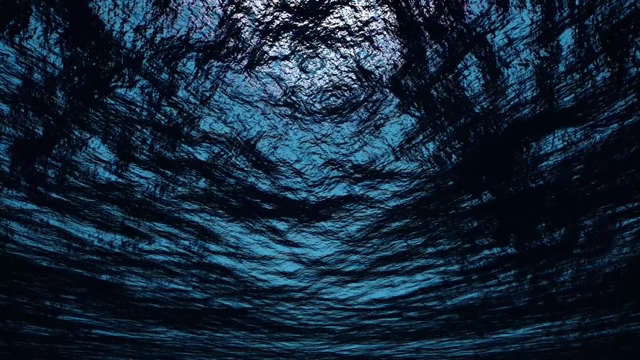 Europa. Ganymede, The third of Jupiter's Galilean moons, The largest moon that we know of and home to the largest water ocean in the solar system. But there's something else that sets Ganymede apart from anything else we've seen before. 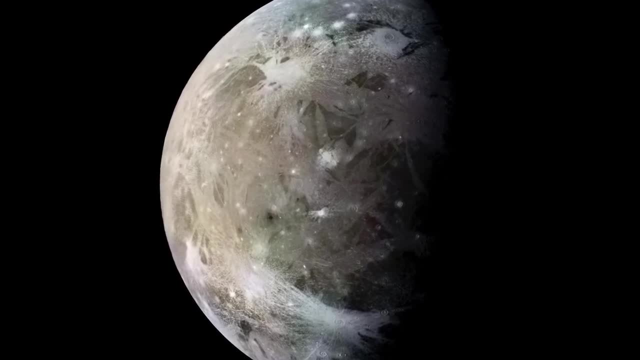 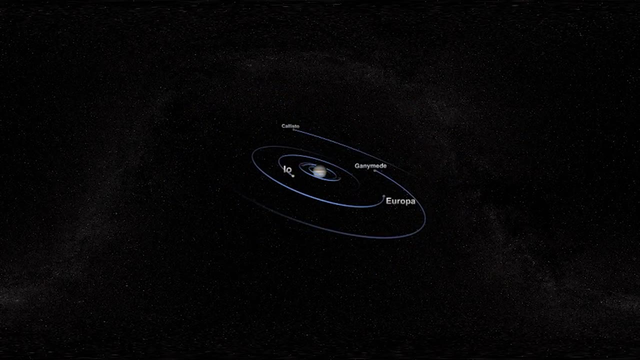 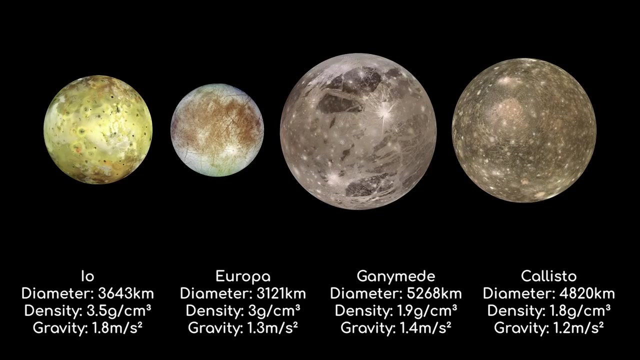 This Jovian giant contains an intriguing mystery buried deep beneath its surface. There are 79 different moons of Jupiter, and Ganymede is the third of a group known as the Galilean moons. Ganymede is the largest of these four, with an impressive diameter of 5268km. 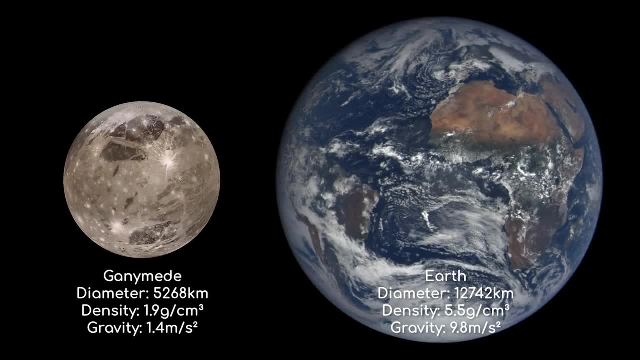 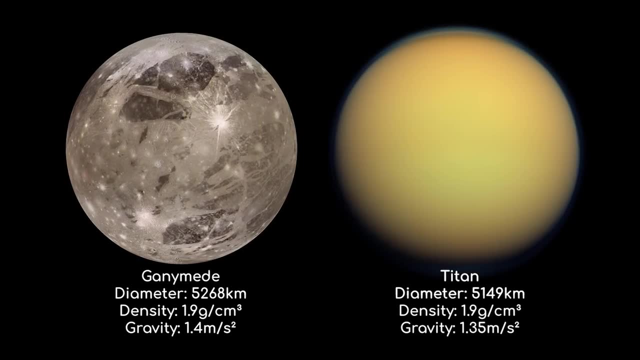 For a point of comparison, this is 0.41 times the size of Earth's diameter and 1.02 times greater than the previously thought to be largest moon, Titan. It initially appeared bigger because of its thick atmosphere, which stretches higher than the Earth's diameter. But Ganymede is the third of. 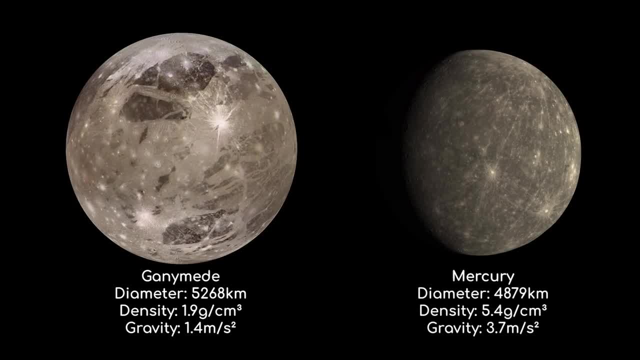 hundreds of kilometres into space. Ganymede's volume is even 26% larger than Mercury's, although it doesn't contain as much mass. Ganymede's average density is 1.9g per cm3, compared to Mercury's 5.4.. This is because of its composition. 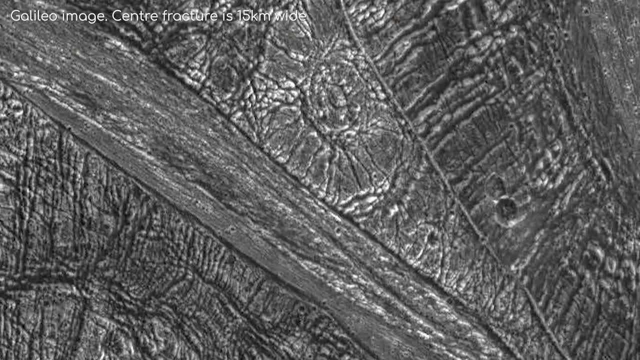 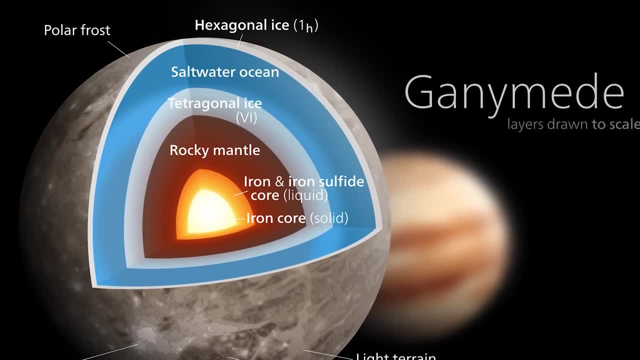 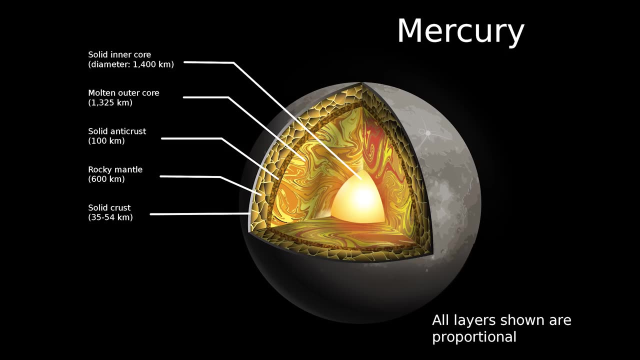 Like Europa, Ganymede's surface is a thick crust of water ice extending 150km deep, underneath which is believed to lie a vast ocean of liquid water. When I say vast, it really is, Because, while Mercury has very little water and is rich in 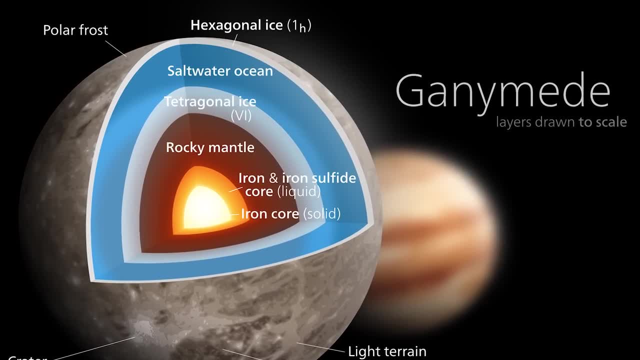 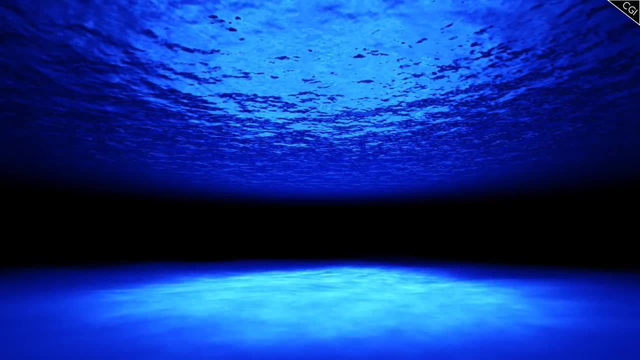 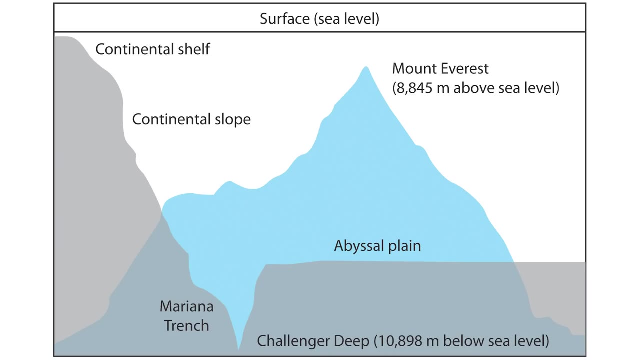 dense metals. the abundance of water on Ganymede reduces its average density. The ocean of Ganymede is so big that it contains more water than all the oceans and seas on Earth, and it is estimated to be 100km in depth, on average, 10 times deeper than the deepest point in our ocean. All of this water? 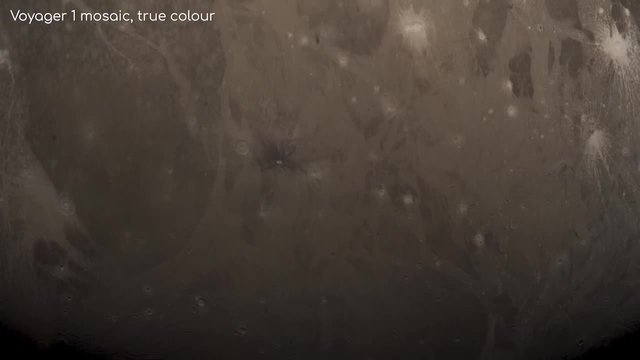 means that Ganymede is only 50% of the ocean's density. Ganymede is the third of hundreds of the oceans on Earth and is the second largest ocean in the world. This means that Ganymede is only 50% rock, the rest being water and small amounts of metals and other ices. 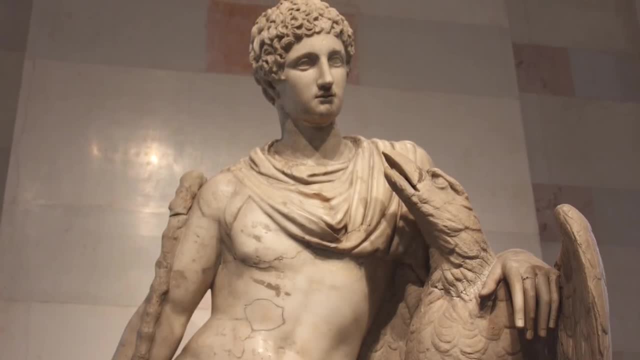 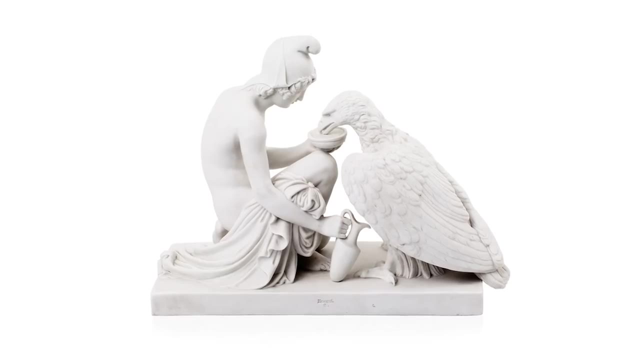 This seems appropriate to me, as the name Ganymede comes from the classical mythology, where Zeus or, as the Romans called him, Jupiter, claimed a young boy called Ganymede and took him to be a cupbearer for the gods. It seems fitting that the moon Ganymede would 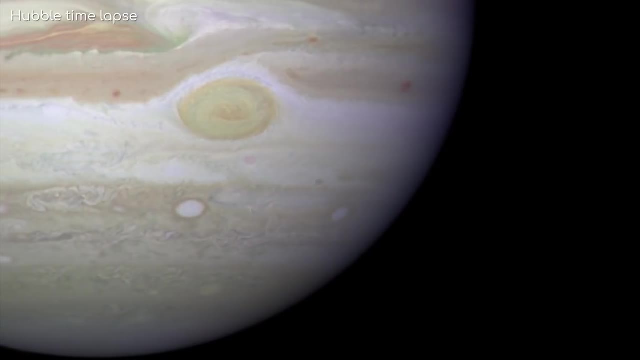 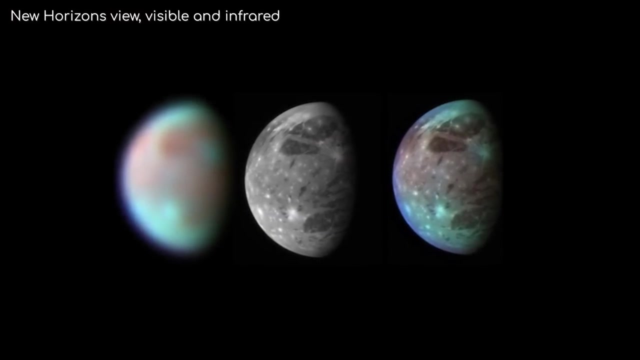 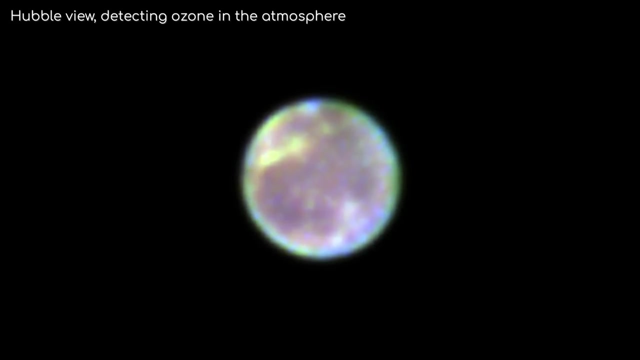 also carry so much water around for Jupiter. Interestingly, Ganymede has an atmosphere that contains oxygen. Now you might be wondering: with all the water in the world, what is Ganymede? Is it possible that life exists on Ganymede? While it's certainly possible, there are some. 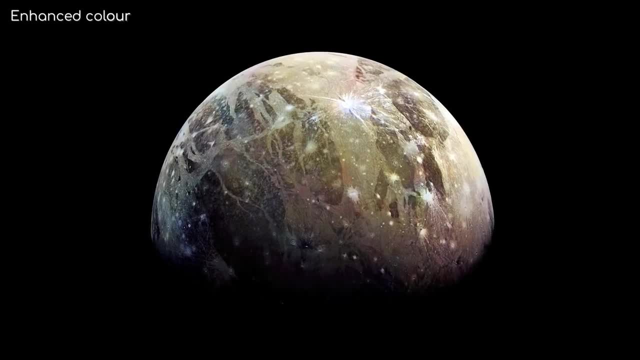 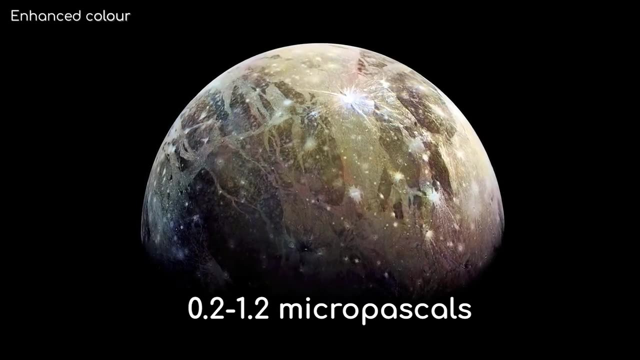 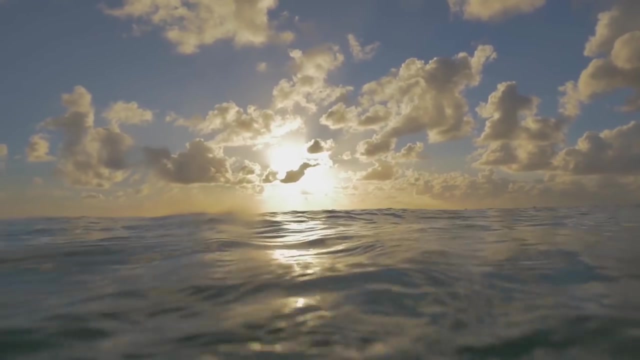 features of Ganymede that make this unlikely To begin with. the oxygen atmosphere is very thin. It is estimated to be somewhere between 0.2-1.2uPa, or about 100 billion to 500 billion times less than Earth's atmospheric pressure at sea level. That would be impossible to breathe, And 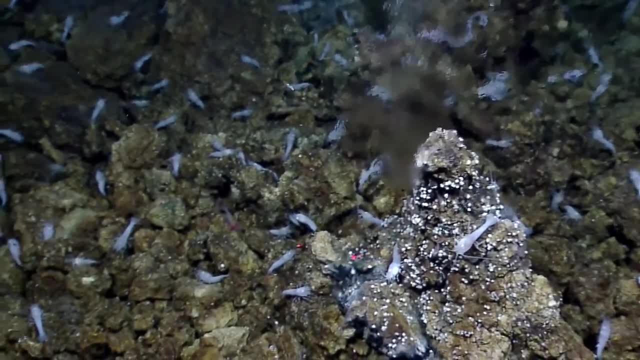 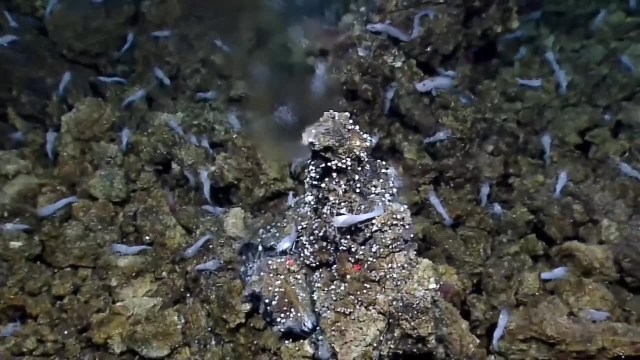 while the atmosphere is so thin? what is Ganymede? The atmosphere is very thin, It is estimated to be. While our own planet Earth has certainly demonstrated that ecosystems can flourish in the depths of oceans without sunlight to sustain it, there could be a big problem that prevents 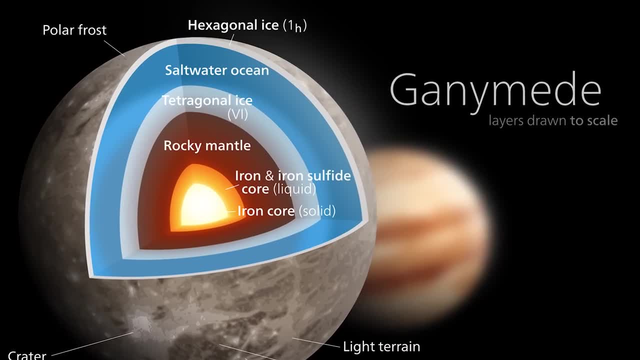 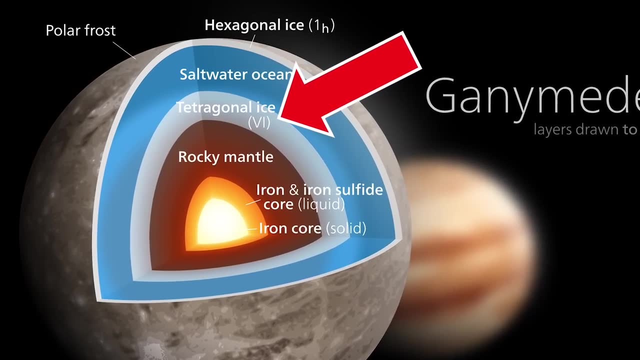 this from happening on Ganymede. This is because the ocean of Ganymede is so deep that water down at its bottom would likely be compressed back into an ice through sheer pressure. Life in the deepest parts of our ocean can survive thanks to minerals being ejected from. 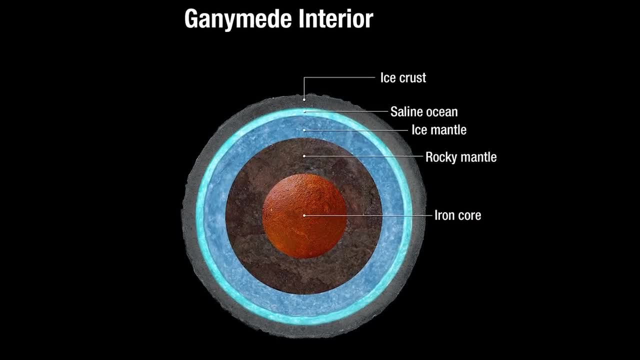 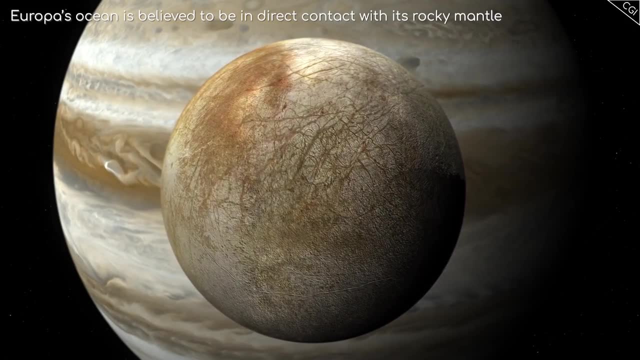 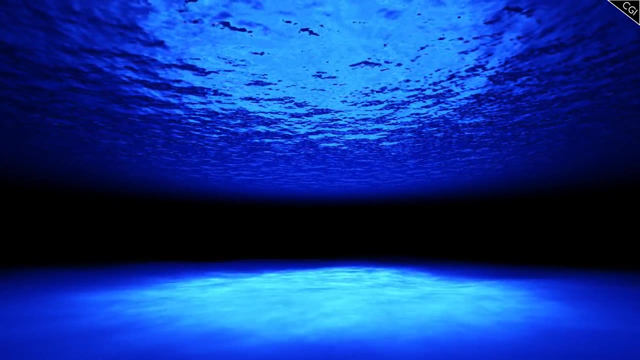 geothermal vents. With such a thick ice layer between the core and the ocean, it is unlikely that this would occur on Ganymede. Europa, Ganymede's neighbouring moon is considered a more likely candidate for life because of this. However, if Ganymede's ocean is salty, which there is an increasing amount of evidence, 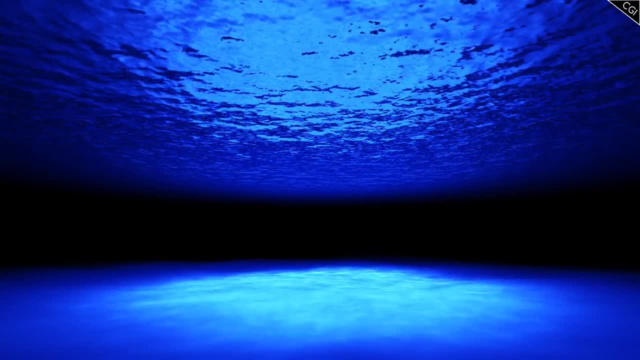 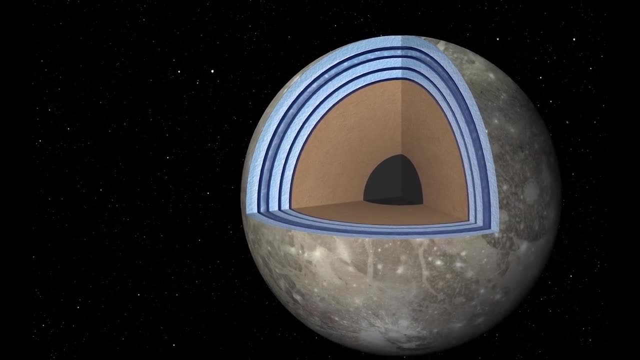 for it could change the interior make-up of Ganymede drastically. Models suggest that, with a salty ocean, it could be that there are multiple layers divided by sheets of ice. If this is the case, the most internal layer could indeed be in contact with the rocky. 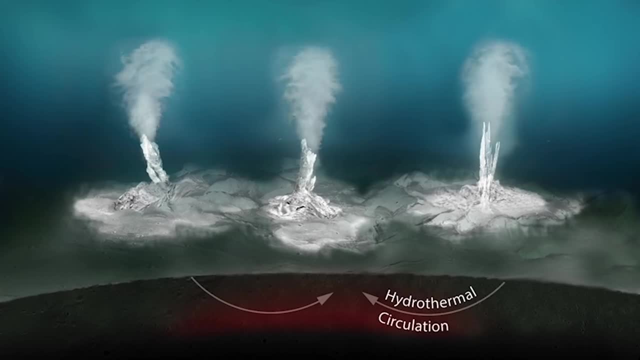 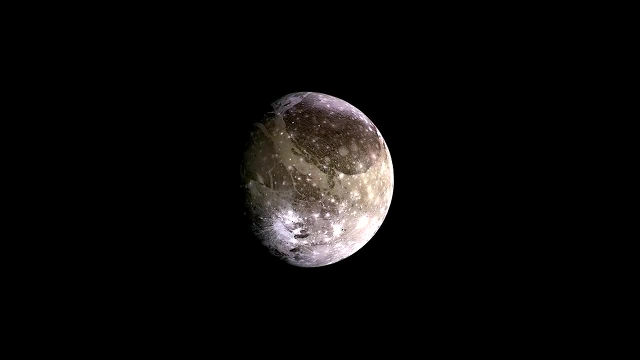 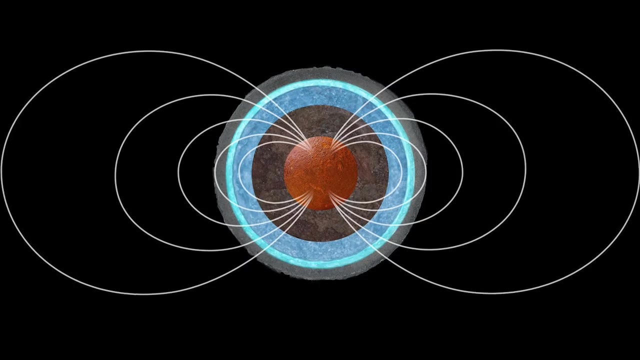 core, increasing the chances of life existing there. But underneath Ganymede's ice and water exists something else truly surprising, something that scientists do not have an explanation for. Somehow Ganymede is producing a magnetic field. The magnetic field of Ganymede was first discovered by scientists in 1996, when the Galileo Space 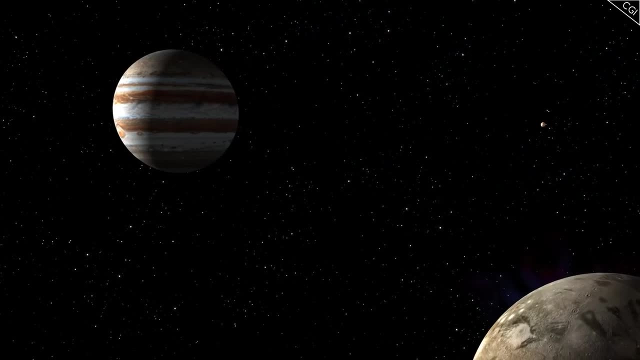 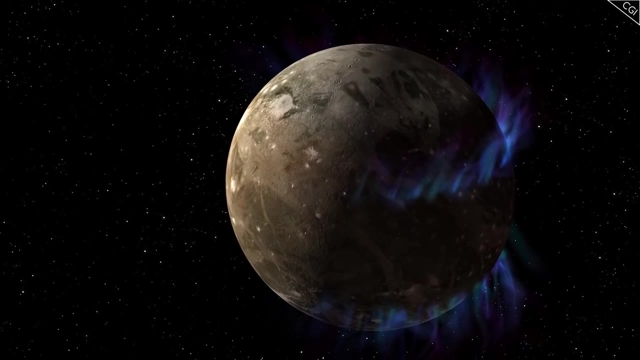 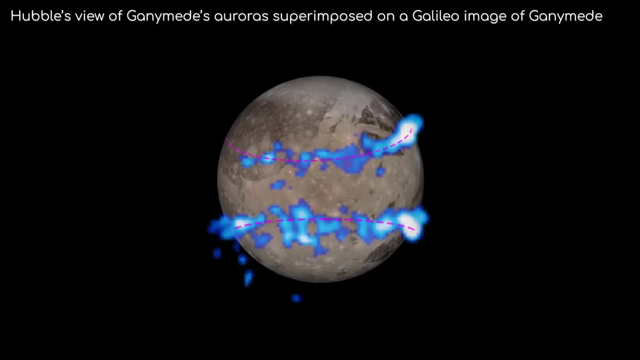 craft began a series of flybys of the icy moon. The big indicator of a magnetic field is the presence of auroras and, incredibly, auroras were detected in Ganymede's tenuous atmosphere. Not only that, but as Hubble studied Ganymede over an extended period, it became clear that 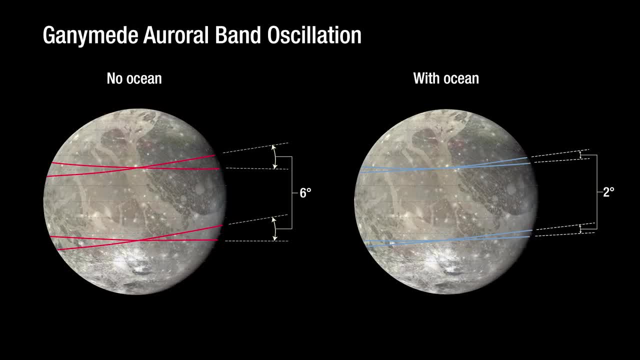 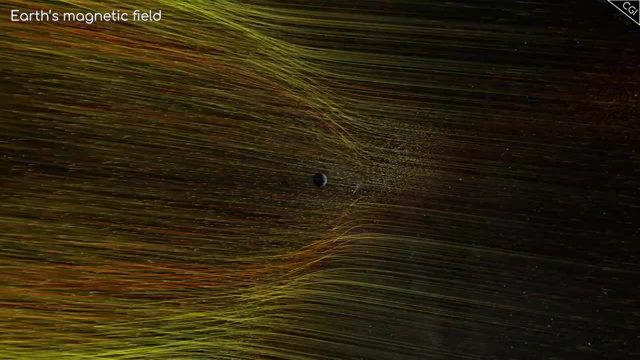 these auroras didn't wobble as much as expected, likely a result of something known as magnetic friction in a salty water ocean under the surface. A magnetic field is significant As it's the feature on Earth that shelters the planet from solar radiation, enabling 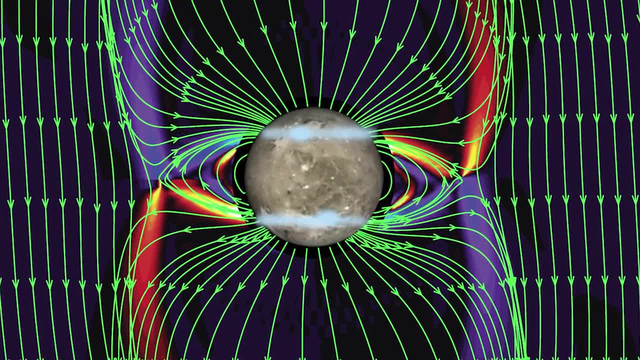 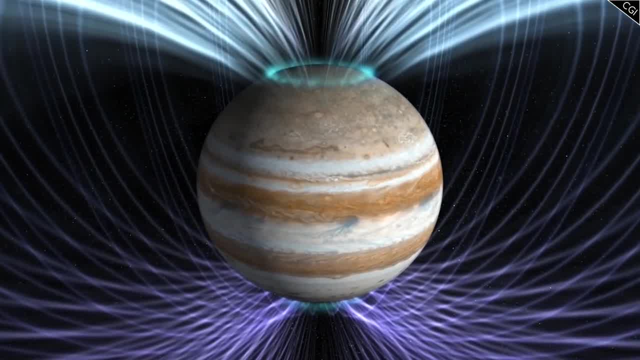 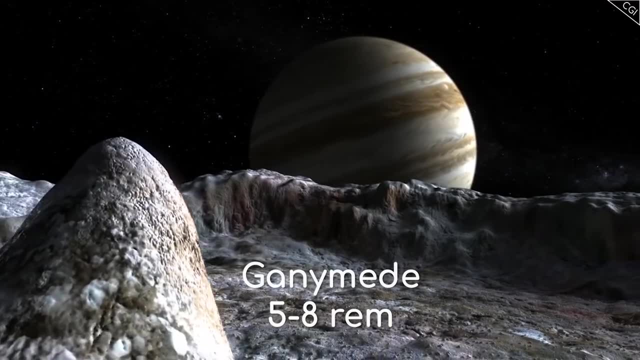 all life to flourish. The field around Ganymede does not completely protect it from such radiation. Being tucked within Jupiter's incredibly powerful magnetic field and radiation belt means it's still getting pelted with a lot of radiation. Ganymede's surface still has about 5-8 rem- enough to make a human severely ill or dead. 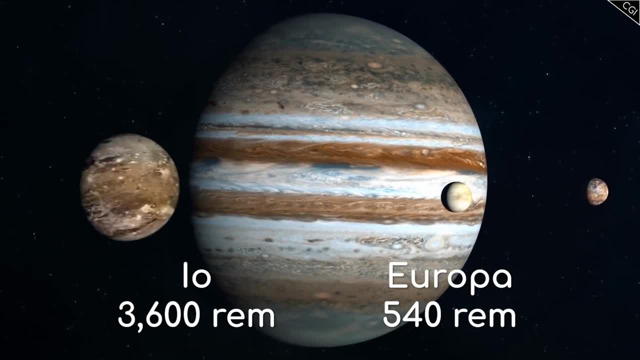 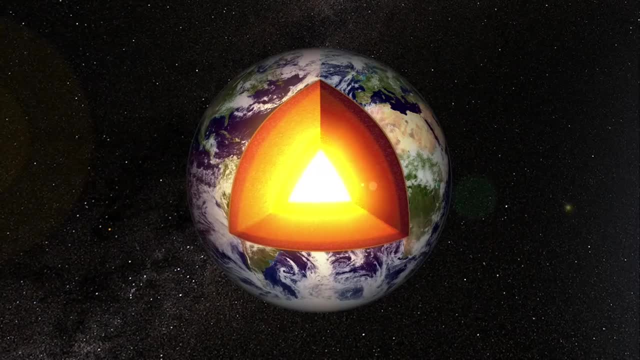 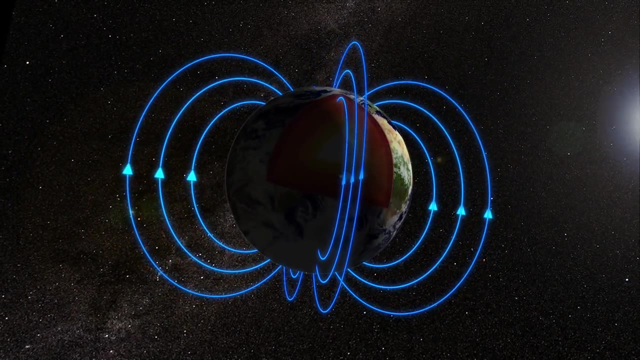 in just two months, But it's still better than its closer orbiting neighbours. Scientists are not quite sure why this magnetic field is here at all. Our planet's core is hot and molten. Convection currents within it move electrons, which in turn produces the magnetic field. 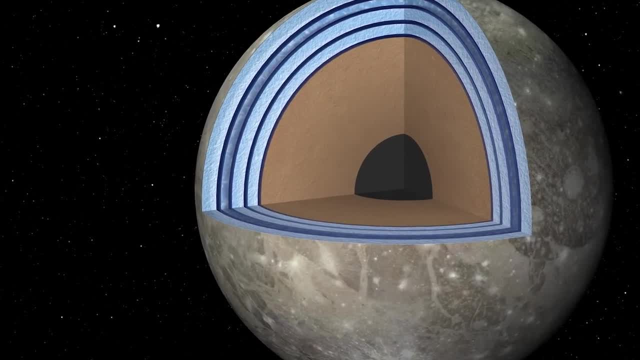 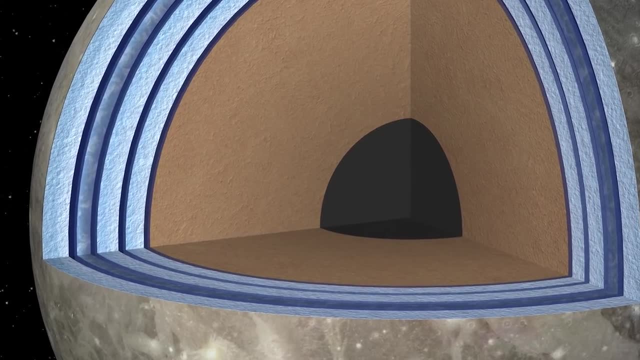 that surrounds us here. However, this shouldn't be happening on Ganymede. Ganymede is smaller than Earth and, given its size and composition, scientists believe that the core should have cooled down enough by now that it should be a solid mass, not. 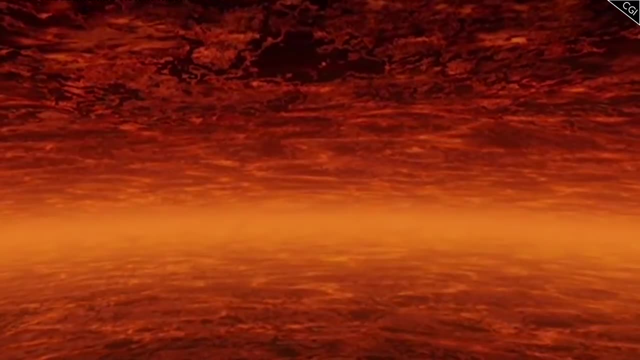 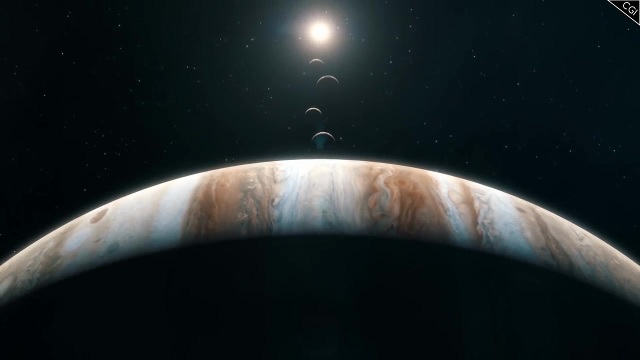 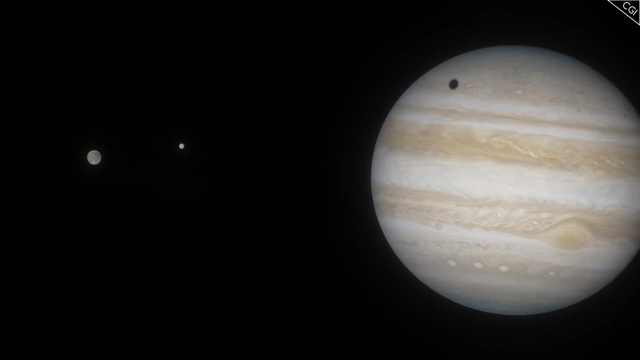 liquid. This would prevent electrons moving through convection and would prevent a magnetic field, And none of the other moons of Jupiter have a magnetic field. In fact, Ganymede is the only moon in the entire solar system that has one. So what's going on? 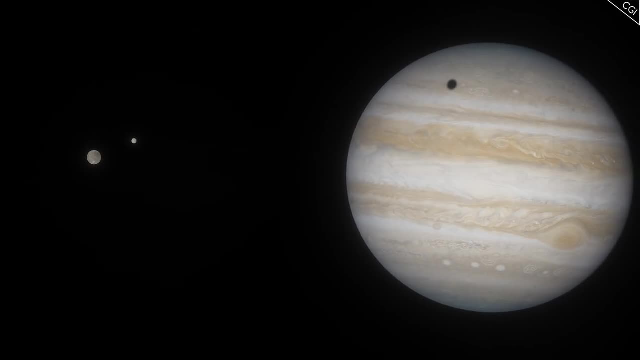 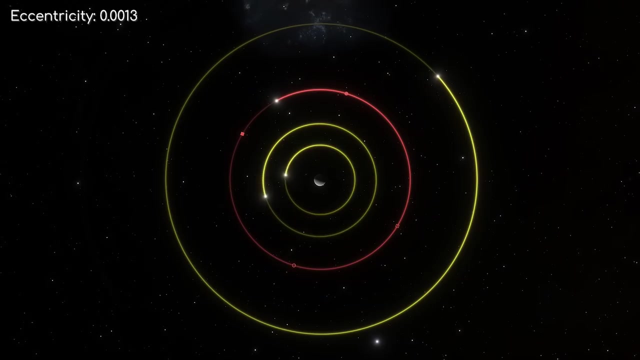 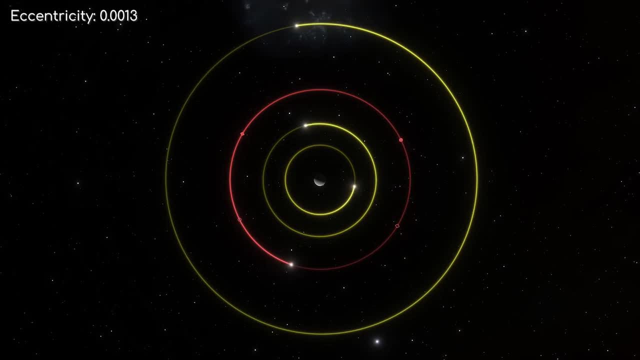 Ganymede orbits around Jupiter roughly once every seven days in an exoplanet. Ganymede orbits around Jupiter roughly once every seven days in an exoplanet. This means that at some points of its orbit it's closer to Jupiter than at others. 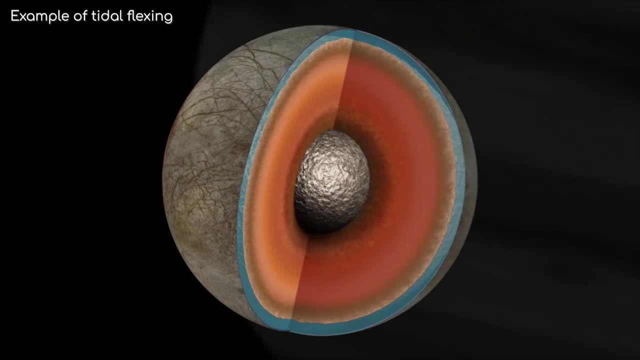 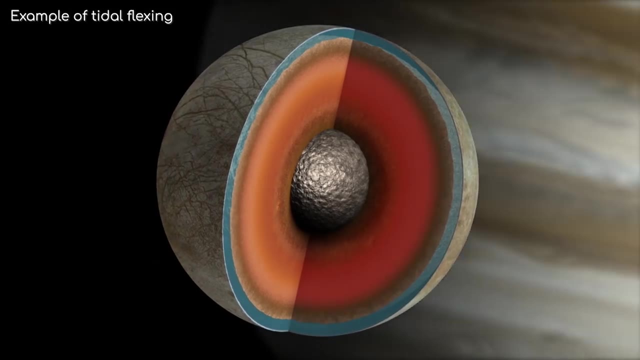 When an object comes under a strong gravitational force, it will stretch in the direction of that force, as mass is pulled in the direction of gravity. However, the further an object gets from the source of gravity, the more it will compress back to its original shape. 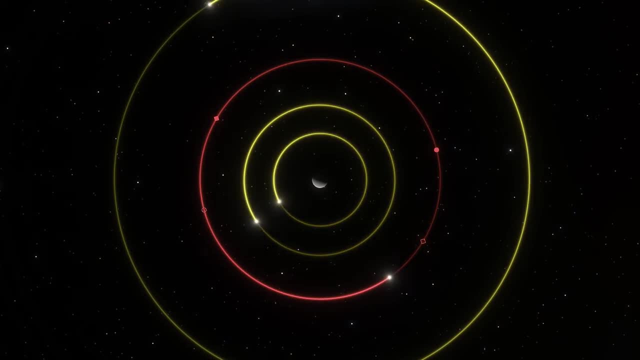 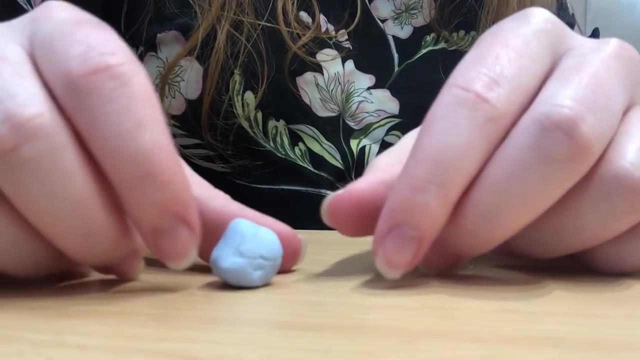 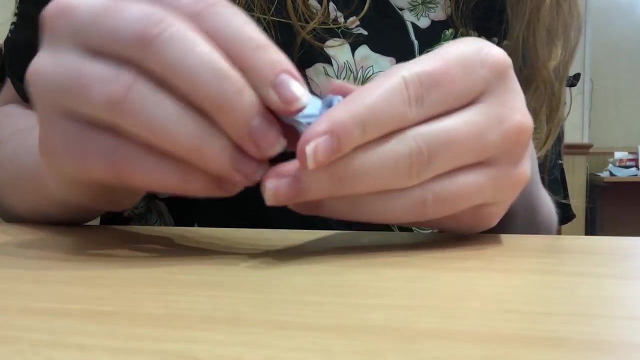 As Ganymede has an eccentric orbit around Jupiter, it is constantly coming under more and then less gravity And is constantly stretching and contracting. Have you ever pulled and stretched blue tack repeatedly in your hands before pushing it back to a ball shape? Then you might have noticed that after a while it gets surprisingly warm. 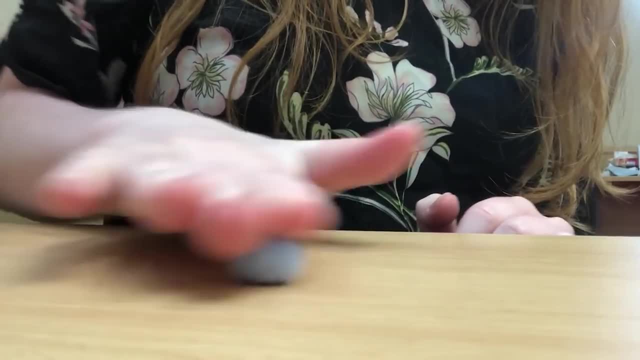 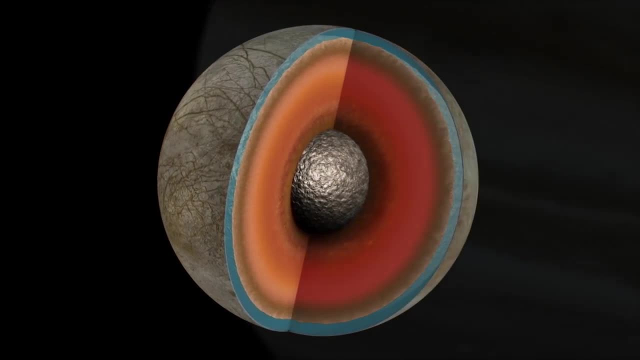 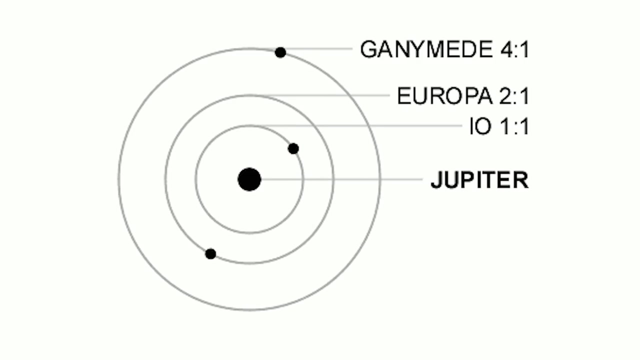 This is because stretching produces friction as the material rubs up against itself, And on the scale of moons and planets, this friction adds up A tidal force. creating heat through friction is known as tidal heating. On top of that, In a process I find fascinating, Ganymede has formed an orbital resonance with two of 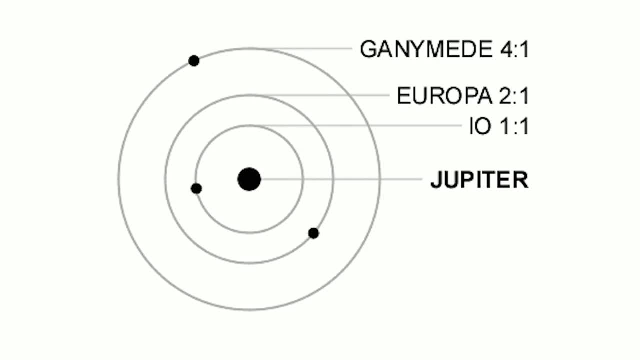 its fellow Galilean moons, Io and Europa, in what is called a Laplace resonance. For each time Ganymede orbits Jupiter, Europa will orbit exactly twice and Io exactly four times. This mathematically precise configuration has not happened by coincidence, but is evidence. 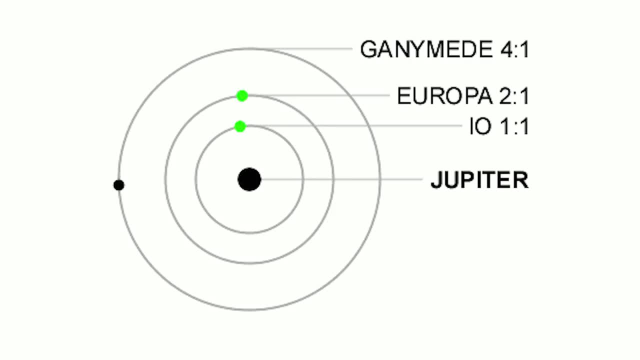 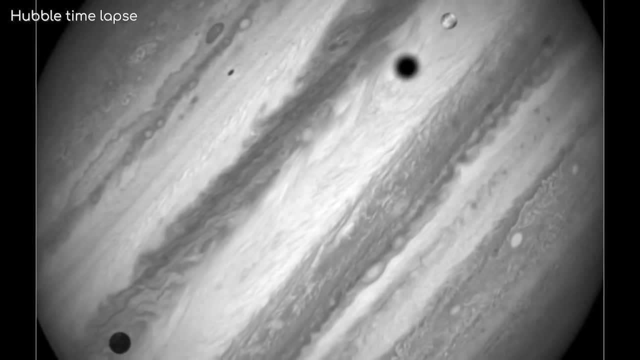 of the moons' gravities pulling on each other and the whole system attempting to conserve the resulting momentum. However, it's not a coincidence. However, it means that Ganymede is constantly being pulled by its neighbour's gravity and is under a lot of gravitational stress. 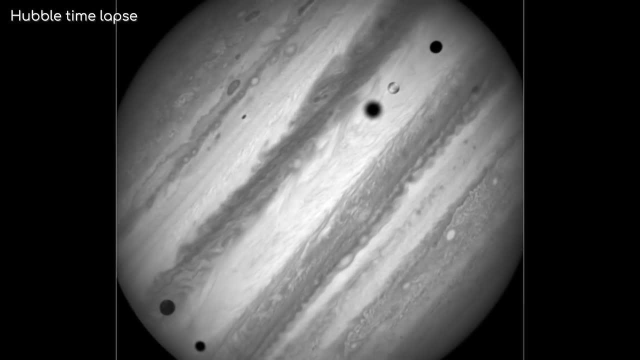 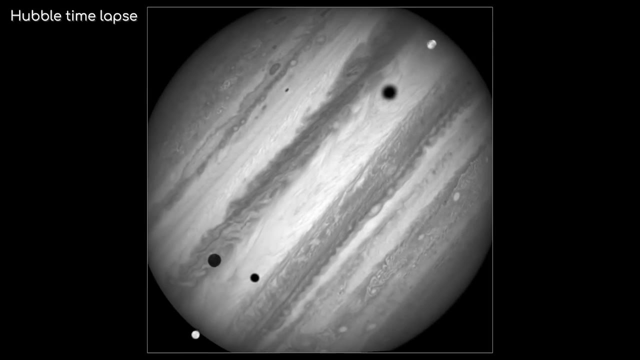 So perhaps tidal heating is warming up Ganymede enough that its core remains a liquid after all, helping it to continue to produce its magnetic field. Scientists do not know for sure, but it would perhaps explain why the surface of Ganymede is so interesting. 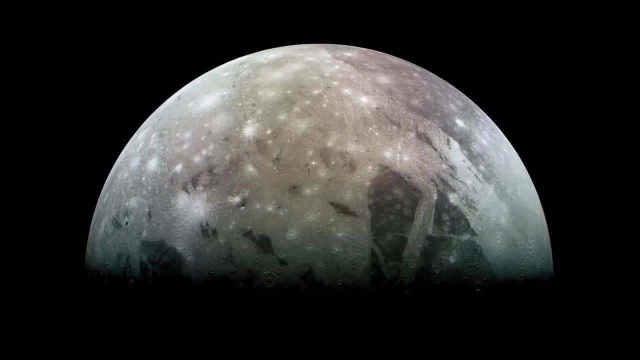 You may have noticed that Ganymede's surface is split into large dark regions that cover about a third of its surface. However, Ganymede is not a magnet. It is a medium-sized dark region that is also filled with light- up to a third of its surface. 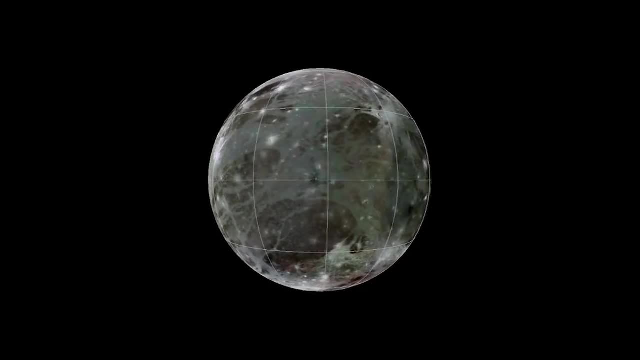 and there is a higher chance of it being a magnet, as it is actually light up to a third of its surface, And it is the same for the rest of the surface. If the surface of Ganymede is dark, Ganymede is light and it is light meaning Ganymede. 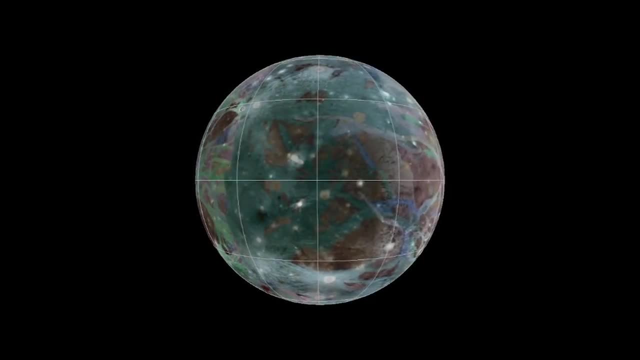 is light. The lightest regions are the ones that make up the other two thirds. Through examining the number of impact craters on these two sections, scientists can tell that the dark regions are actually older than the lighter ones, as they contain more craters. 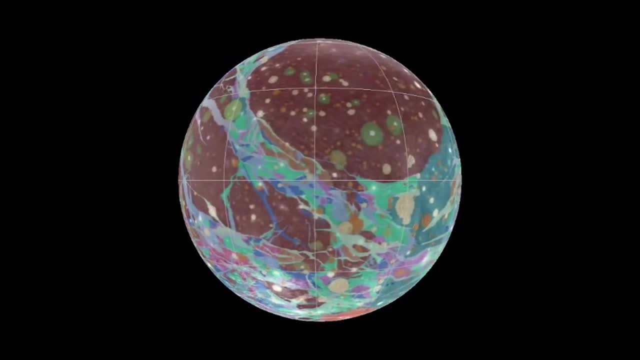 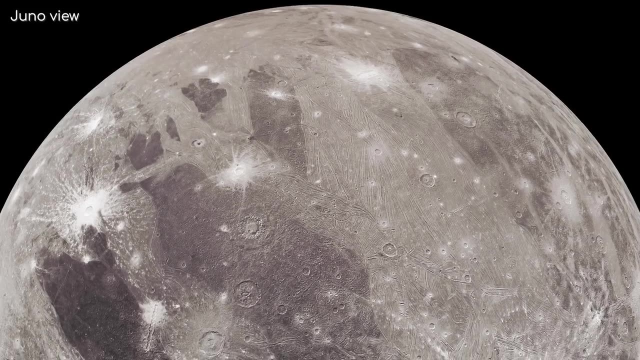 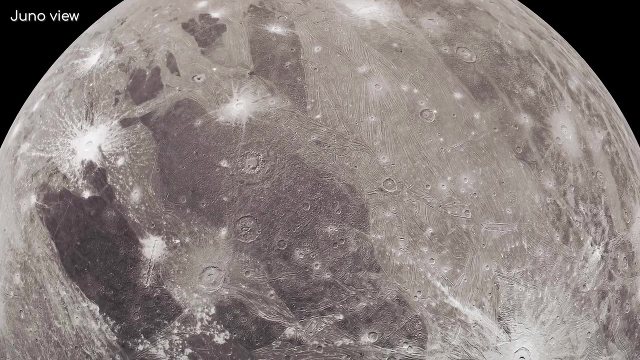 The lighter regions might have fewer craters, but they do contain long ridges and grooves, up to 700m high and thousands of kilometres long. Truly an impressive sight. But again, scientists are not sure how these ridges formed. One explanation is that tidal forces stretched out the surface of the moon in an unstable. 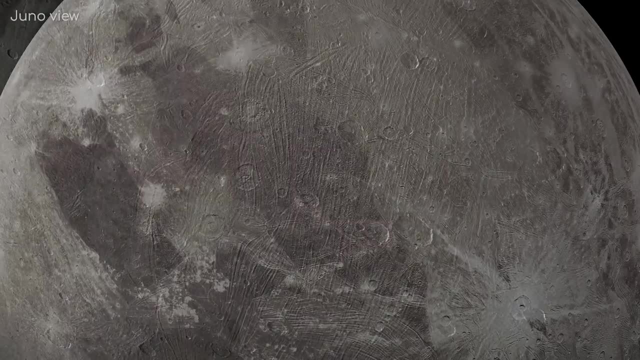 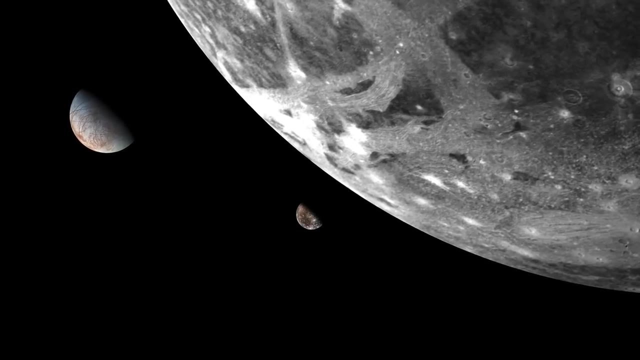 period of Ganymede's ancient history. Perhaps this same tidal force could have also warmed Ganymede's core and preserved its magnetic field. Whatever its cause, the magnetosphere of Ganymede has been instrumental in helping scientists understand the composition of the moon. 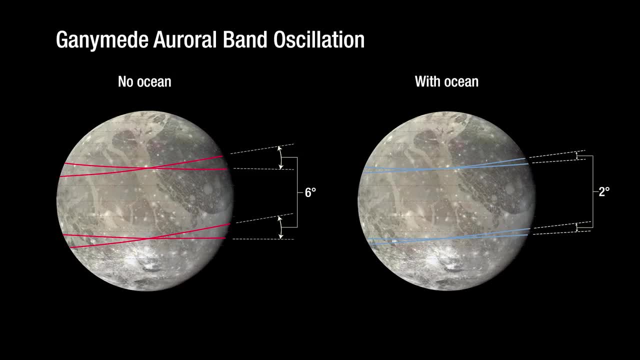 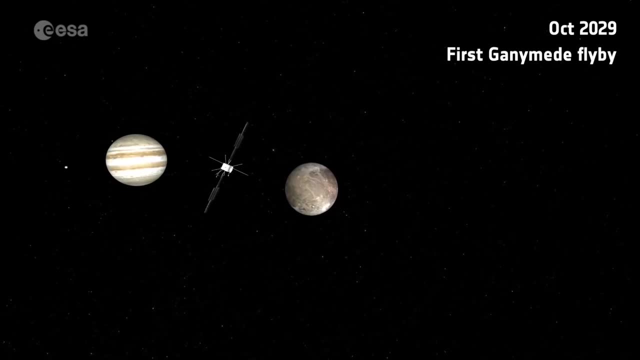 By measuring the areas that auroras appeared in Ganymede's atmosphere, scientists were able to confirm the existence of Ganymede's subsurface oceans, all without having set foot there. And as for the rest of Ganymede's mysteries, maybe JUICE, the Jupiter, Icy, Moon Explorer? 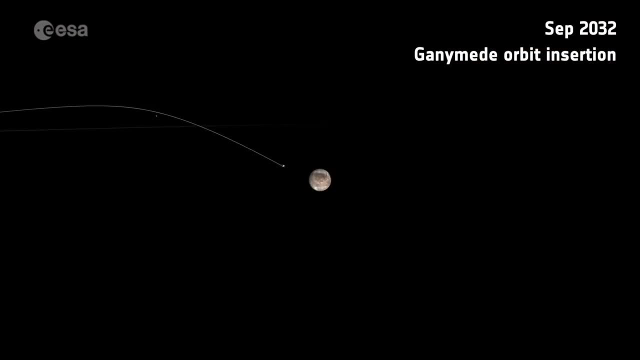 will find us the answers. The ESA spacecraft is set to launch in 2022, and, though it won't reach orbit around Ganymede for another 10 years after that, it's to investigate the inner workings of a number of Jupiter's moons, including Ganymede. 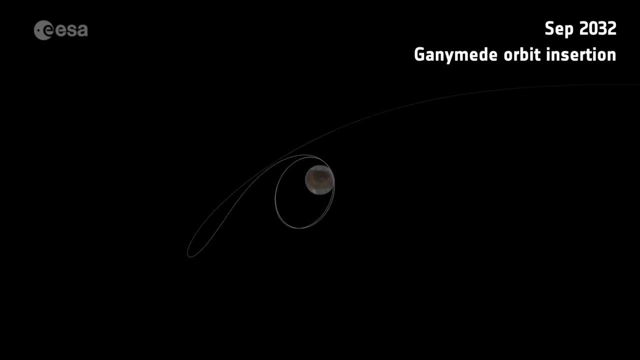 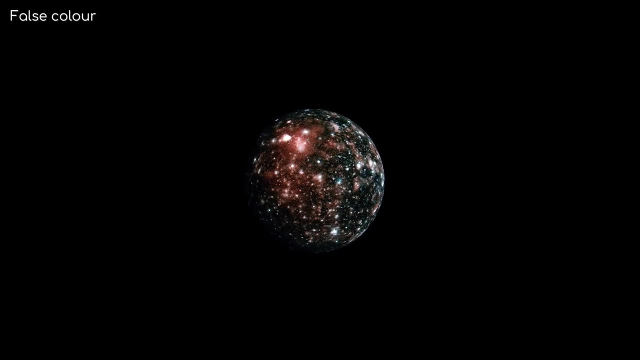 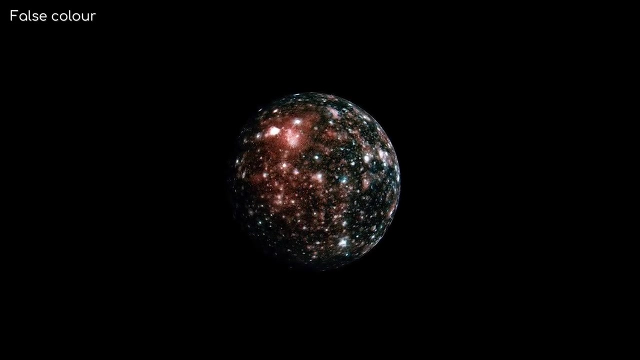 Until then, we may have to let Ganymede's mysteries remain just as they are: Just that: a mystery. Callisto. Despite the fact it is the third largest moon that we know of, I think the majority of people would be hard-pressed to say any facts about it at all. 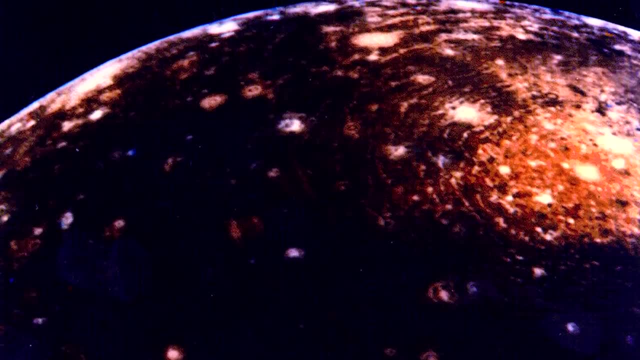 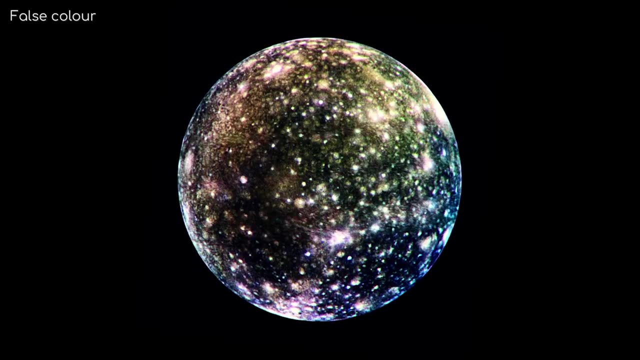 Is it just a boring world, or do we simply not know much about it? Actually, we know more than you may first assume, and it is far from boring. Let's start with the ESA. The ESA is the world's largest solar system. 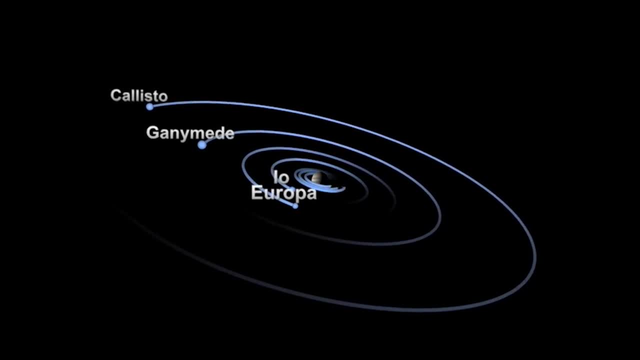 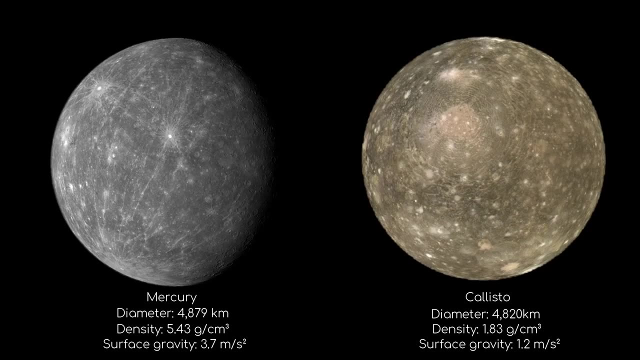 It is the world's largest solar system. Let's start with where it fits into the Jovian system. Callisto is the third largest moon in the entire solar system and it's just smaller than Mercury at 4,820km across. 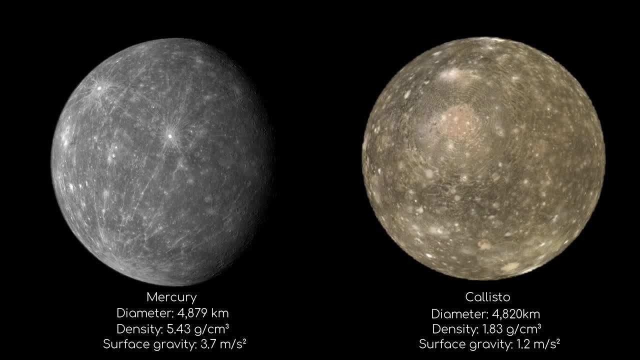 However, while its diameter is only 58km less than Mercury's, it is only one third of the mass of the planet, meaning it's less dense and its gravity is a lot weaker. It is the second largest of the Galilean moons and orbits Jupiter much further out than the 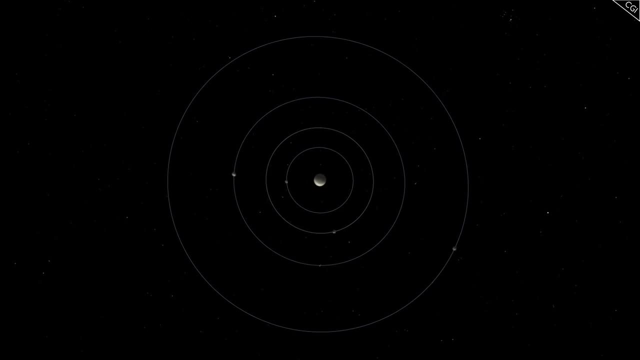 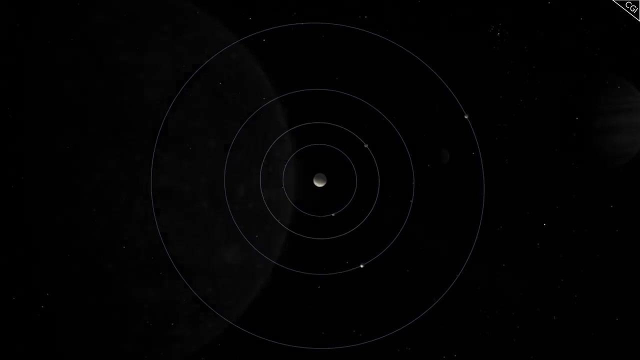 other three, Taking 17 Earth days to do so, at an average distance of 1.9 million km. Even at this distance, it is still tidally locked with Jupiter, meaning the same side of Callisto always faces its parent planet. 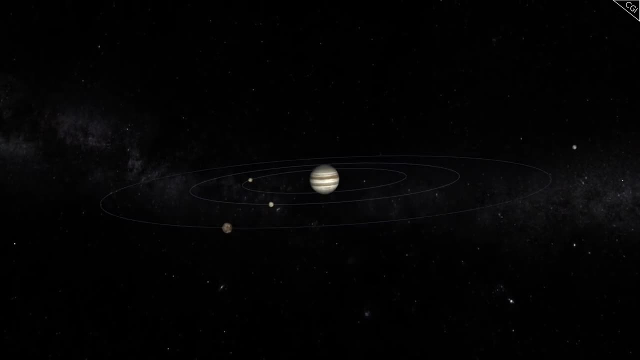 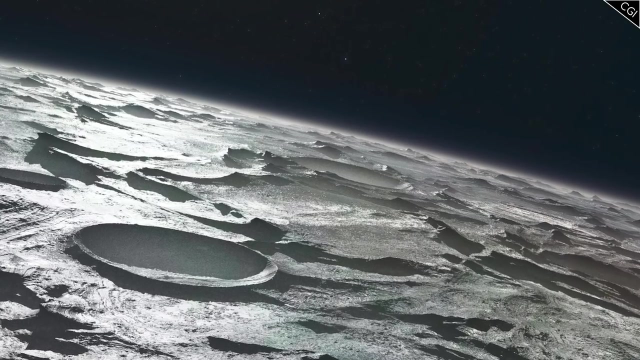 However, it does mean that it is not locked in an orbital resonance with the other three moons, nor do we believe that it ever was. Callisto has a very tenuous atmosphere composed of carbon dioxide and possibly oxygen too, although oxygen has not yet been released. 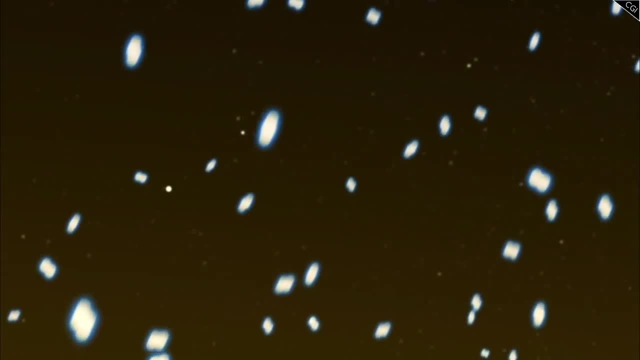 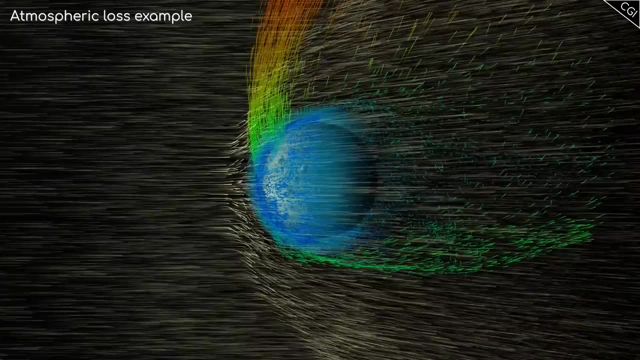 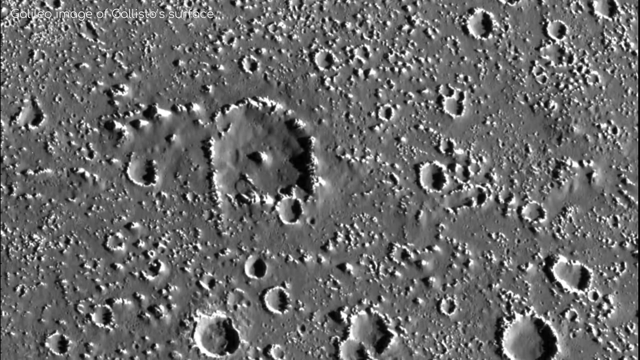 We know, however, that the atmosphere is so thin that the molecules contained within it do not collide and theoretically, the atmosphere should be stripped away by atmospheric loss processes in just four years. Scientists believe that Callisto's crust is replenishing the lost atmospheric particles. 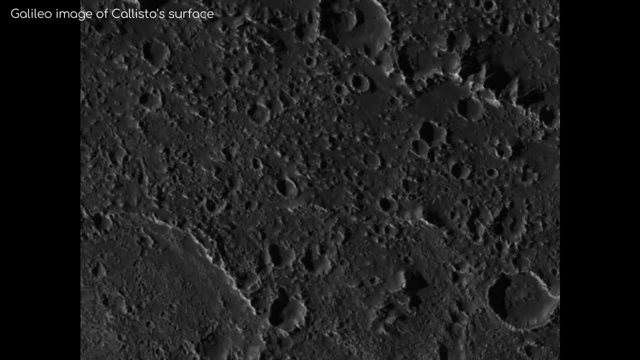 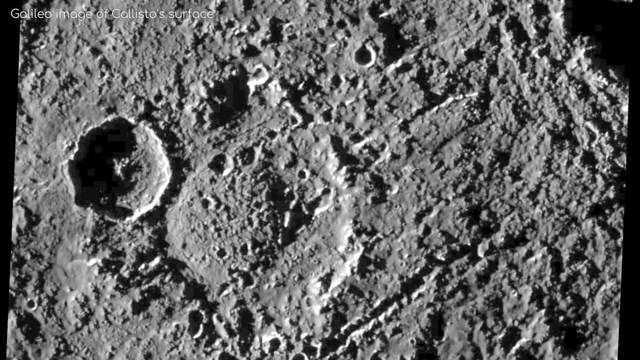 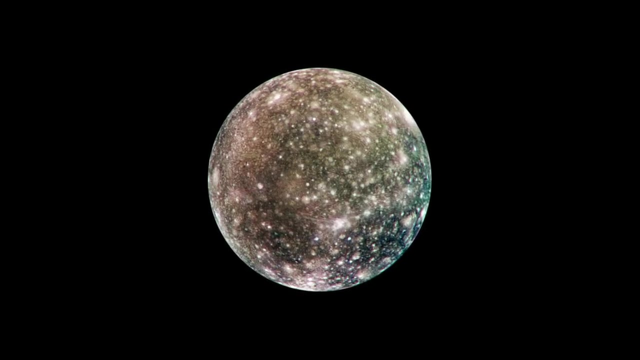 through sublimation of carbon dioxide surface ices evidenced by some interesting surface features. Now, the surface of Callisto is one of the most ancient in the solar system, with evidence placing it at over 4 billion years old. You'll immediately notice the speckled nature of Callisto. 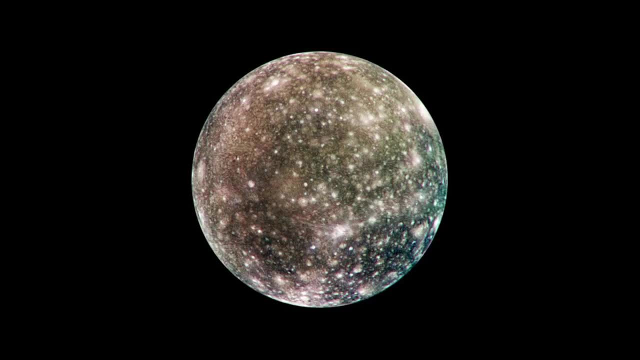 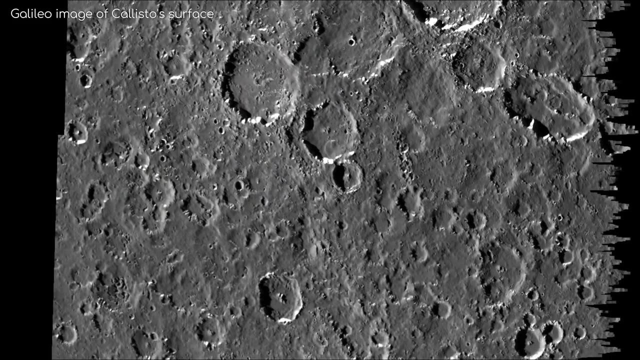 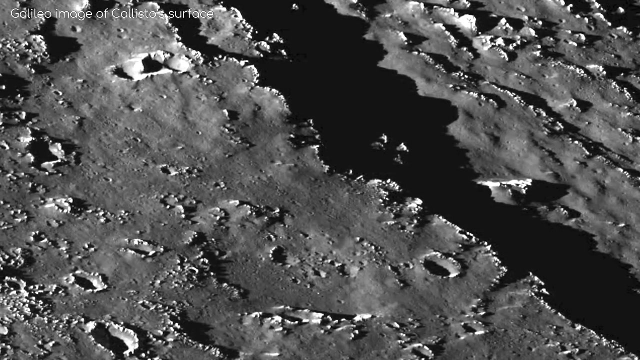 Its surface is completely covered with various sized impact craters, more so than any other object we've observed. In fact, it's close to saturation – any new crater will probably just overlap another one at this point, Without any geological activity. cratering is perhaps the only process that has vastly 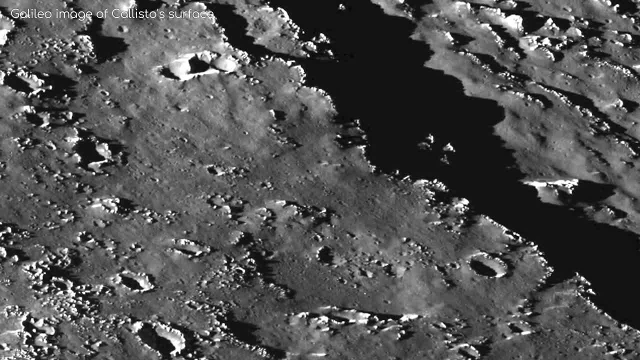 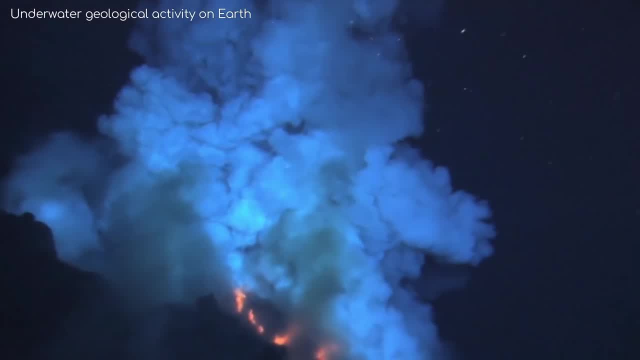 been impacting Callisto's atmosphere. Observe the surface's appearance over its lifetime. Why is Callisto's surface so old compared to a lot of other bodies in the solar system? Well, on geologically active planets like Earth, there are processes that can erase. 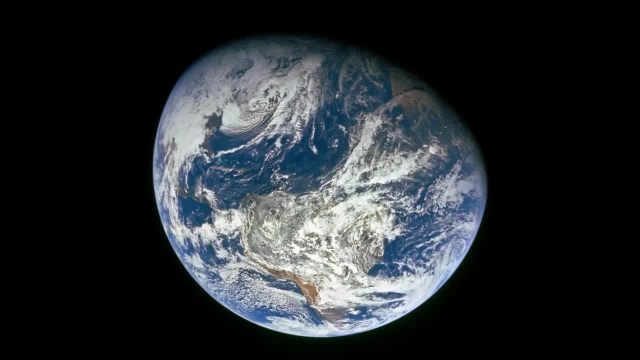 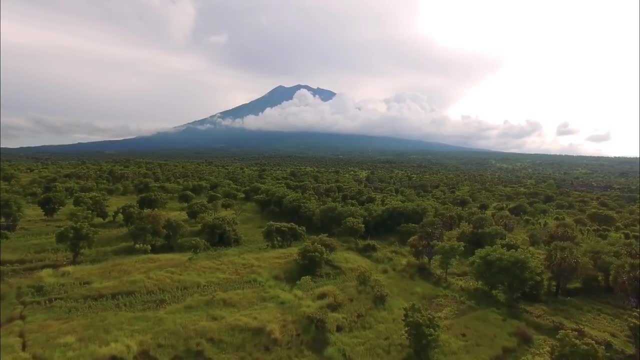 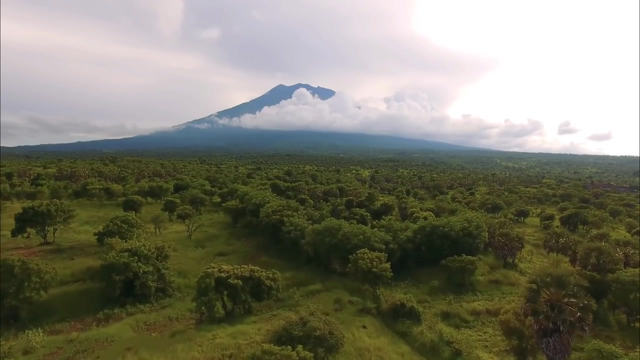 almost all evidence of past impacts. Earth has one of the least cratered surfaces in the solar system because so much happens on its surface – it has weather, water plants, volcanism, tectonic plates and human activity. These act together to break apart, wear down and lift up the ground. 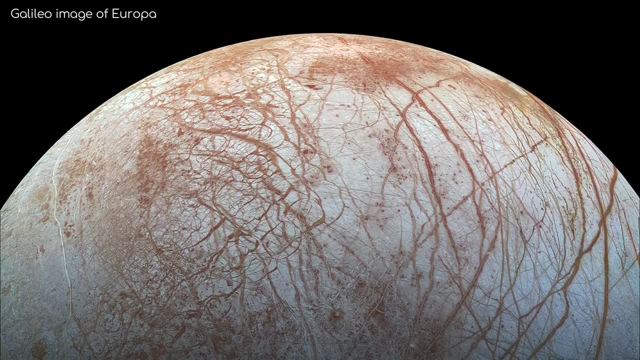 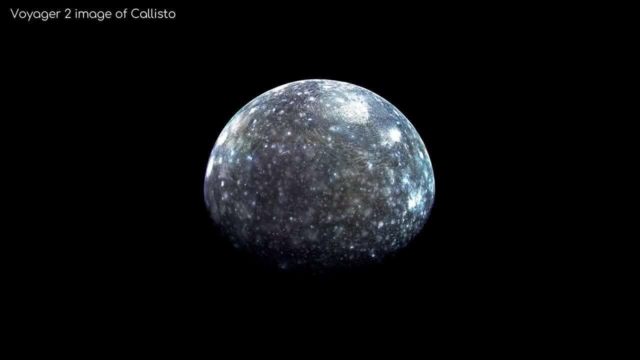 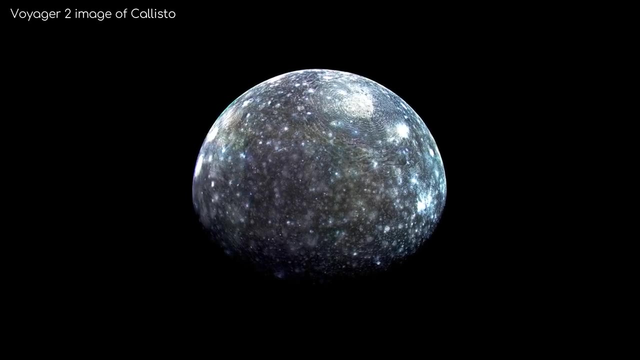 Even other Jovian moons like Europa or Io, have comparatively fewer craters thanks to tidal forces which cause geological activity on their surfaces. This doesn't happen with Callisto. Callisto does not show any signs of geological processes such as volcanism or plate tectonics. 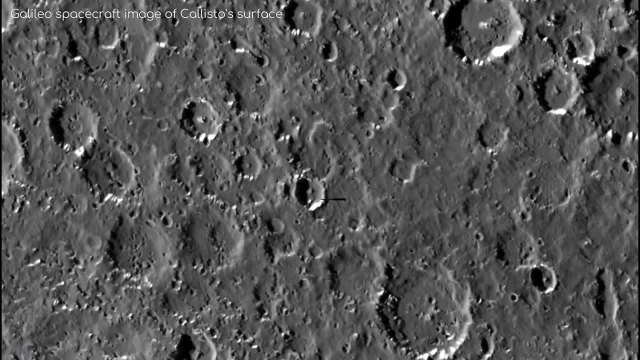 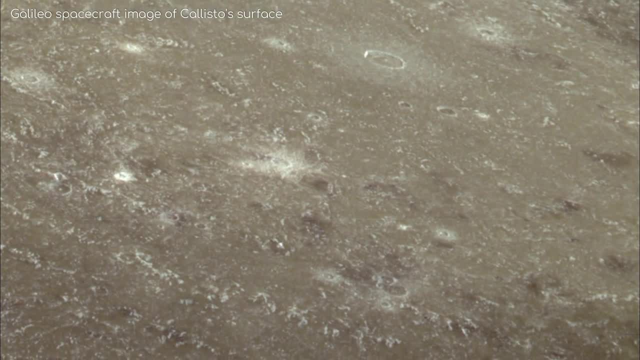 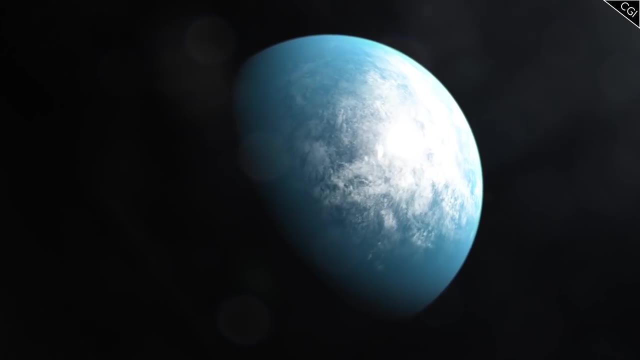 and so its surface has remained intact after all these years. Many tidal forces, and thus no geological activity, impact Callisto in another, very unique way – there are no mountains to speak of on its entire surface. When Callisto initially formed at the very beginning of the solar system, it was likely. 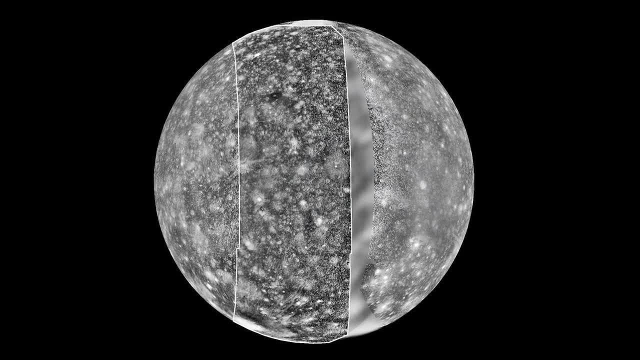 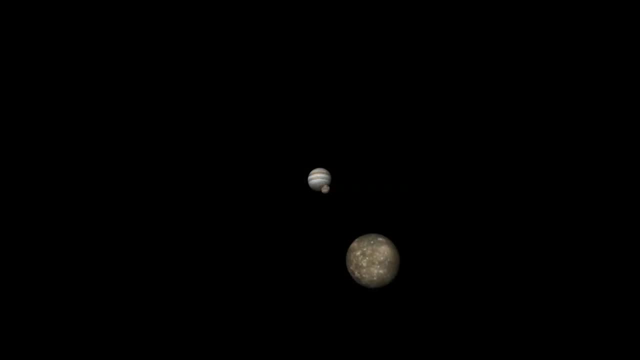 an ocean world that has since frozen over and, apart from the bombardment of meteors, it has stayed exactly the same ever since. So let's have a look at some of these craters, because some of the biggest are truly impressive. 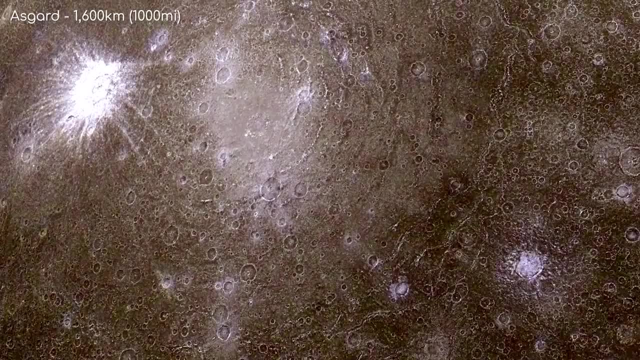 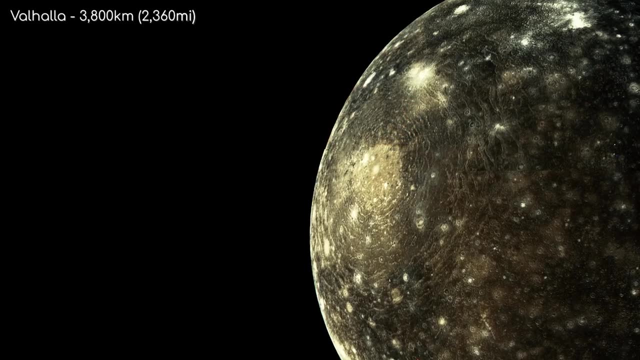 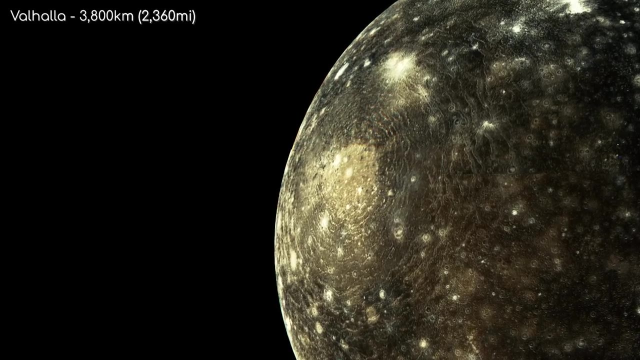 This is Asgard, the second largest impact crater on Callisto, measuring 1,600km in diameter, And this is Valhalla, the largest multi-ring impact crater in the entire solar system, with a diameter of 3,800km. 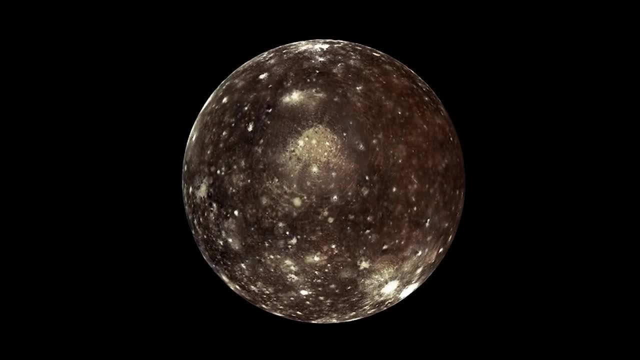 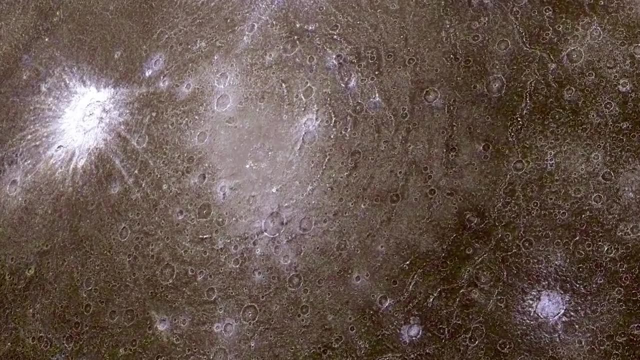 It's these craters that add to the unique appearance of Callisto, as they contain more rings than craters anywhere else. With these craters, the impactor was large enough that it made its way into the atmosphere way too quickly, have completely punctured the thin crust, with it eventually refreezing over in the 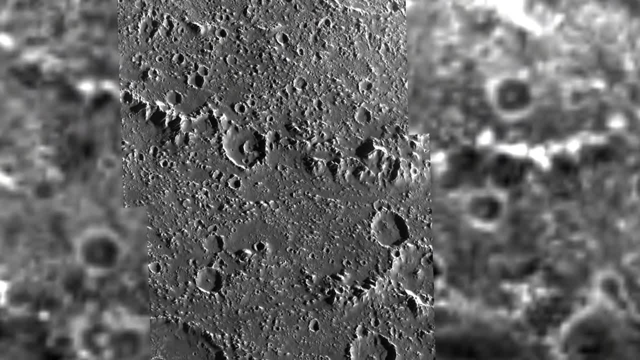 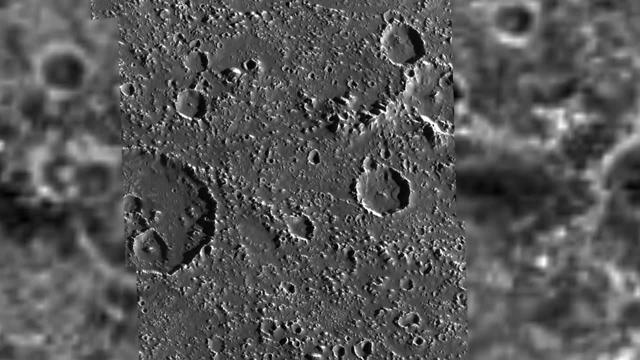 light patches you see in the middle. Zooming in on these middle regions, you'll notice they have a mottled appearance. There seems to be a big difference, in contrast, between the bright knobs and the darker plane. These regions are a lot less cratered than the rest of Callisto's surface, which would 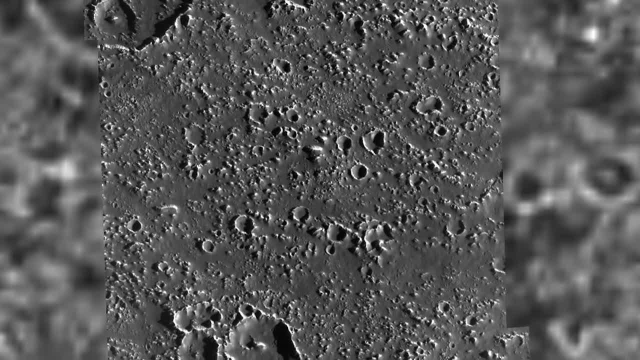 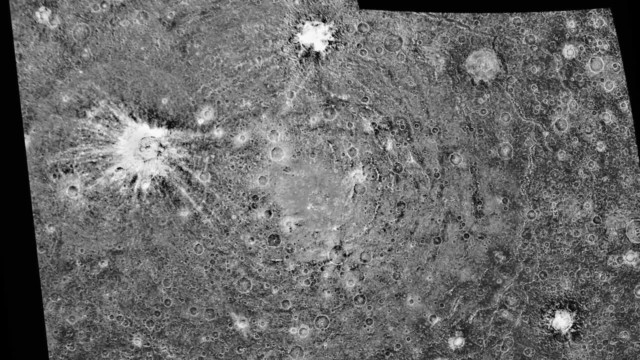 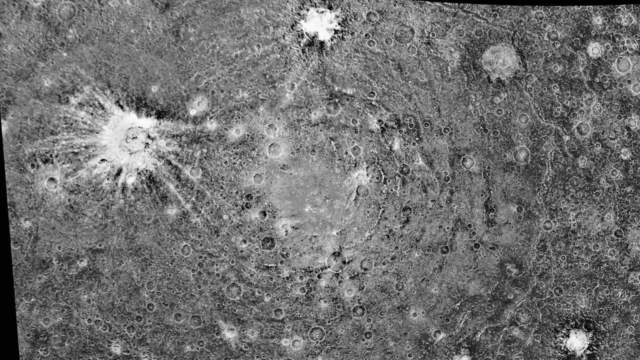 make sense if the plane truly is a refrozen surface, likely making it 2 billion years younger than the rest of Callisto. The rings are likely fractures in the crust, a concentric failure in the brittle shell of the moon. Interestingly though, within the rings, these bright knobs are still visible. 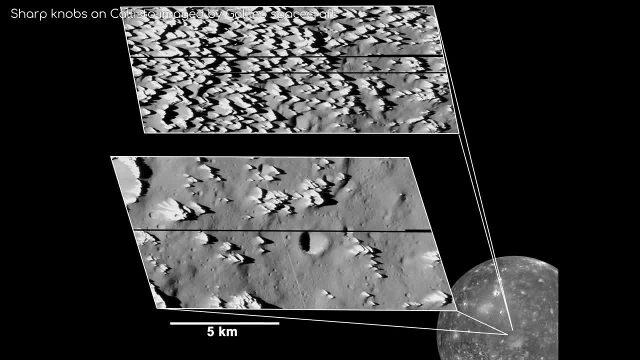 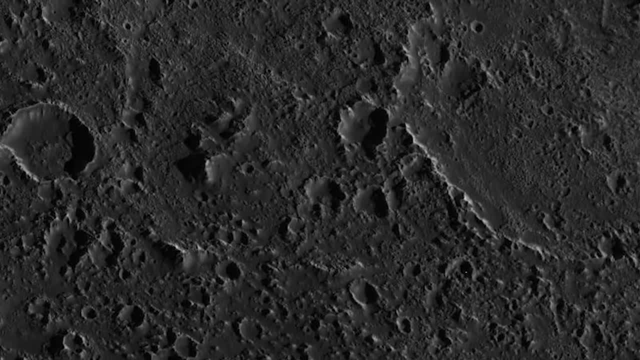 So what are the knobs? Well, they are believed to be the degraded remains of the millions of crater rims from Callisto's past. We don't know exactly why they have degraded so much over time, but perhaps it's due to micrometeor images. 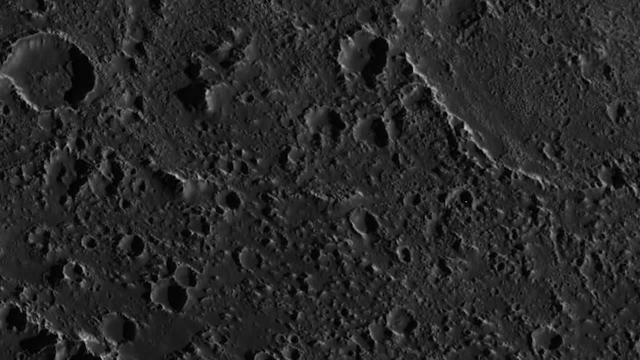 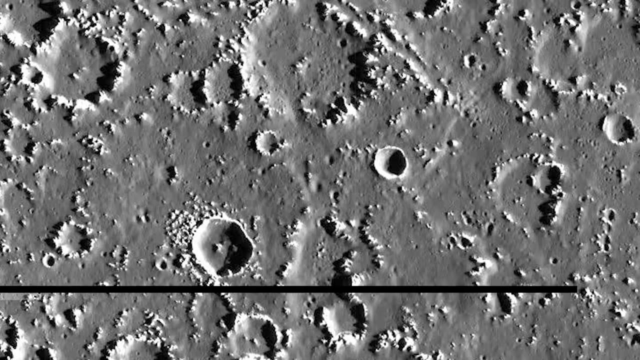 Maybe it impacts or simply the ice is slowly sublimating over time. They are brighter than the lower planes because the rocky debris from the meteors and micrometeors will have fallen down the knobs over time, leaving the pure ice exposed at the top. 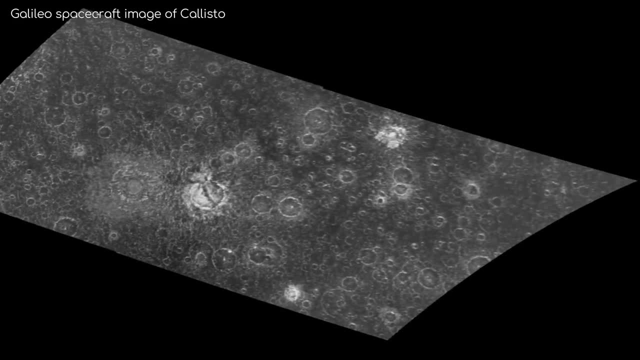 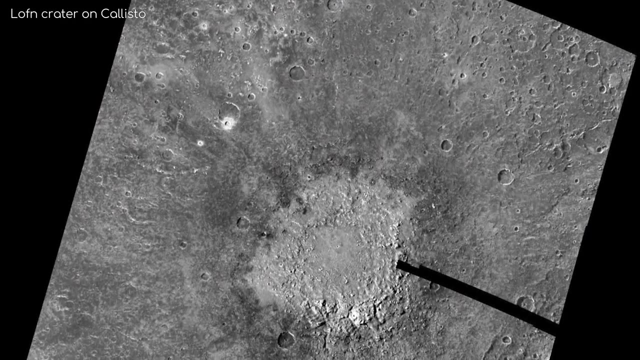 Smaller impact craters are also fascinating due to their uniqueness. Most impact craters are shallower on Callisto compared to our moon. For instance, the Luffen impact structure: It's well over 100km wide. However, it's only 600m deep. 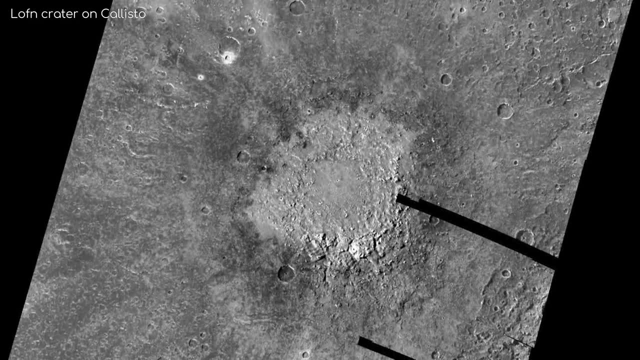 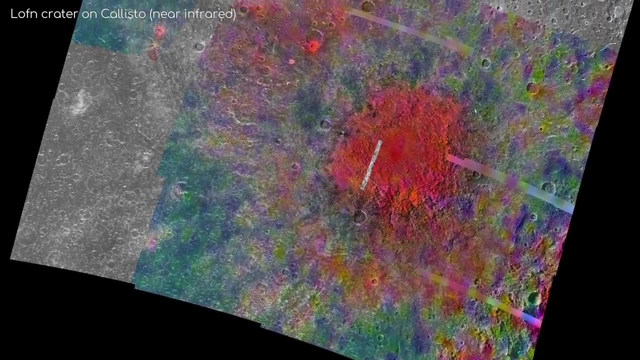 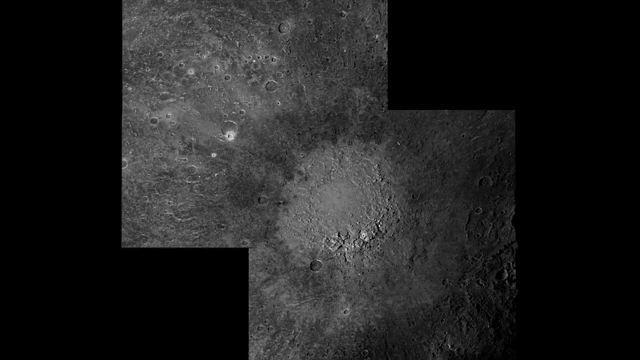 This could be because the impactor was breaking apart before it impacted, causing more of a spread-out shotgun effect on the surface. or it could be that the surface has since levelled off from other larger nearby impacts that have occurred later on. This crater is believed to be over a billion years old at least, yet you can still clearly. 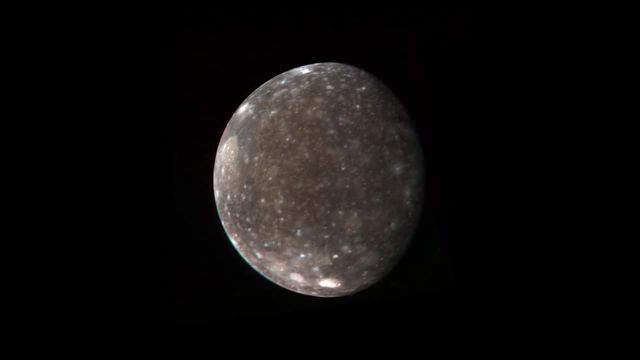 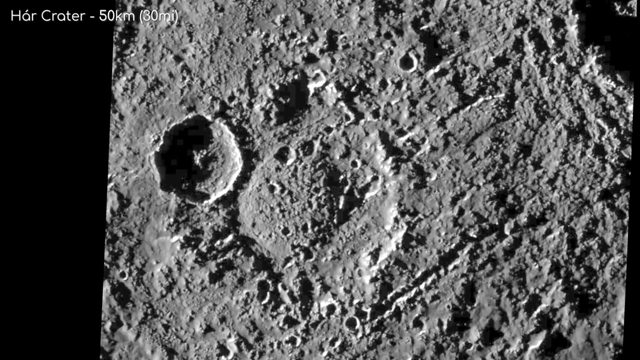 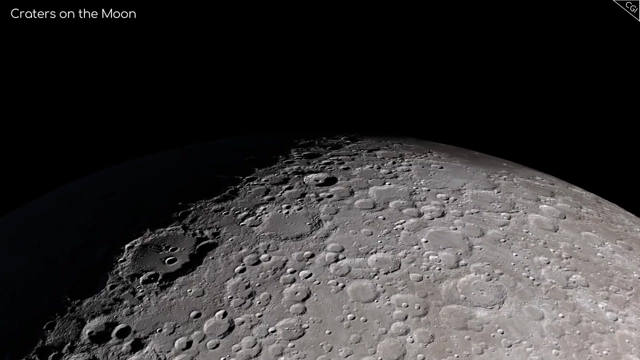 see the ejector that has streamed away from the impact- clear evidence of how unchanging this remarkable moon is. With some craters, like Haar crater, there is even a large dome found in the middle, With typical large impacts on other worlds. you will see a few concentric rings and a 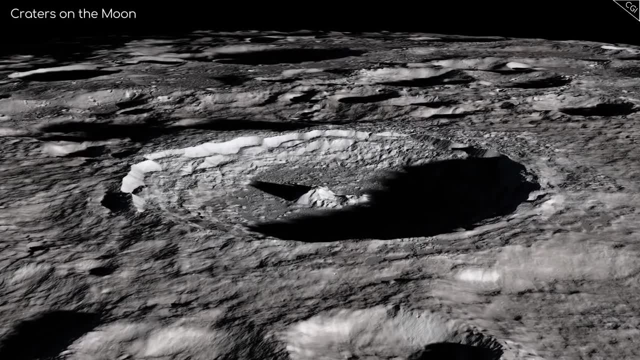 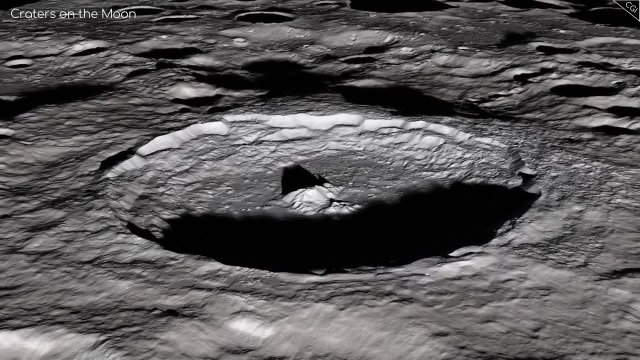 raised peak in the centre. This is very much the case on our moon. However, Callisto has some remarkable examples of large craters where just the opposite happens. Look at Tinder. here, Instead of a peak, there is actually a pit in the centre. 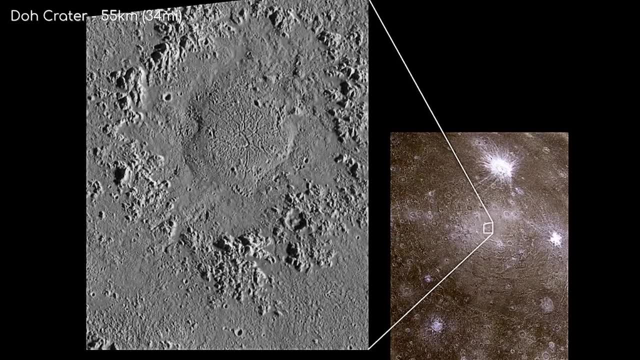 This is a very interesting example of a large crater. It's a very interesting example of a large crater. This is a very interesting example of a large crater. This is a very interesting example of a large crater. Why does Callisto have such unique craters? 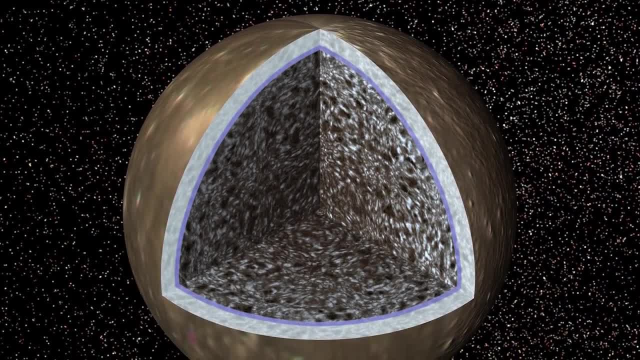 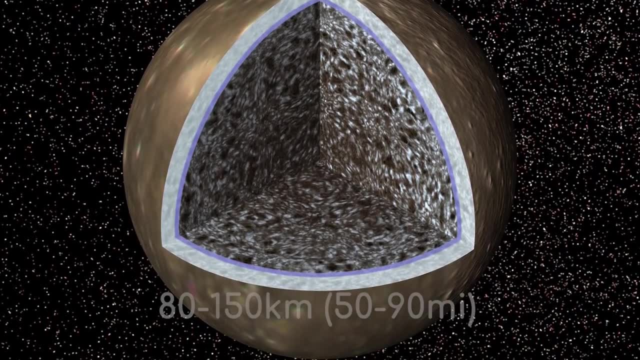 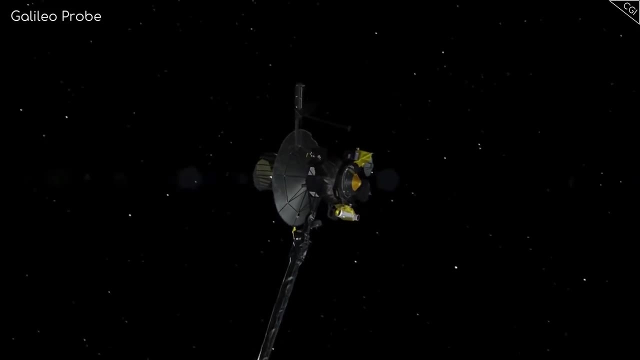 It could be due to the fact that Callisto's crust is not just brittle but pretty thin too, with either soft ice or a salty ocean underneath. Estimates put the crust at 80 to 150km thick. The Galileo space probe, which spent several years around Jupiter, spent a significant 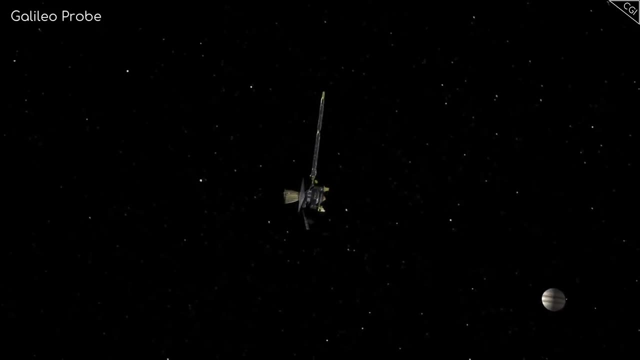 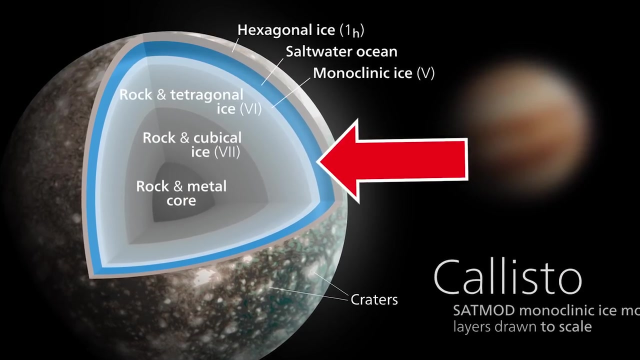 chunk of its time aptly studying the Galilean moons, Galileo found that Jupiter's magnetic field was much smaller than Jupiter's. This means that the magnetic field could not penetrate through Callisto, implying there is a highly conductive layer under the surface, at least 10km thick. 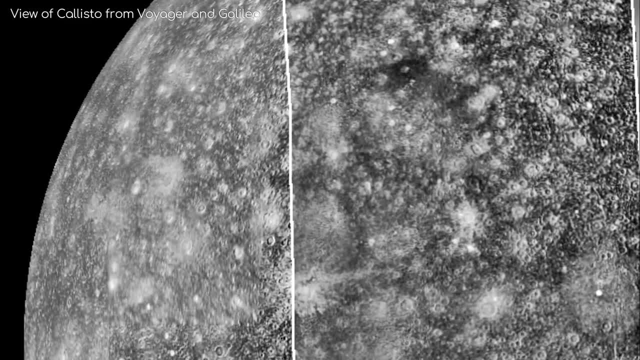 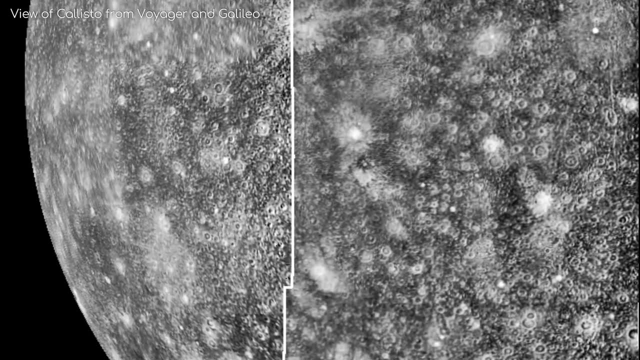 This couldn't have happened in ice or silicates. unless the ice layer is at least partially molten or very large temperature gradients can be maintained below the ice to create a conductive effect. Data also suggests that Callisto has a small silicate core at its centre, with a radius of about 600km, Which begs the question: Can Callisto be conducive to life, like other icy worlds with water mantles under their surfaces? Well, life as we know it requires liquid water and energy to exist. Callisto might have an ocean of liquid water under its surface, but being about 800 million. 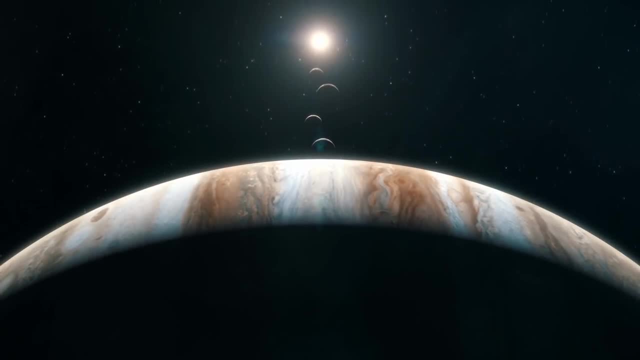 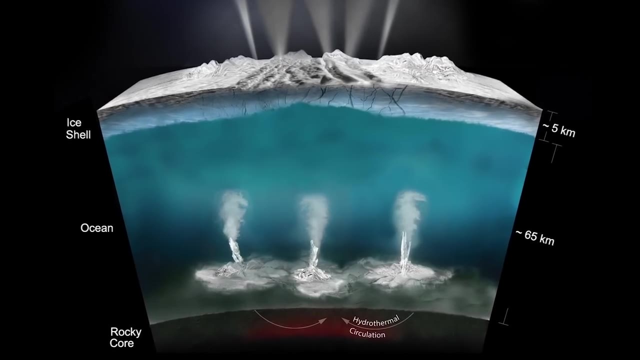 kilometres away from the Sun, it barely receives any heat from our star, And the absence of tidal forces doesn't help either, leaving radioactive elements the only source of heat to warm this subsurface ocean. The only source of heat to warm this subsurface ocean. 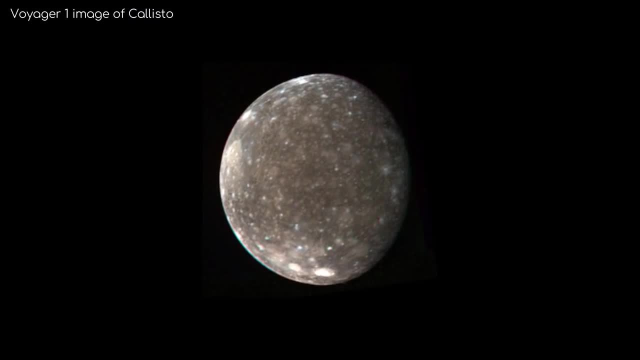 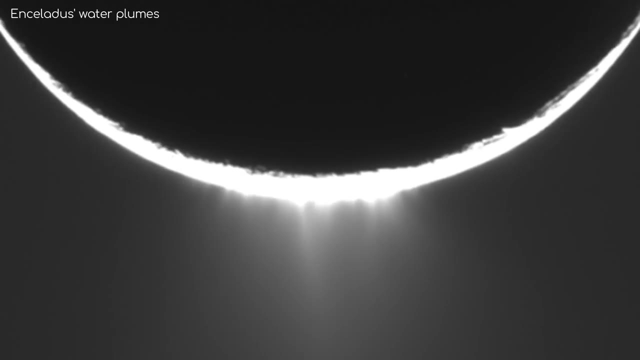 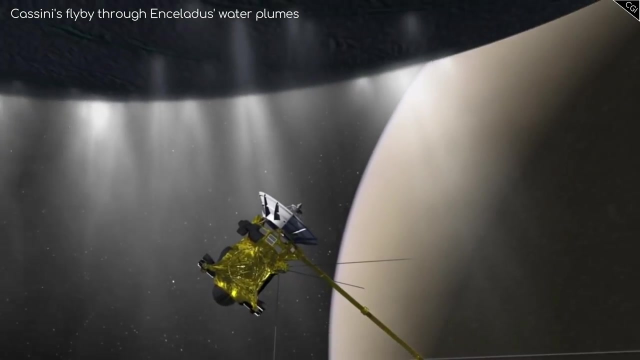 The only source of heat to warm this subsurface ocean And, unfortunately, even visiting Callisto won't prove anything. Moons like Europa and Enceladus have vents ejecting water directly from their subsurface oceans, meaning we can investigate habitability prospects without ever going into the oceans. 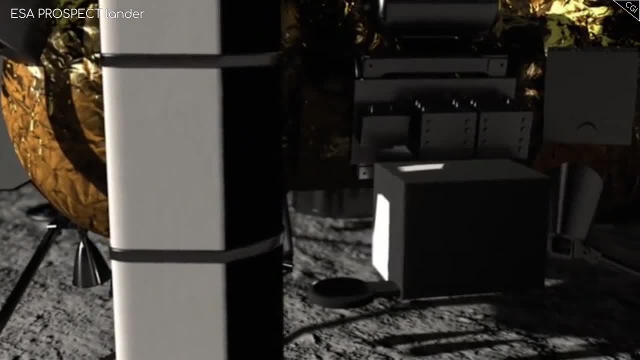 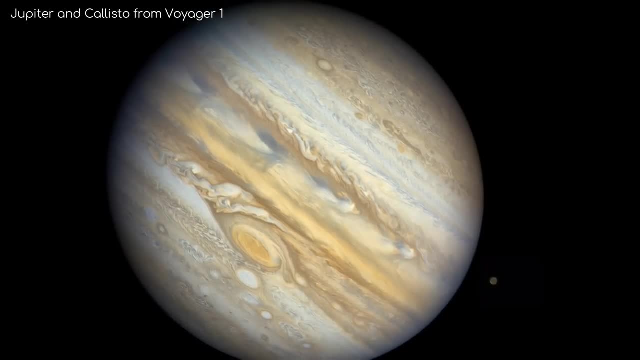 themselves. No such vents exist on Callisto, so scientists would have to penetrate the crust in order to find out. All these things combined mean that, unfortunately, scientists think that the environmental conditions necessary for life appear to be less favourable on Callisto than on any other icy worlds. 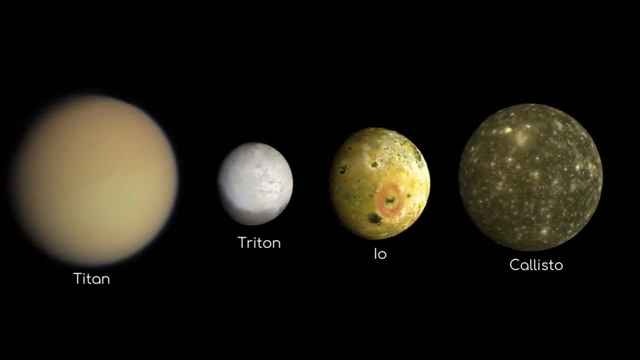 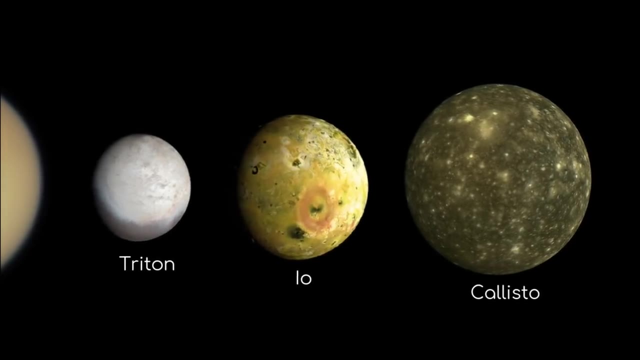 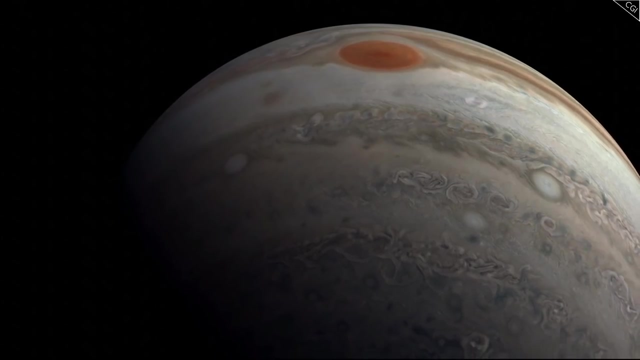 Nevertheless, Callisto shouldn't be ignored. If we ever go to explore the outer solar system, Callisto would make a perfect base. You see, orbiting at a distance of 1.9 million kilometres from Jupiter means that Callisto is located beyond Jupiter's main radiation belt, making its environment thousands of 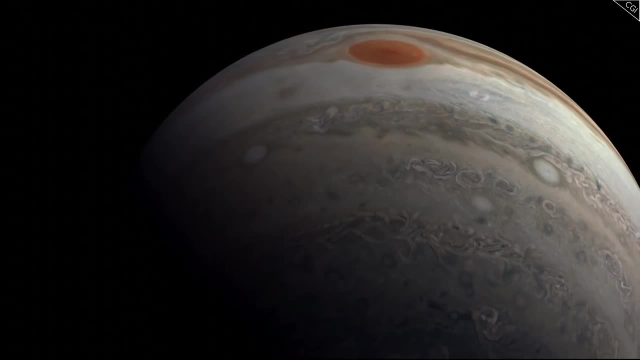 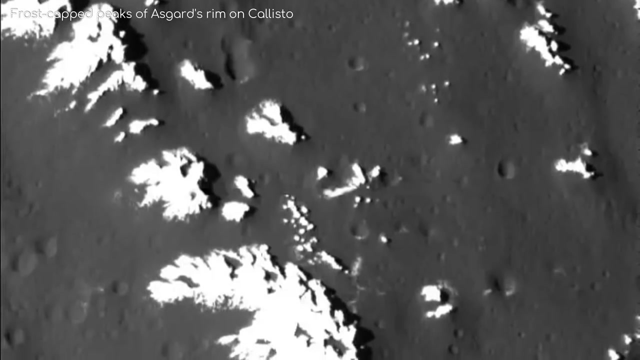 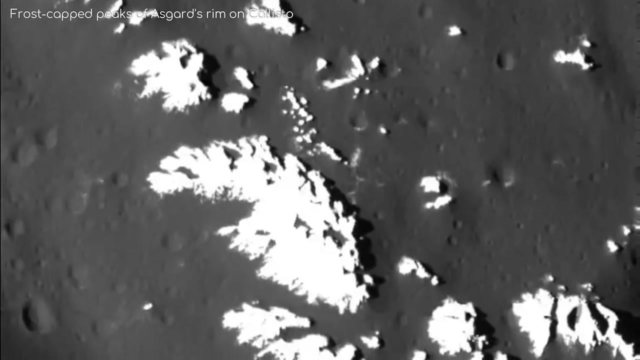 times more conducive to human exploration than its inner moons. Callisto also has a lot of water ice that can be used for propellant production and, of course, is the staple to keep humans alive. Separating the hydrogen from oxygen also leaves oxygen for breathing. 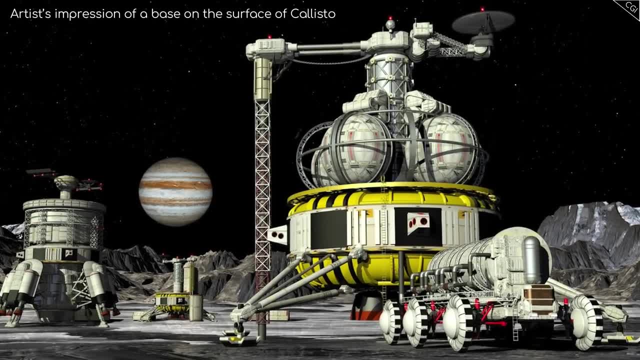 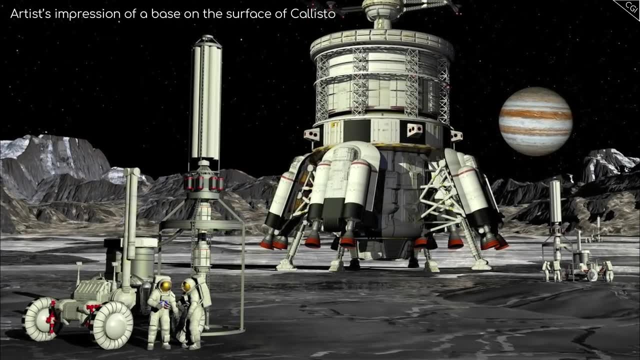 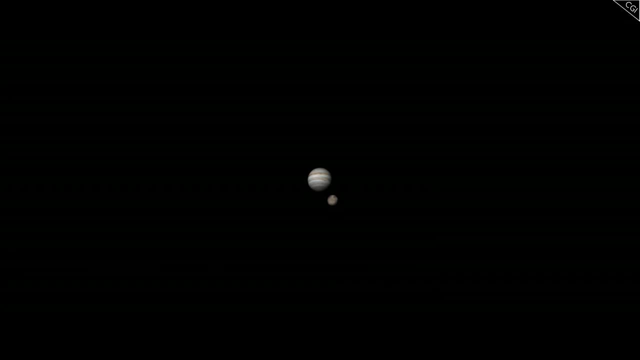 Callisto's geological stability would make for building structures on the surface relatively worry-free, and the lack of huge mountains or deep trenches means it's faster, easier and more efficient to travel over. Thanks for watching. From Callisto, we could better explore the inner Jovian system from a safe distance or 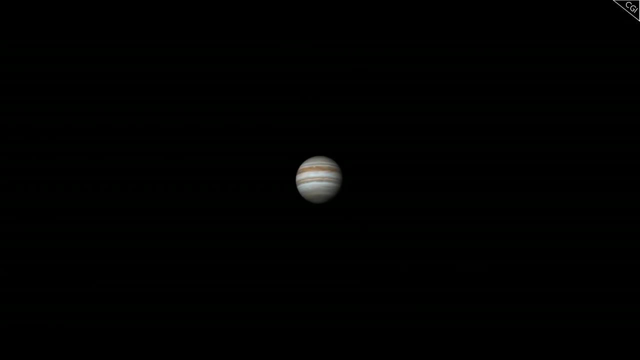 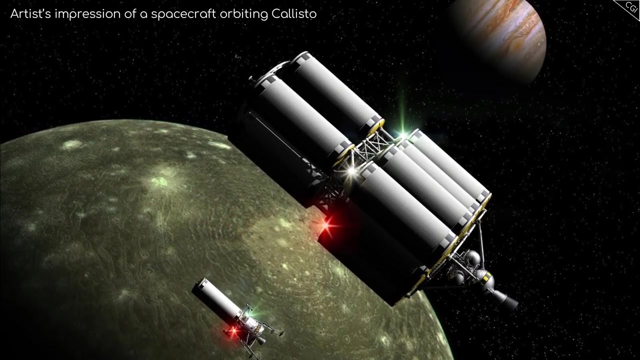 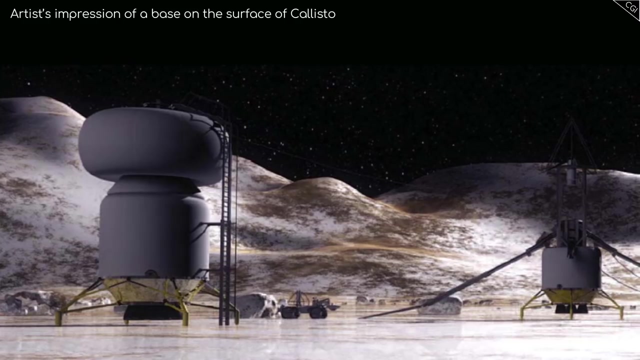 use it as a way station for heading farther into the outer solar system. Lifting off from Callisto would be ideal, thanks to its low gravity, and you could get a gravity assist from a close flyby of Jupiter. It's true that this is a futuristic prospect, although if we ever do become a space-faring. 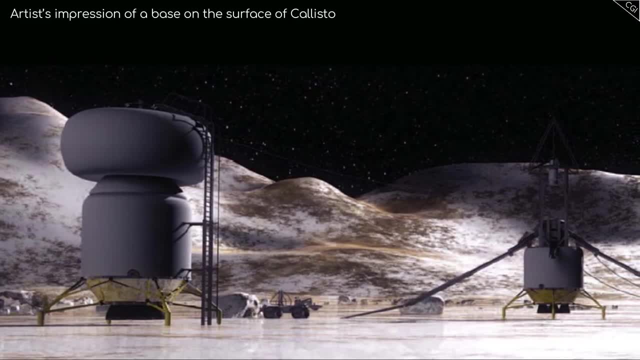 species. this is a distinct possibility. Now, while Galileo did an admiralty experiment on Jupiter, it was also possible that the space-faring system of Callisto would be able to do that. While Galileo did an admirable job studying Callisto during its few flybys, there is still. 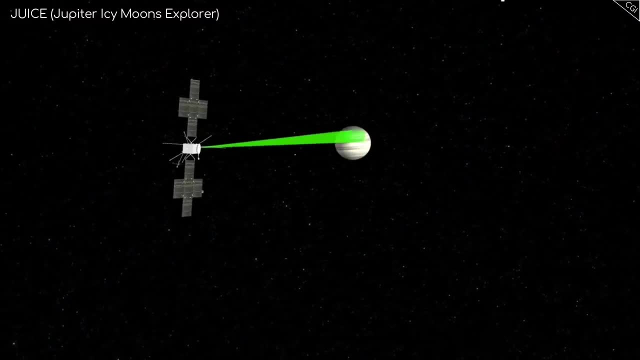 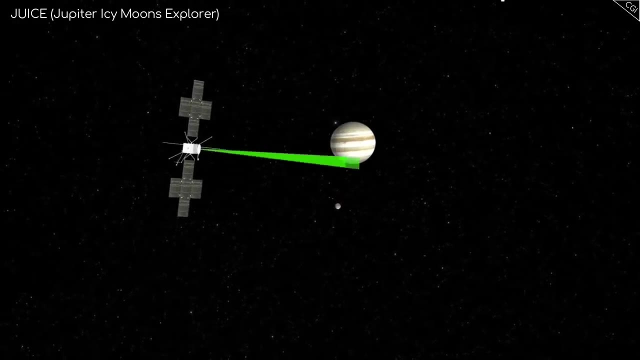 a lot of information gaps that need to be filled. With any luck, we'll get that from the European Space Agency's Jupiter Icy Moon Explorer, due to launch in 2022, which will reach the Jovian system by 2030 and will explore Jupiter. 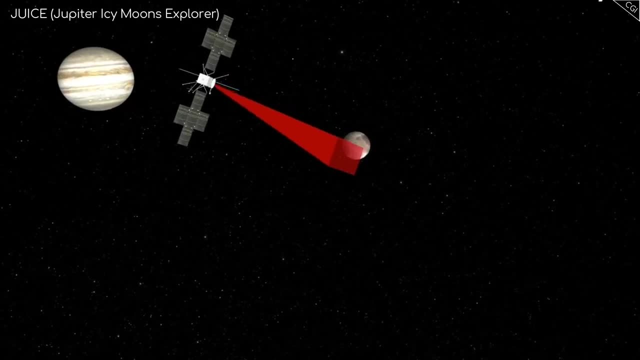 and three of its largest moons: Ganymede, Callisto and Europa. ESA has planned several close flybys of Callisto during this mission. This mission might provide more insight into how Callisto can be used as a space-faring system. 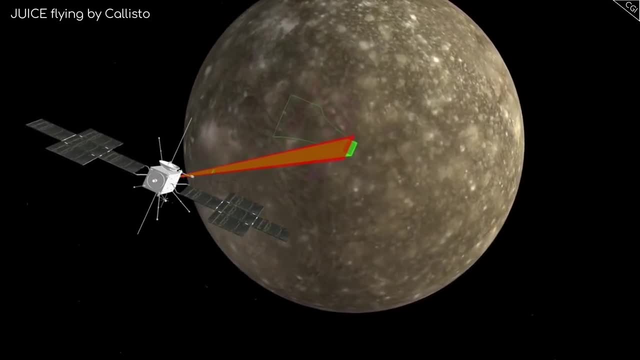 ESA has planned several close flybys of Callisto during this mission. This mission might provide more insight into how Callisto can be used as a space-faring system. ESA has planned several close flybys of Callisto during this mission. This mission might provide more insight into questions like: does it have a subsurface? 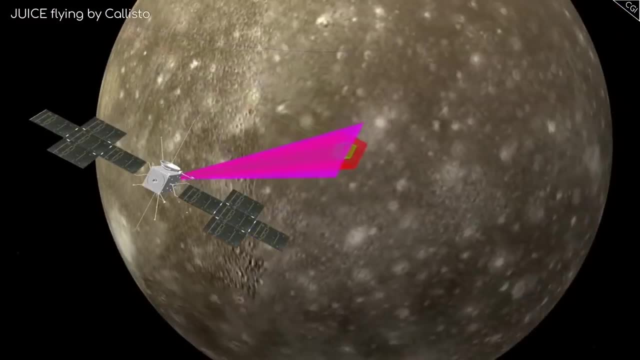 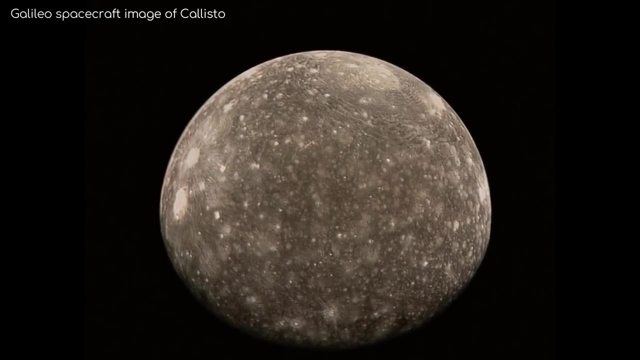 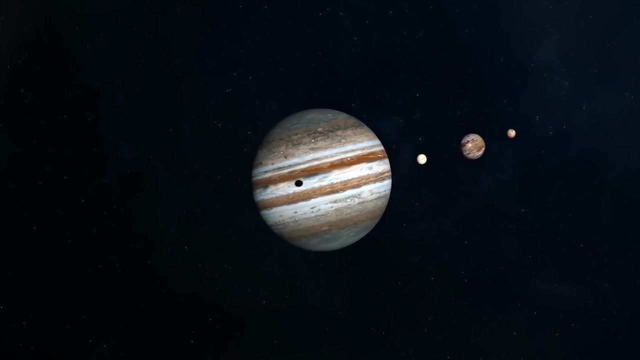 ocean and, if so, does it or can it sustain life? Beyond that, there's also the questions we haven't thought to ask yet. Who knows what more we will still discover about this incredible moon. So there we have it: almost everything you could want to know about the Galilean moons.